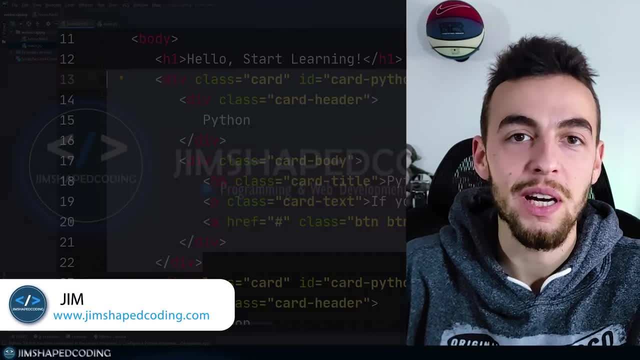 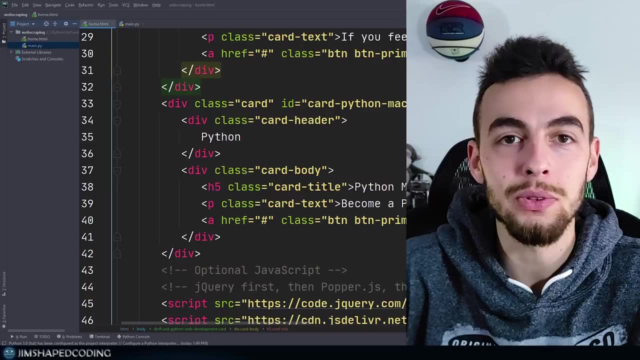 Hi everyone and welcome to a special Python tutorial where we are going to learn how to perform web scraping. So, first of all, thanks to free code camp to giving me this opportunity of being a guest on their channel, And I have a YouTube channel as well that is named Jim shape. 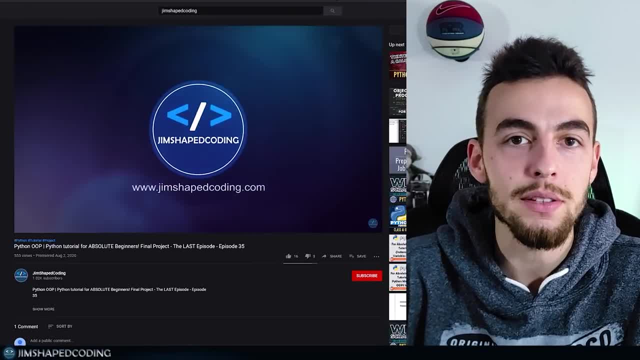 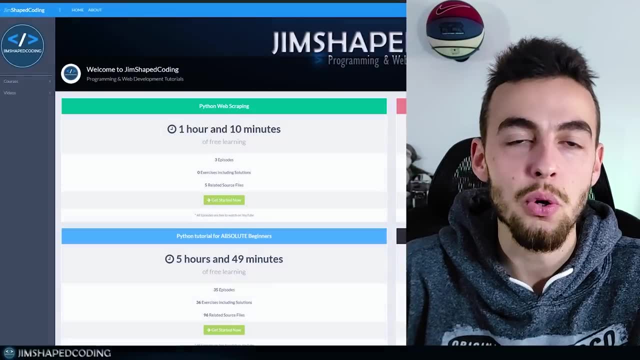 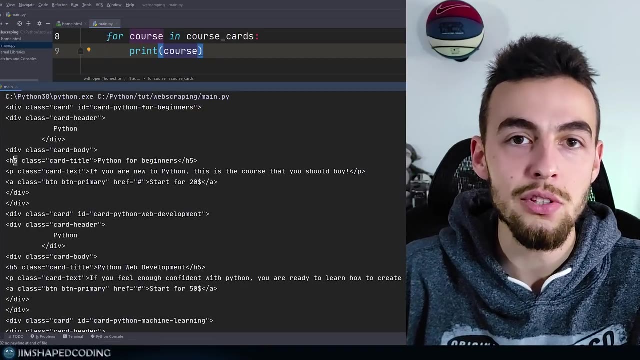 coding, And you can find there any tech related topic, such as programming language, web development and more content that I'm uploading once or twice a week, So we can just go ahead and find the link from the description. Okay, so in this video I'm going to do my best to teach you anything. 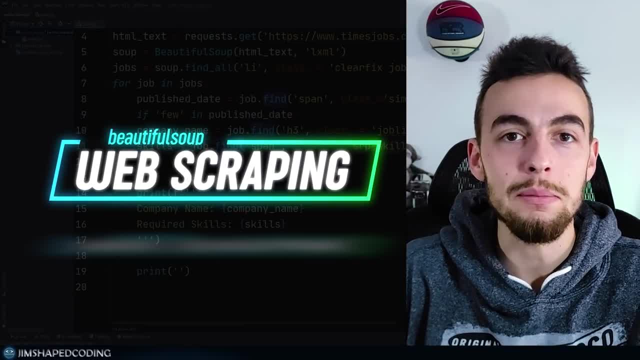 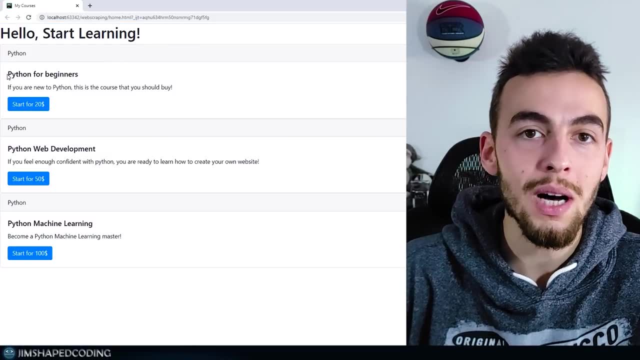 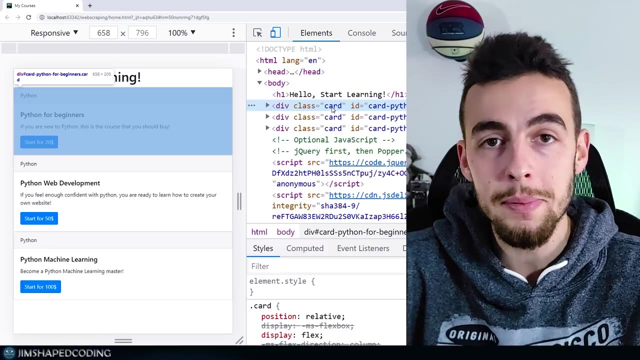 that is related to web scraping, And I'm going to do that with the beautiful soup library, And that is a special library that will allow you to gather any information you want from any website you want. Okay, so this website could be your bank account, could be a job post website like LinkedIn. 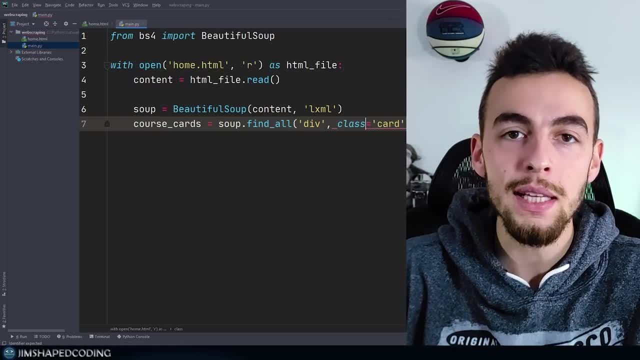 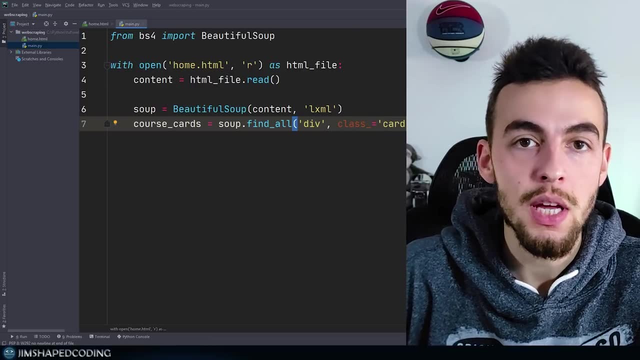 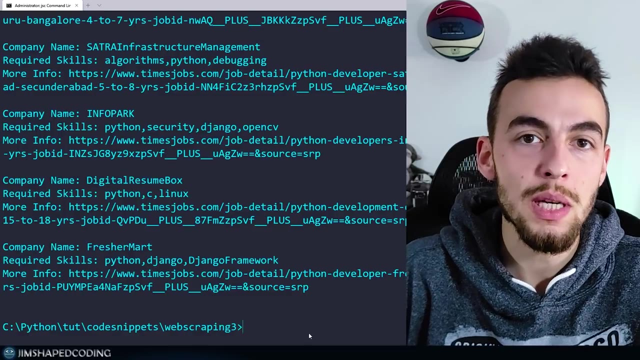 this could be Wikipedia or a sports website and really anything that you can think about. So we will start by scraping a basic HTML page first, just to understand the concepts, and then we will move on to scraping a real website. And by the last 15 to 20 minutes of this, 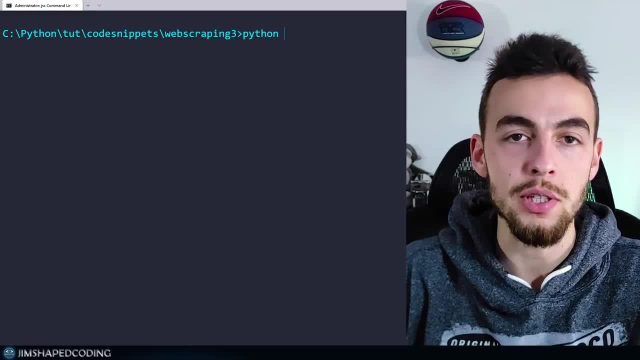 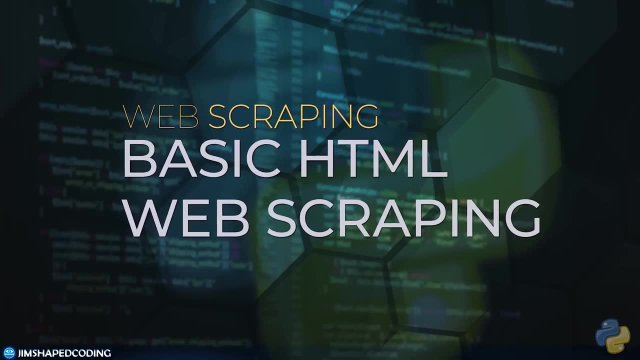 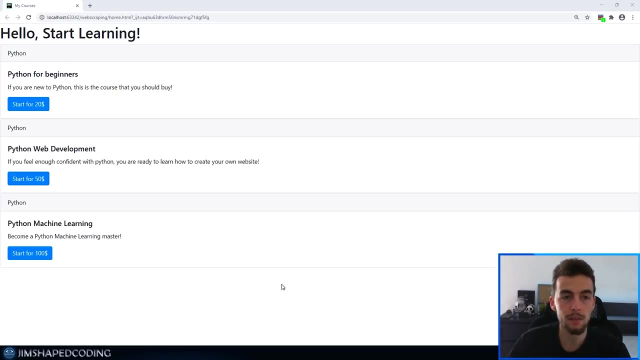 tutorial. I'm going to show you how we can store the information that we have just pulled from this website. So let's begin Right. so this is the web page that we are going to start web scraping, And I'm going to explain what is going on here, So you can see that we are having a basic title And then 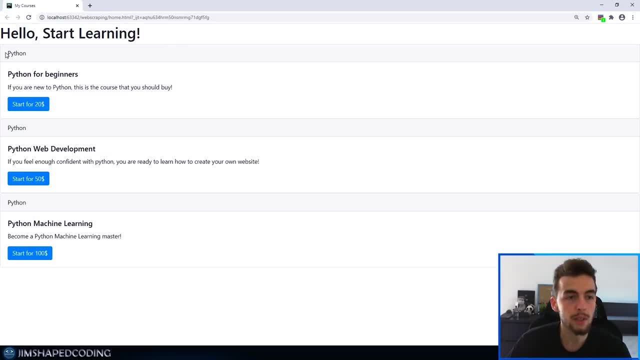 we are having a kind of three paragraphs, So you can see that we have a title of Python, And then we have a kind of secondary title, And then there is a basic explanation about the course itself, And then we are having a button that says start. that will probably lead us to a different page. 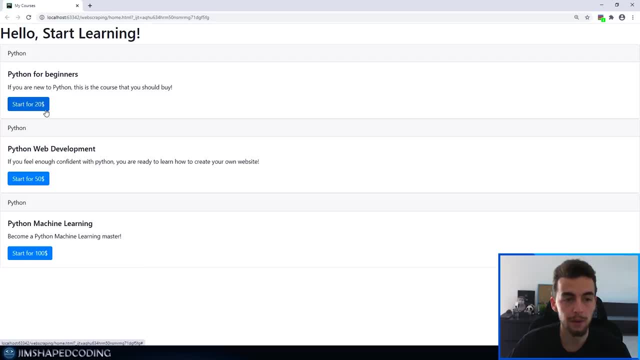 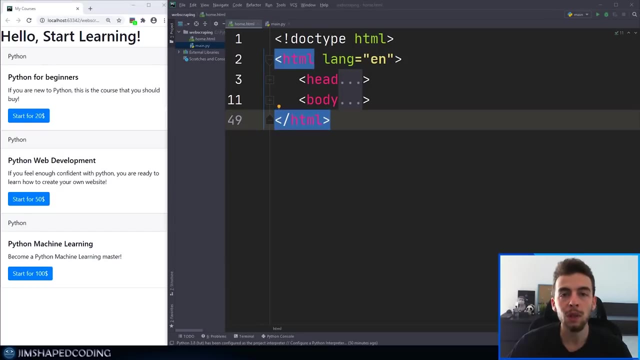 if we click on it And then you can see that it has the price here as well. Now we are kind of hitting ourselves three times here, And this is what is responsible to that web development paragraph And then also for that machine learning paragraph. Now, what we are currently looking at, 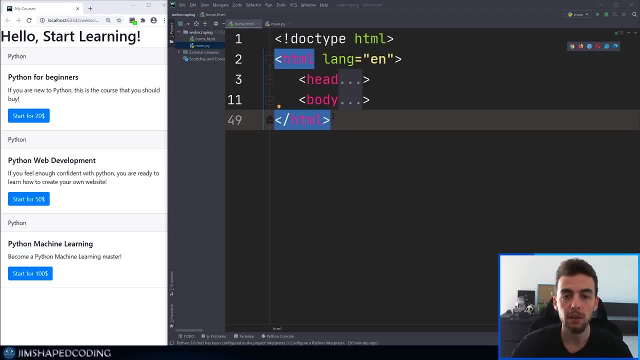 it is basically the behind the scenes of that page. So this is the HTML code that is defined in order to show you that Hello, start learning page, And you can see that inside our HTML documents, all of the code is being created with tags. 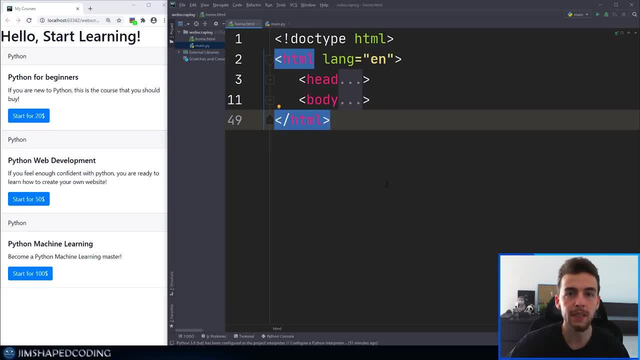 Now those tags are what are responsible to display different information for you, And you can see that we have a big tag that is called HTML And then, inside of that HTML tag, we are having a head tag and then a body tag. Now you can see that we are defining a closure. 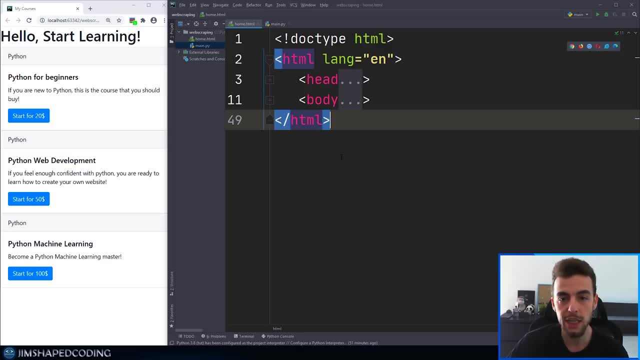 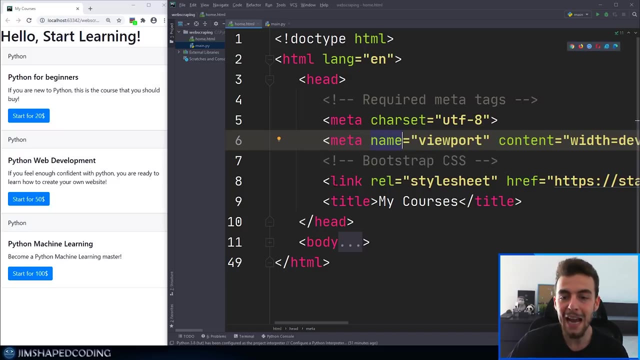 for each of our tags with the fourth slash here, And then you are probably going to see that for the different tags as well. Now let's expand the head tag here, And then inside of it we are seeing some meta information. that is not quite relevant for us, But we see that. link tag. 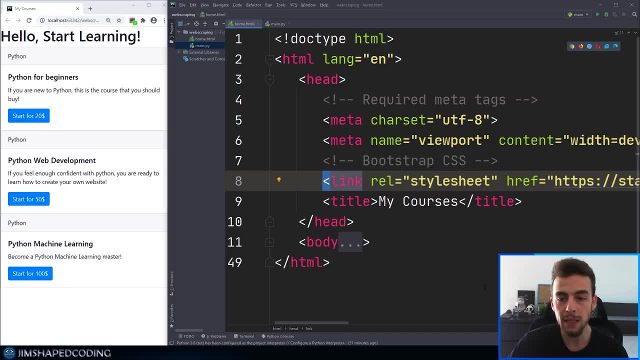 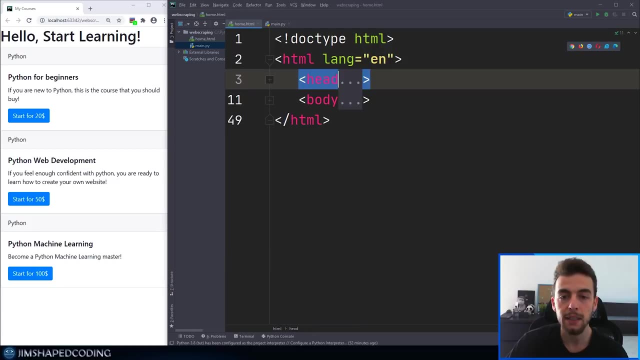 which is responsible to import some styling for our page. And then we can see that title tag, which is responsible to customize our tab name, And that is why you see my courses over here. Now I will close back the head and then I will expand the body, So the body is responsible to display. 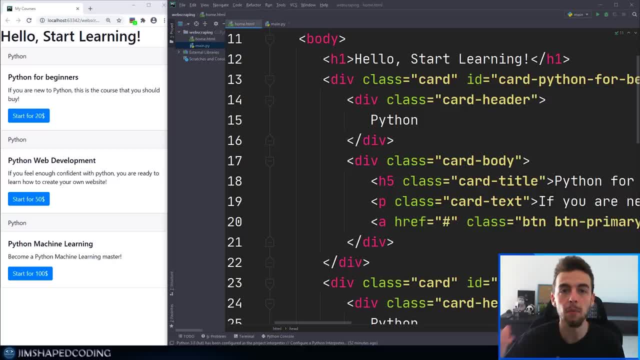 what is going to be on the page. So I will expand the head tag here And then I will expand the body, And then I will expand the page itself, which is the page's body, And you can see that we already have the h1 tag that is created here And then between the closure, which is the area that you 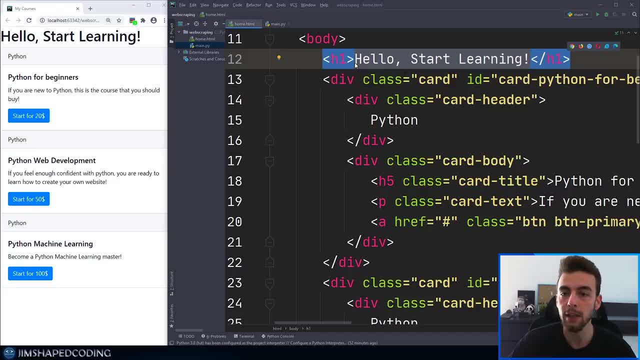 can write the text for that tag. we see the Hello comma- start learning. And then we are having some div tags here, And when you see the tag of div, this is the very basic tag that will create some tags in different styling. So you'll see here the class. 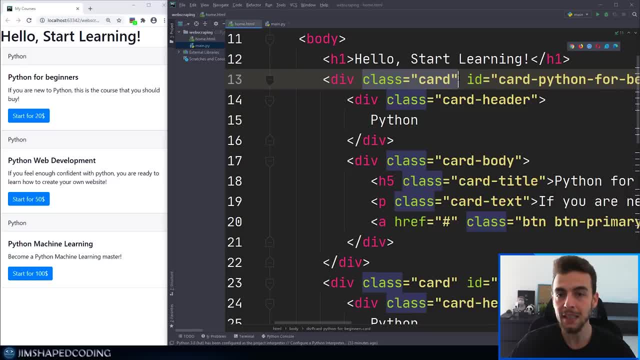 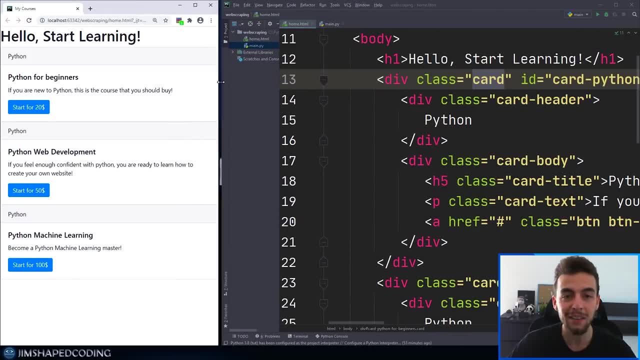 equals card. what this attribute assigning does here, it is importing the card styling And that is why you see the kind of carding style for each of our paragraphs over that page And you can see that we are having one more div inside that card class which is called card header. So this is the 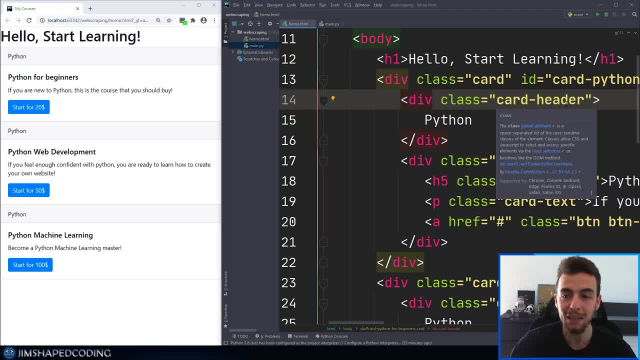 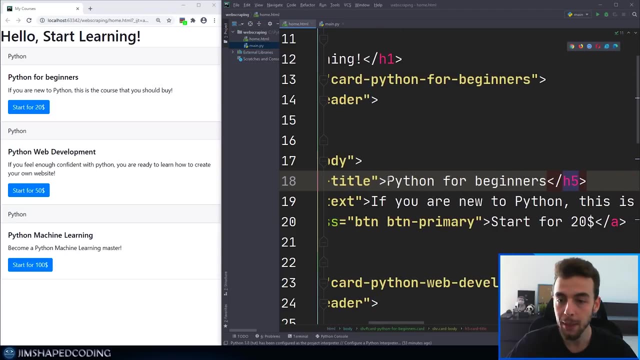 styling for card header- This is why it is called that way- And then the text is Python, And then we have the card body And we have the age five tag, which is a kind of smaller header that you can display, And if I scroll right here, you can see that Python for beginners text and then the closure. 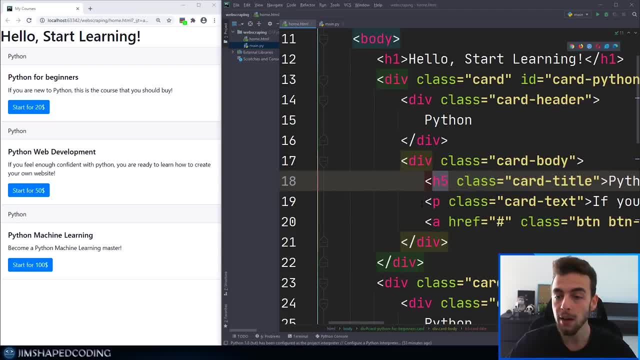 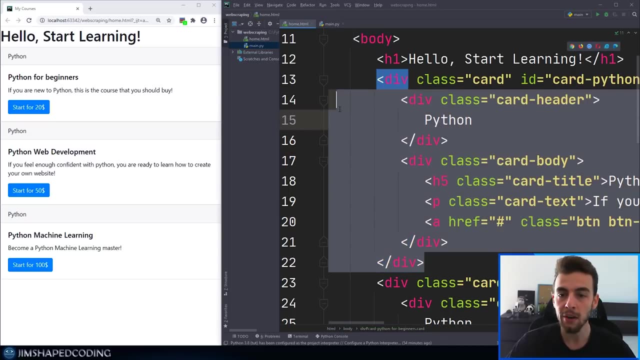 for hy age five tag, and we are having a paragraph and then the a tag which is allowing us to lead to another page. So when you see the a tag, it is basically a reference to another page that you can visit. Now this entire page is a reference to another page that you can visit Now, this entire. 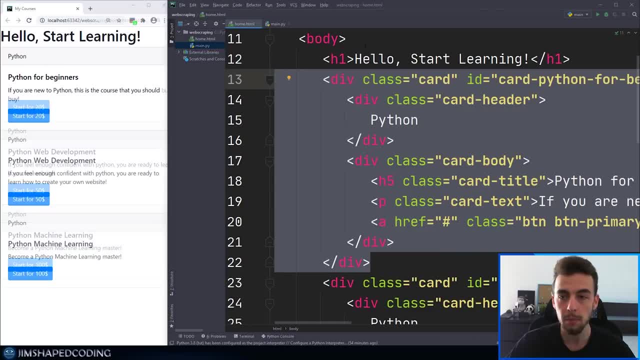 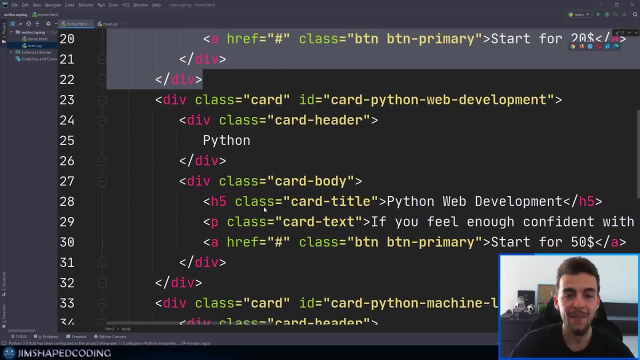 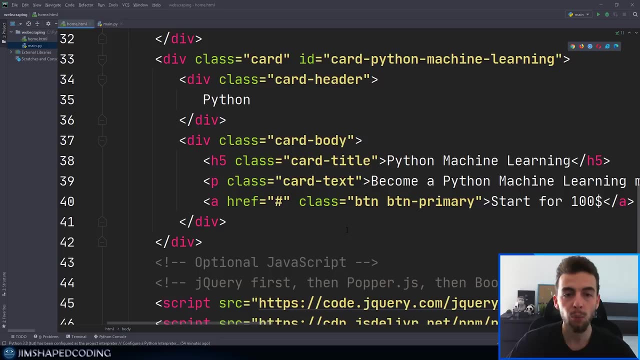 code that I'm currently marking. let's actually make our page a bigger here. This entire code that I just marked is kind of repeated three times, And that is why we see the page that we saw previously. Okay, so it is quite important to understand And we are going to scrape that page and pull some. 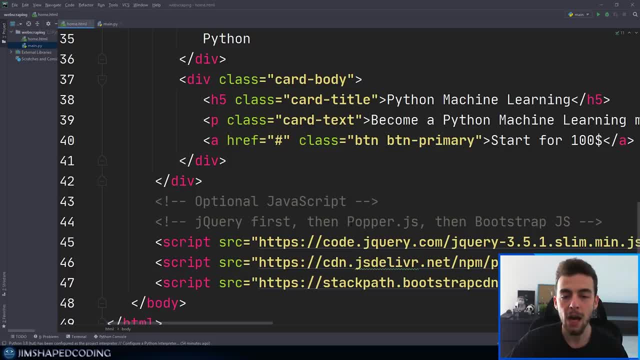 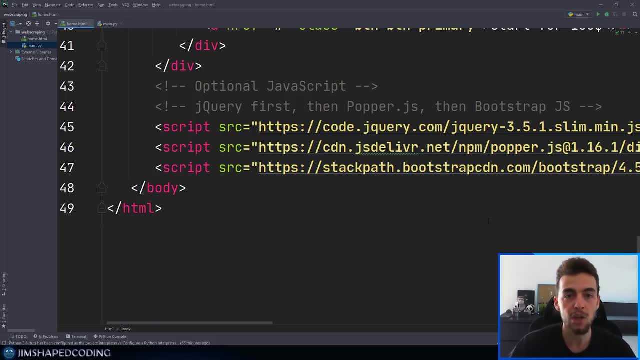 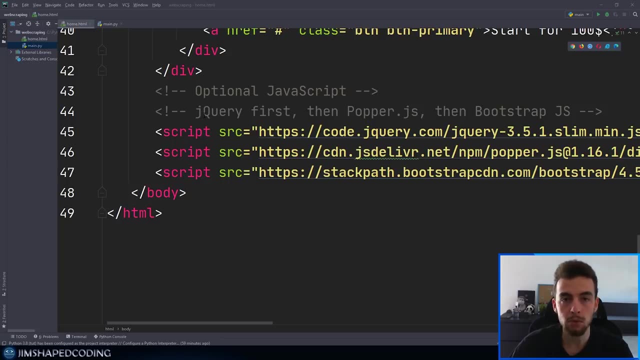 information with the beautiful soup library. Now, if you are confused with the script tags, you don't, because those tags are responsible to import some JavaScript libraries, And that is something not relevant for us right now. Okay, so we are going to switch to Python now in order to apply some basic scraping for that. 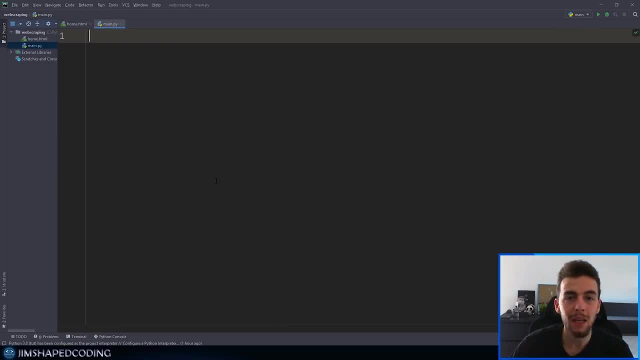 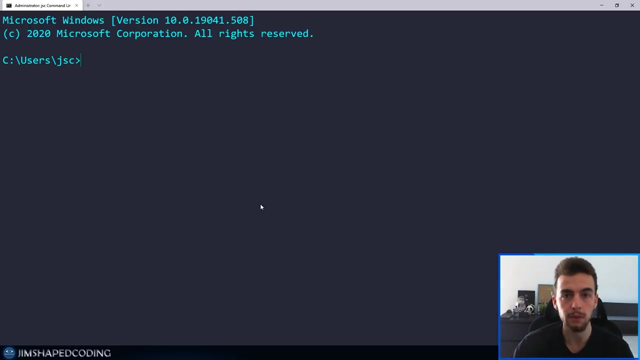 page. So I will go and start working on my mainpy file And you can see that nothing is here. Now, before we actually start, we have to install some libraries, And one of them will be the beautiful soup. So I will open my terminal And, since I'm working with my system, global interpreter. 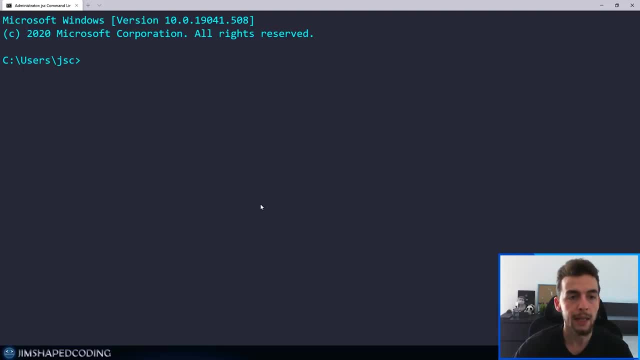 I will open my system global interpreter And since I'm working with my system global interpreter, I will allow myself to install it over here And I will go here and write pip install And then we will write here: beautiful soup for so make sure that everything is not spaced or not split it with. 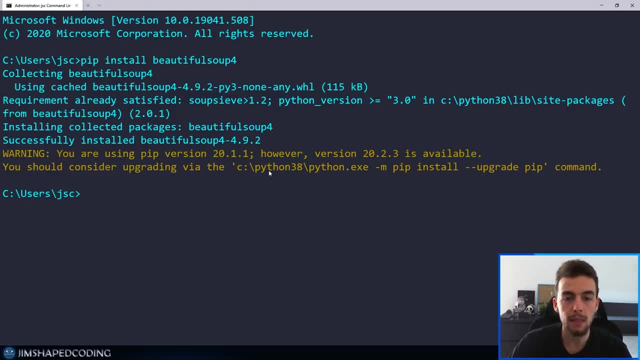 dashes, And then I'm going to hit enter, And then you can see that it is installed successfully. And then the next thing that I want to install will be something that is going to be used from the beautiful soup library, And that is the parser method. And that is the parser method, And then 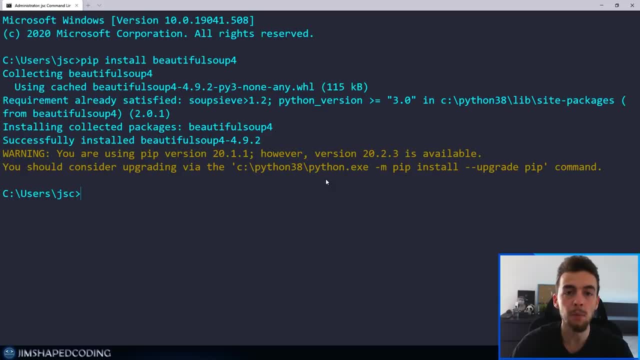 the next thing that I want to install will be something that is going to be used from the beautiful soup library, And that is the parser method. So when you work with beautiful soup, you have to specify the method that you are going to parse HTML files into Python objects. Okay, 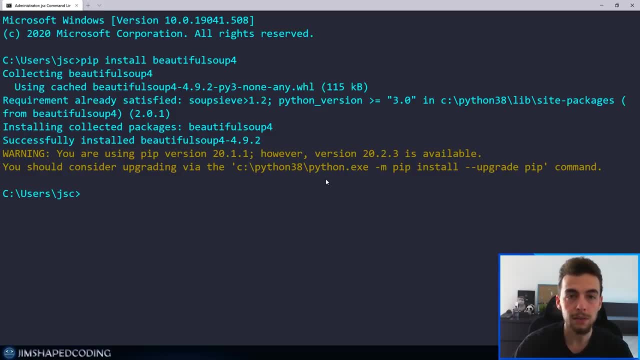 so there are going to be different methods to parse your HTML code, And I heard that the best of them could be the lxml parser, Since if you work with the default HTML parser, it is not going to deal well with broken HTML code. So just go ahead and install the lxml parser library. 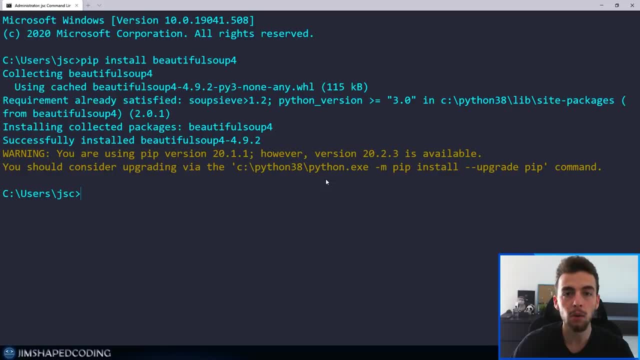 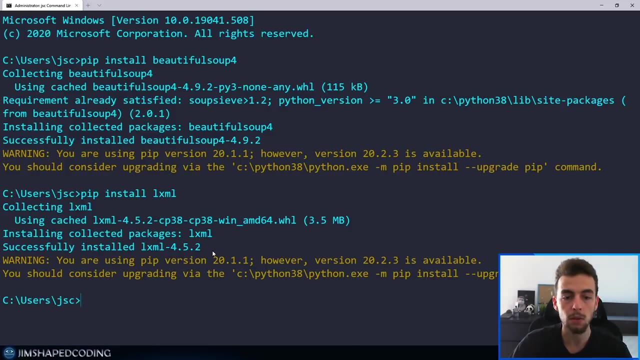 And you can also do that with pip install, And then we are going to use that when we work with the beautiful soup. So I will go here and then write pip install lxml And then, once I do that, let's wait until it's finished. Great, So we are ready now to go back to Python and start working. 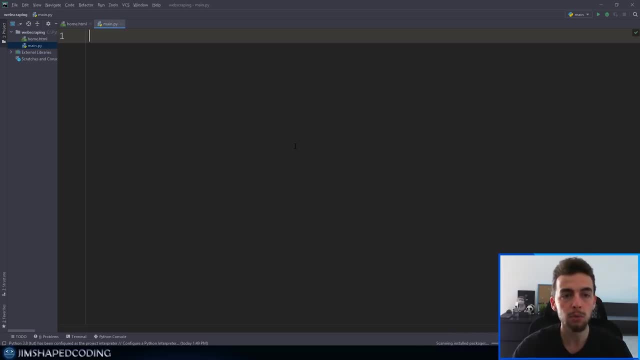 with the beautiful soup library. Now we have to go here and import that beautiful soup library. So it is a little bit confusing because the libraries folder is created as bs4. So that is why we are going to write here: from bs4, import beautiful soup like this. And once I have done that, 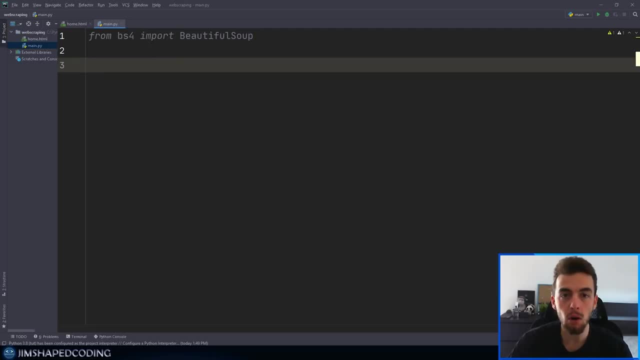 I have to figure out how I'm going to access the content inside the home dot html file that is right there inside my web scraping directory. So, in order to do that, we are going to need to create a new directory. So, in order to do that, we are going to need to. 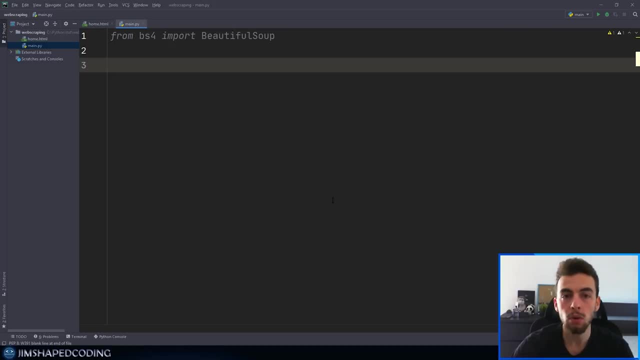 create a new directory. So, in order to do that, we are going to need to create a new directory, So we have to work with file objects. Now, if you don't know how to work with files in Python, that is totally fine, because we are going to go over it And it also might be worth to check. 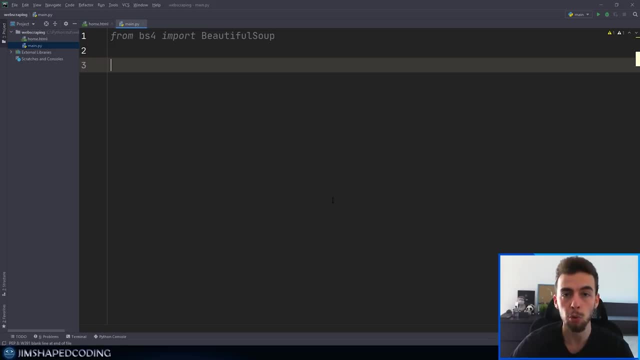 my channel out if I have already uploaded how to work with files in Python, So I'm going to write here with open. So this is basically a statement that will allow me to open a file and then read the content of that specific file. So 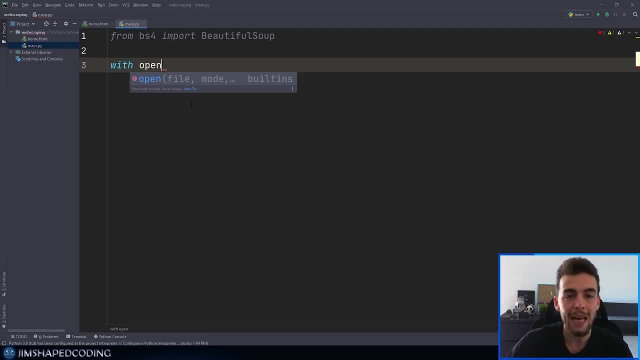 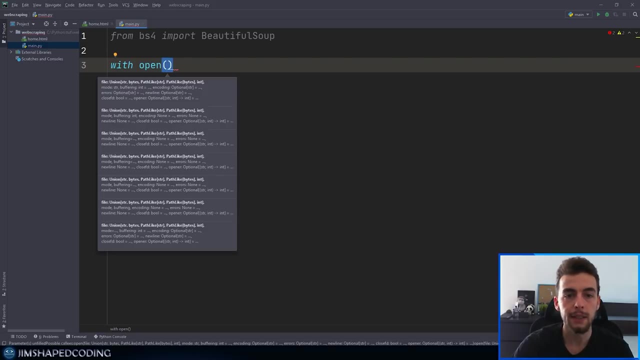 as you can see from the auto completion, I have to specify as my first argument the files name. So I'm going to close the parentheses here And then inside here I'm going to write my HTML files name. Now, since the Python file and then the home dot HTML file are in the same exact directory, 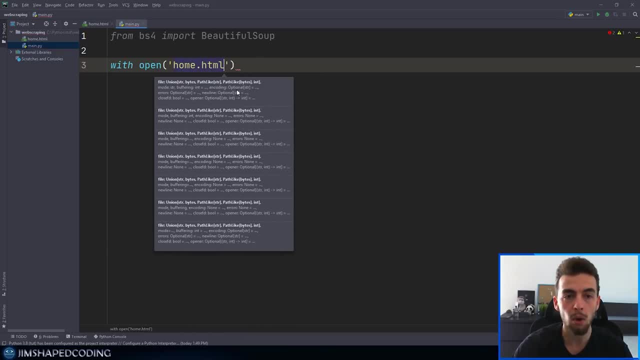 it will be okay just to write its name, So it will be home dot HTML And the second argument will be the methodhtml, And then the second argument will be the methodhtml, And then the second argument will be the method that you want to apply when you open that file in that Python's memory. So you 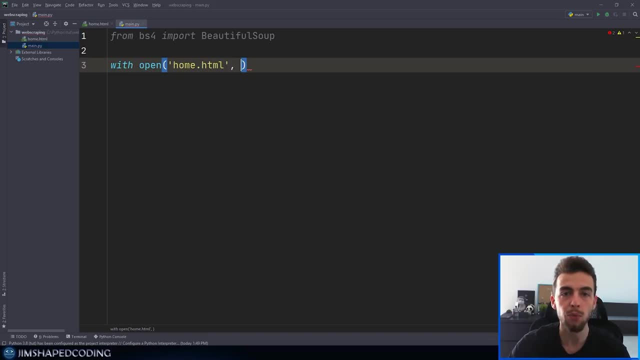 have a couple of options when you work with Python files. you can read them, you can write them or you can do both. And if we only want to read the content, then we somehow want to specify that we only want to read this file. So we will open here a new string And we will write here: are so. 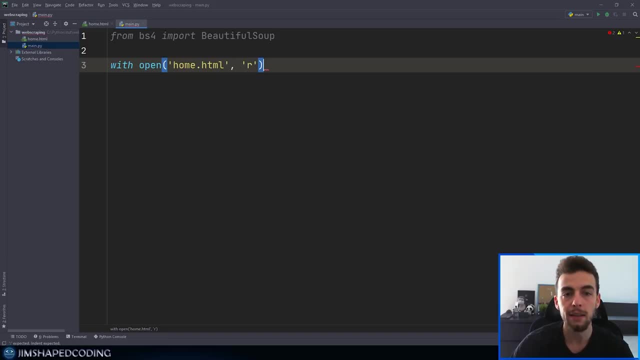 what this tells to Python is basically the method that you want to apply when you open that file. And then the third one is basically that I'm going to read that file only, And once I have done that, I have to write here a variable that is going to be used inside that code block that I just created. 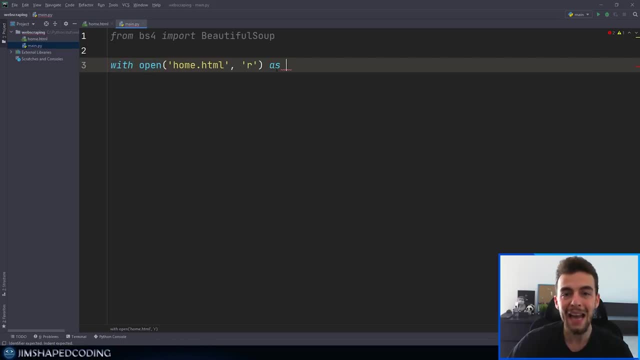 which is the width open. So I'm going to use the as keyword And then I'm going to create here a variable name that is going to be used throughout the block of the open. So it will be HTML, underscore file, And that will be basically my variable. 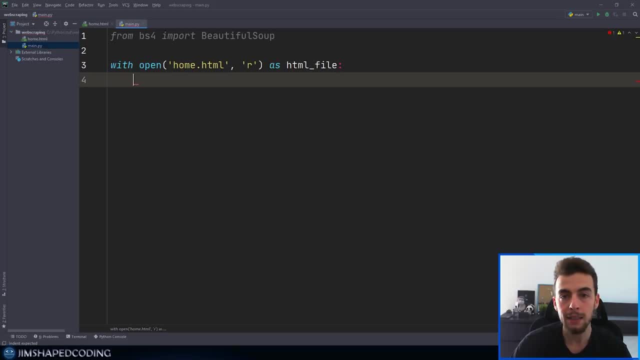 name And then, once I do that, I will go inside the open block And then I will write here: content equals to HTML file dot read. And once I apply the read method, I'm basically reading the HTML file content. And in order to show you how this works, let's first print the 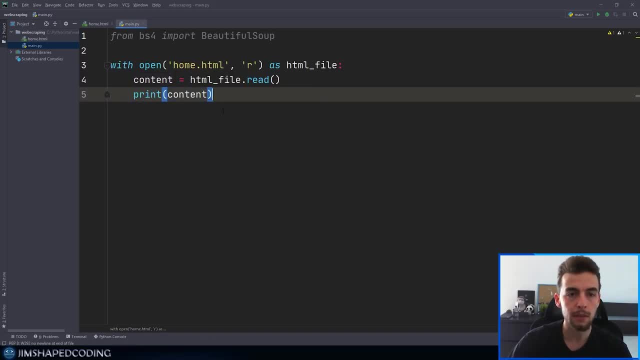 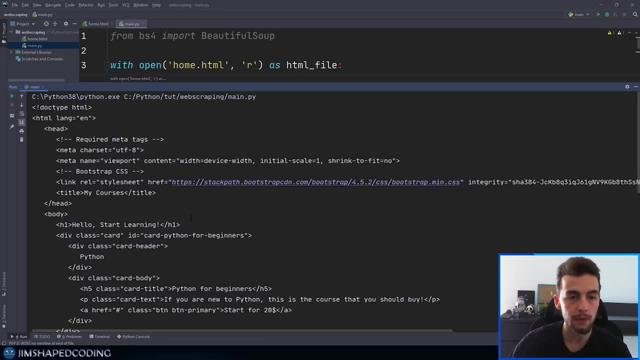 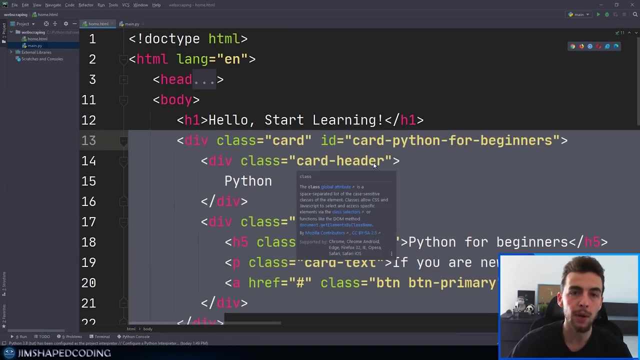 content itself. So I will go here and print the content And then I will run out the file And then you can see that the information that is printed is exactly what we saw in the home dot HTML. Okay, so we kind of did a great job reading this file Now in my future episodes. 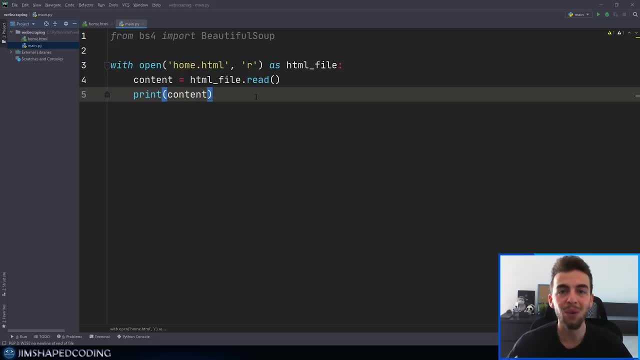 we are going to read HTML files from real websites, But I just want to give you an idea of how web scraping works in a very basic way, Because when you work with actual websites, the scraping and the information pulling is going to be quite harder than the HTML file that I just have written. 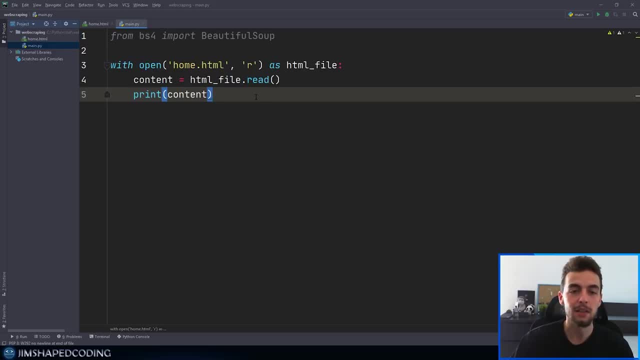 in order to explain the idea of web scraping. Okay, so I'm going to continue on here And I'm going to use the beautiful soup library in order to prettify my HTML and work with its tags like Python objects. So the way you can accomplish that will be by creating an instance of beautiful. 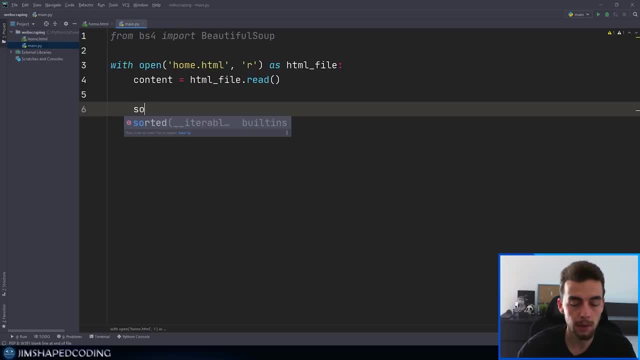 soup, And I will go here and create a new variable- let's call it soup- And that is going to be equal to a new instance of the beautiful soup library. Now, the arguments that I'm going to specify here will be the HTML file that I want to scrape, So the content of that will be: 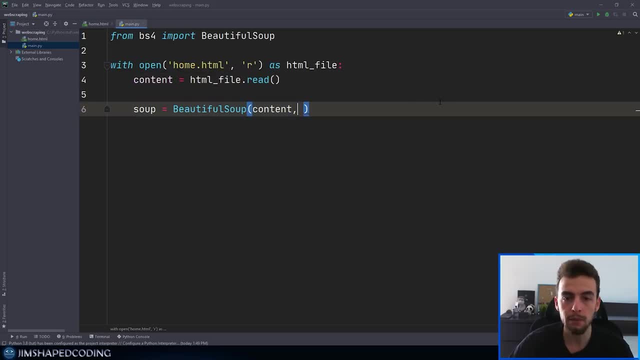 the content variable that is created up above, And then the second argument will be the parser method that we want to use. So we will pass the parser method as string, And that will be the L XML that we have just installed previously. Now, once I go, 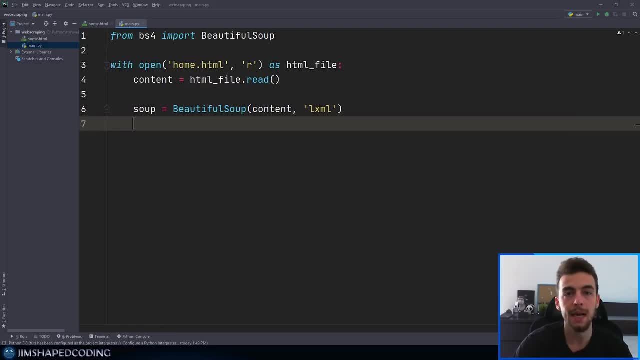 ahead and try to print what is inside that soup instance. it will be something like the following: So we will create here a print statement And then we will go with soup dot prettify. So that will allow you to see the HTML code in a more pretty way. And if I go ahead and 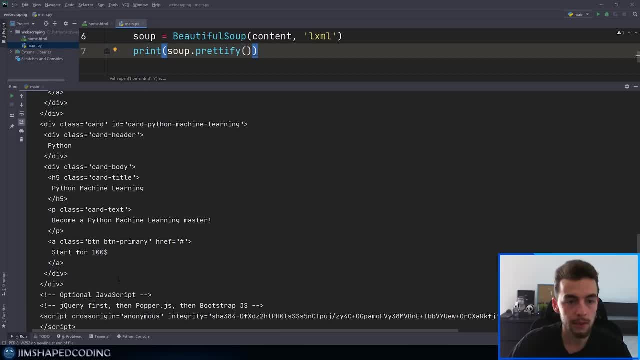 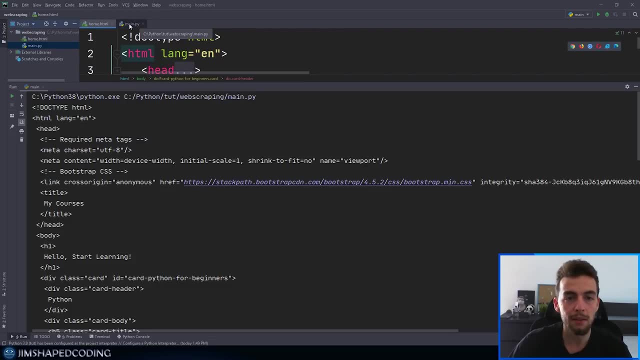 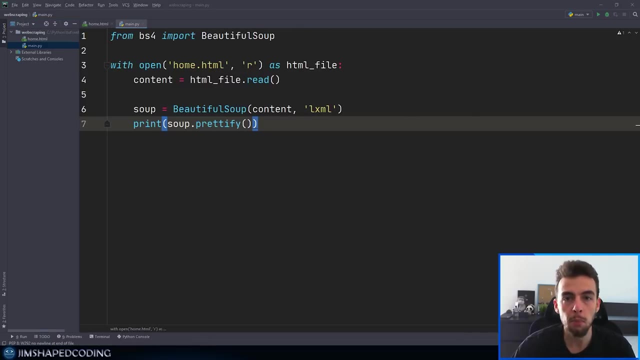 run this, you can see that we see the HTML content that is exactly the same like what we saw in the home dot HTML. So we have done a great job until now. So let's minimize back our terminal And now we are going to get more familiar with the special methods that are created inside the beautiful soup. 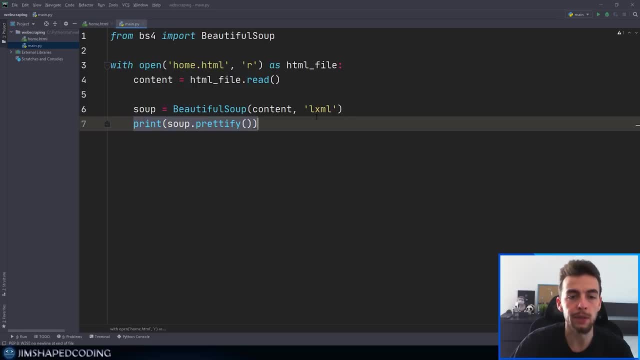 library. So we are going to delete the print from here And we are going to start working how we can grab some specific information that we want to grab. So let's assume that we want to grab all the HTML tags that are created as h5 tags. 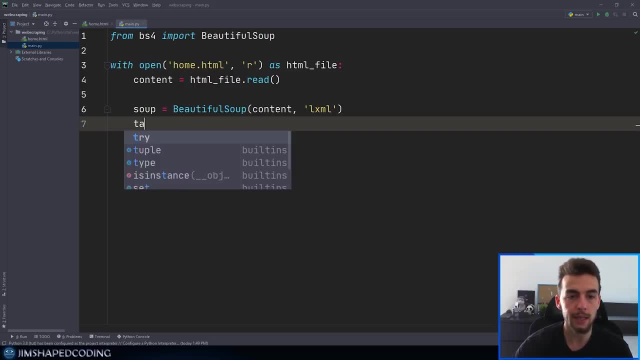 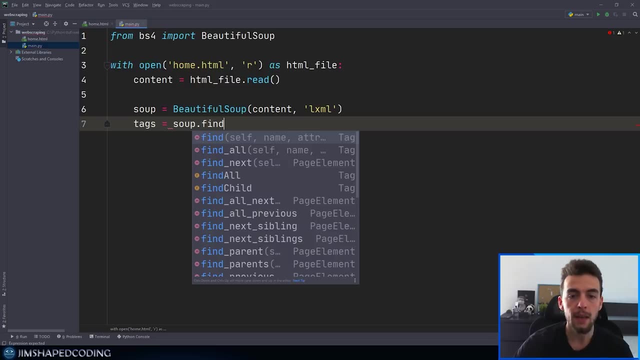 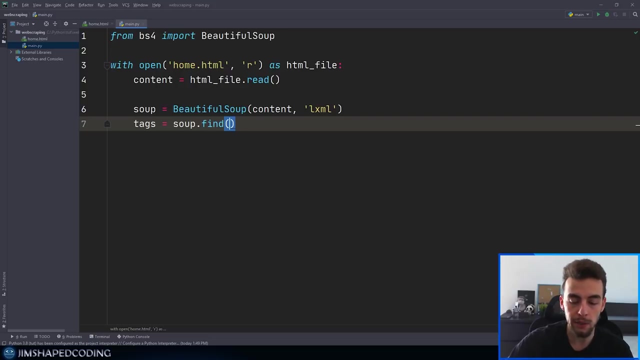 which is a kind of header tag. So we will go here and create a new variable- Let's call it tags- for example, And then we will go with soup dot, fine. And then once I go with fine, it is going to search for the specific HTML tag that I'm going to specify here as a string. So if I go here and 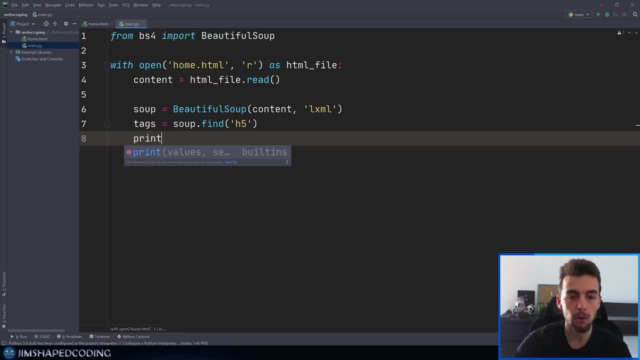 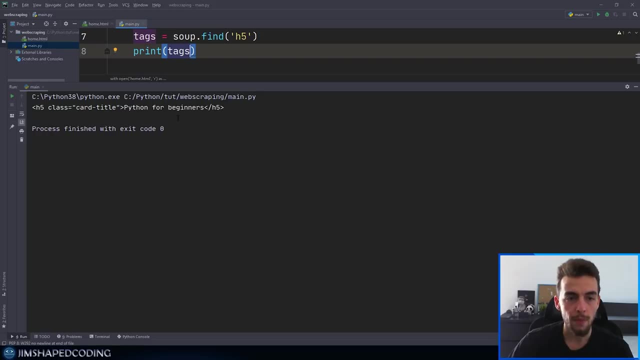 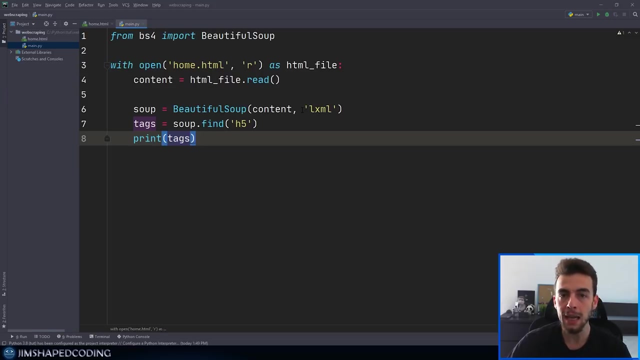 write h5, and then, down below, I go ahead and print the tags. the results of that will be something like the following: Now you can see that we have the entire HTML tag for the h5 tag, as you can see that its text is Python for beginners, But, if you remember, we have more than one h5 tags that are: 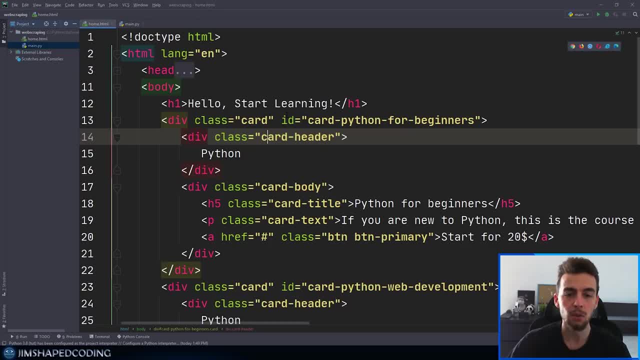 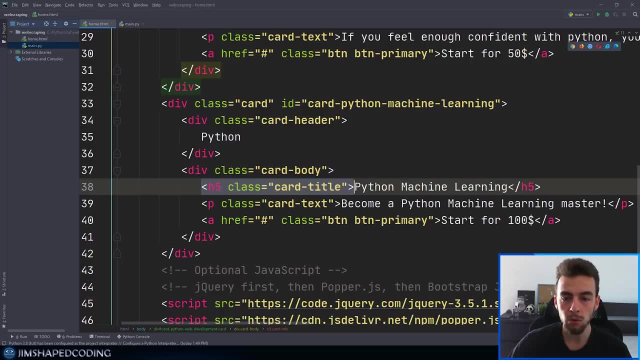 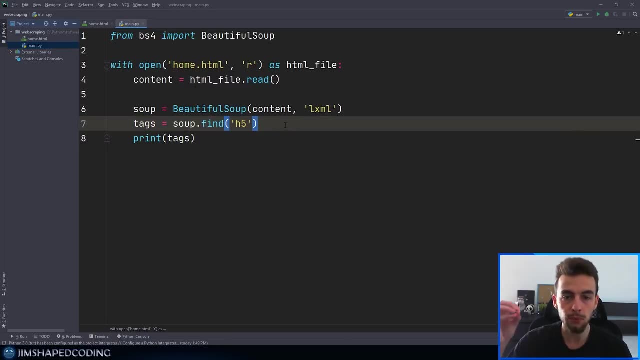 created inside our home HTML tag. So if you remember from the home file, there is a little bit of a difference between the first one here, there is the second one over there and there is the third one over there. And what that means? it means that the find method searches for the first. 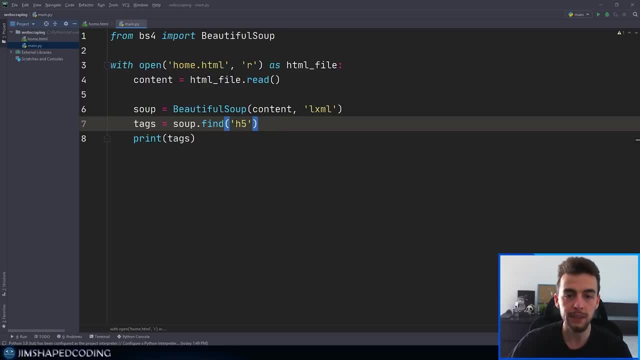 element and then it stops the execution of searching for the HTML tag that you are looking for. Now. if you want to change this behavior and not only grab the first element, then basically you have to change your method into find underscore. all okay, 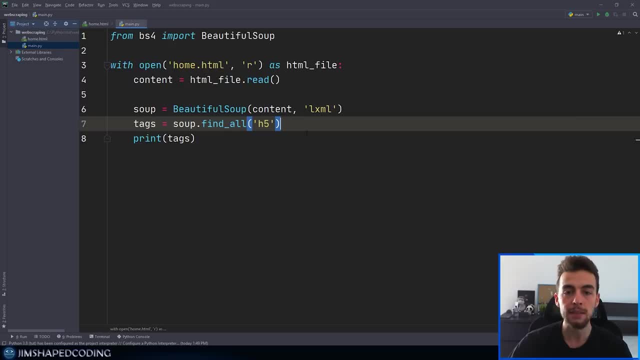 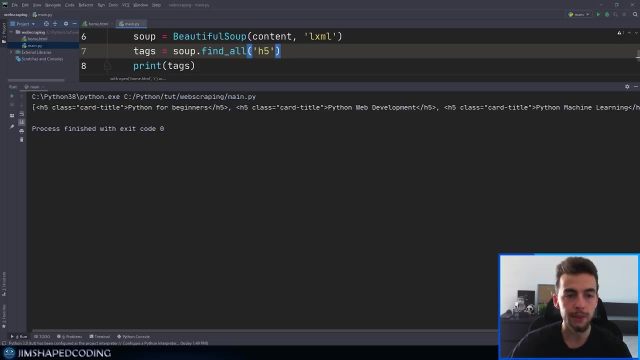 we'll search for all the h5 tags inside the content, And now, if I go ahead and run that out, then you can see that the result here is quite different, as we have here a list And then you can see that it has Python for beginners, and then also Python web development and then also the 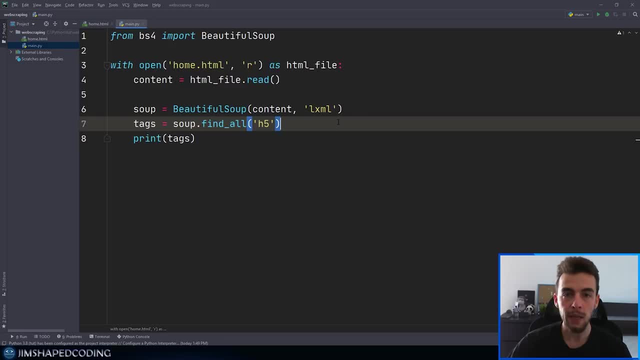 Python machine learning. Now, that will be a great logic to bring you back all the courses names from that web page, So you can go here and change this into courses HTML tags. Okay, so this is what the h5 tags are actually responsible for, And now I can write here some different code that will allow me to. 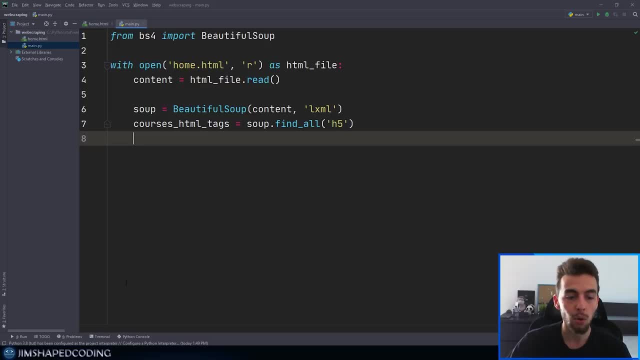 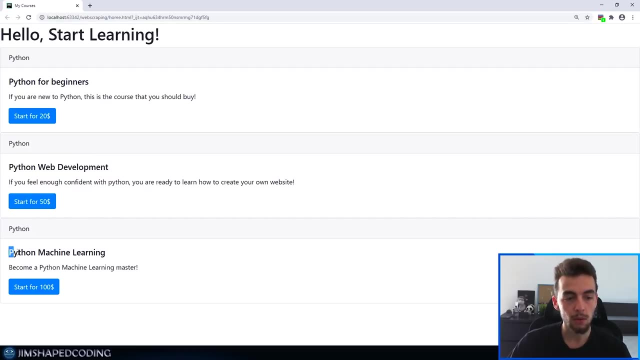 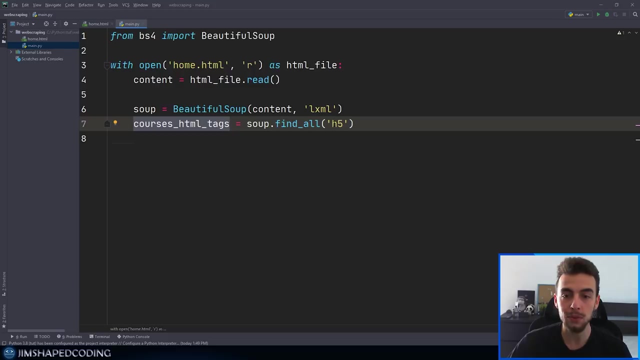 see all the courses that are defined on our page. So we have Python for beginners, and then we have Python web development, And then we also have Python machine learning. So we can work with these courses. HTML tags- that stores all the h5 HTML tags and write a nice program that. 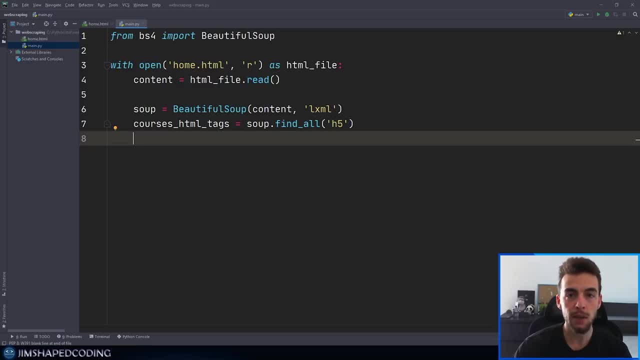 is going to display all the courses. So we can actually create here an iteration over the courses HTML tags because it has a list. So we will go here with four codes in courses HTML tags And then inside of that course tag that we are iterating we can bring only the text attribute. 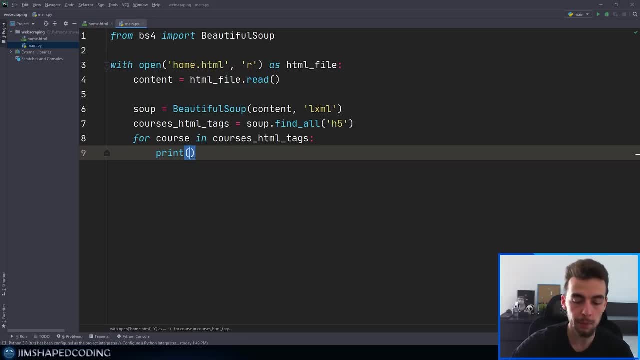 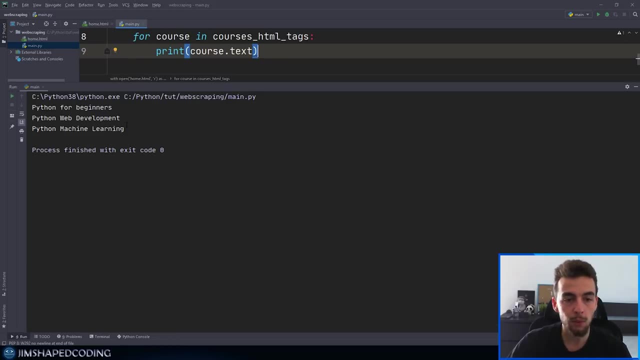 which is going to display the course text itself. So it will be here, course dot text. And now, if I go ahead and run our program, then you can see that we have a nice output regarding all of the courses that are available from that page. So this could be a nice starter to understand how you can scrape. 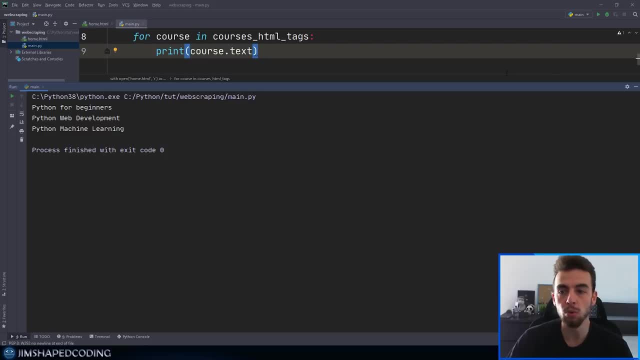 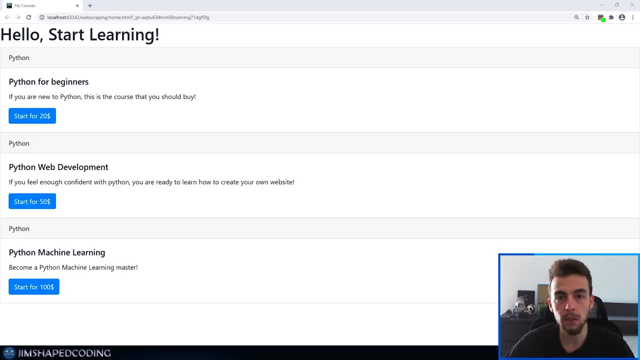 a web page to grab some specific information you want. Alright, so we were able to understand how we can apply some basic scraping to a web page, But when you are going to deal with real websites, the HTML code is not going to be quite friendly. 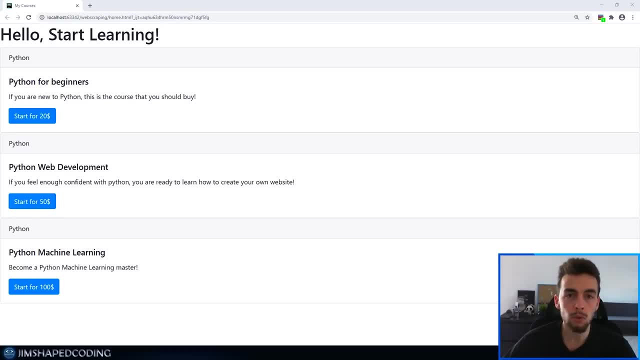 and simple like we had here. So in order to be able to access the HTML code behind the scenes of some page, we have to use the inspect of any browser. So let's say that you want to grab the price for each of the courses, So it makes sense to go with your mouse and hover to that button. 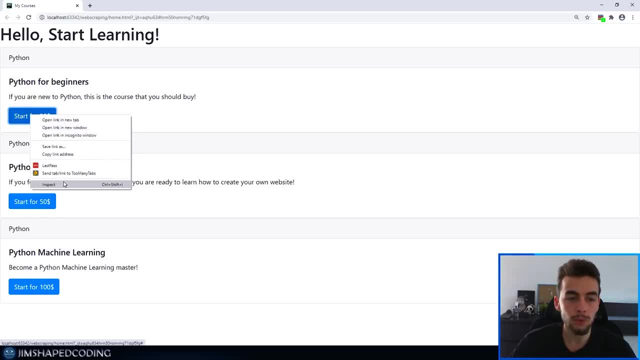 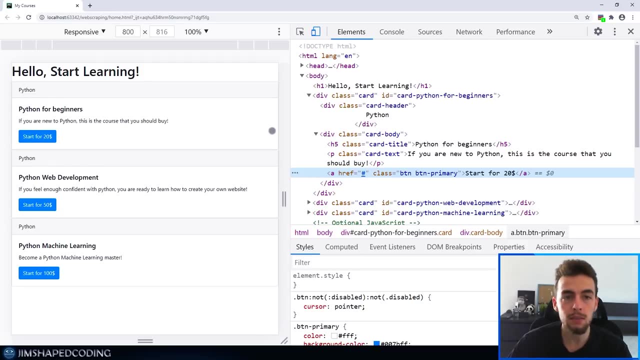 and then right click on it And then you want to look for that inspect option, And once you open that out you will have a new pane that is going to be opened, And then here we can see all the HTML code that is responsible to. 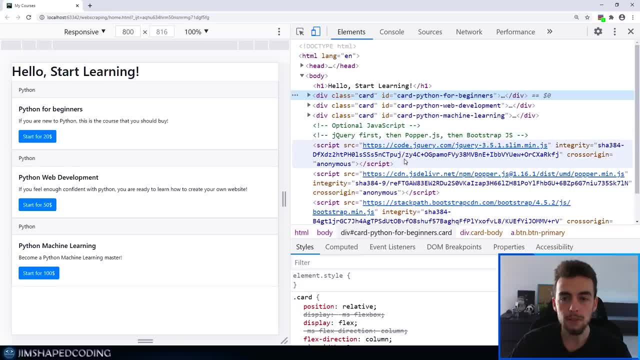 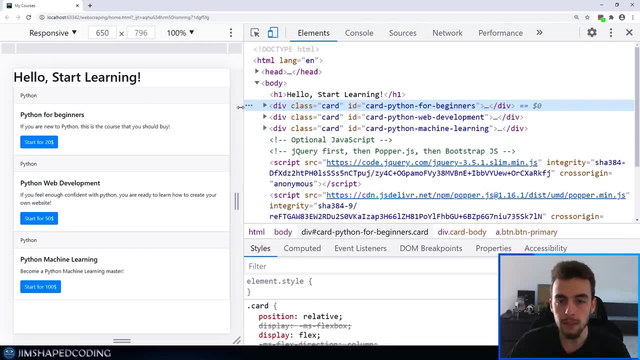 display what is going on on the left pane, So you can see that we have here- let's make it a little bit more bigger, So that will be enough. And then you can see that we have here div class card three times, which is the. 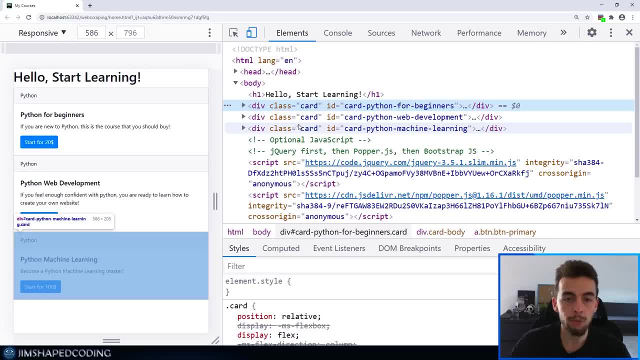 the displaying all the different courses. Now, when you go over different HTML tags with your mouse, you can see that it is going to mark for you the HTML tag that is related to it, So it is a quite important behavior that we should understand. Now let's say that we want to. 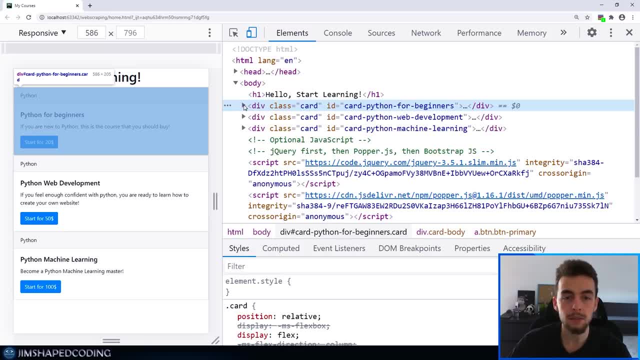 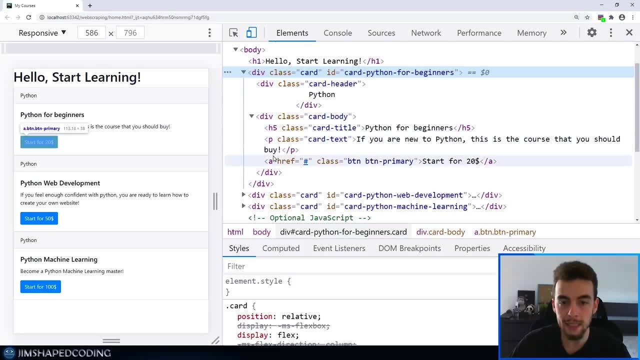 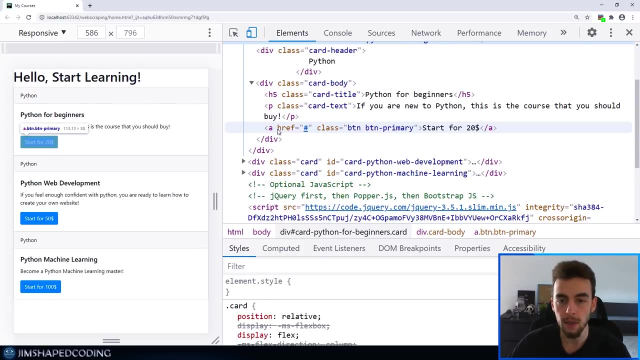 grab the price for that Python for beginners. So it makes sense to expand this tag and see what is inside. So I will go here and search for that button And you can see that it does this. a tag is actually responsible for that button itself And then you can see that its text is start. 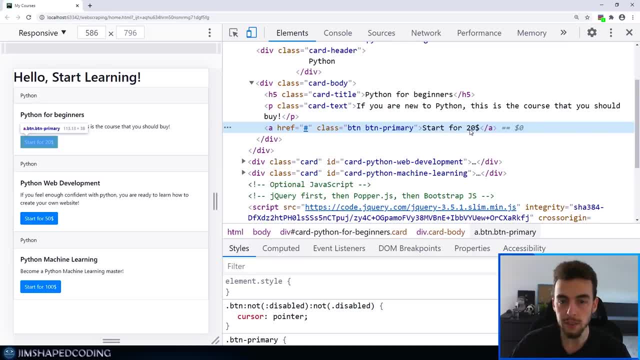 for $20.. So the price information is right there And let's actually write a program that is going to search for that Python for beginners, And then we will grab the price for that course And then we will be able to write a nice program that is going to include a list of all of the courses as 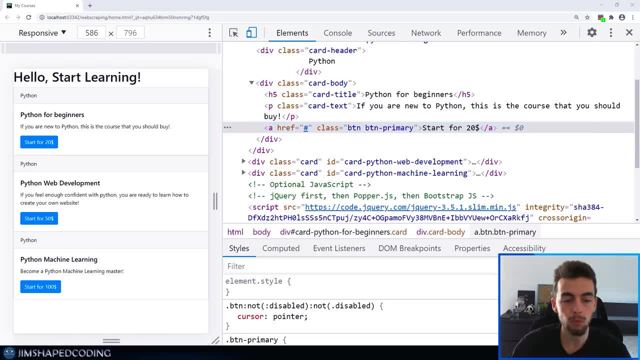 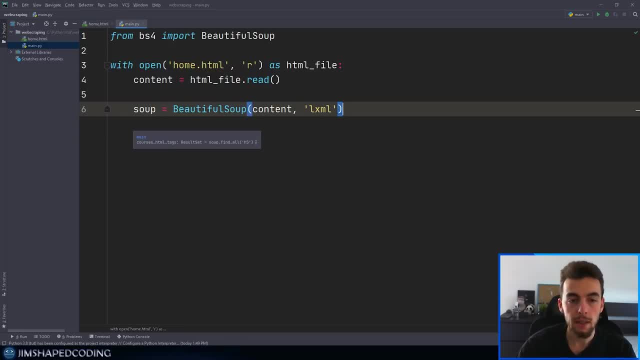 in the prices for each one of them. So let's go back to PyCharm and write this program. So we will go here and delete everything from here, And the first step that we probably want to do is to be able to grab all the course cards. So it will be course underscore cards equals to soup. that. 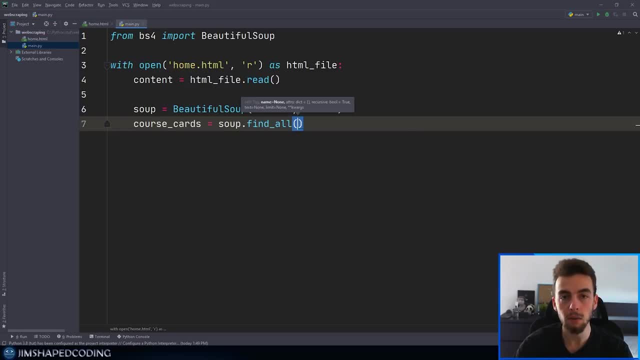 find underscore all, because we probably are looking to bring us back back all the cards. So this is why you have to use find all and not the fine, And I'm going to search for the div tags Now. it could be much nicer if we could filter the div tags that we 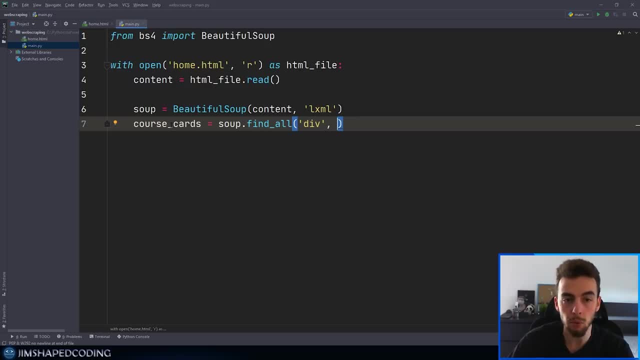 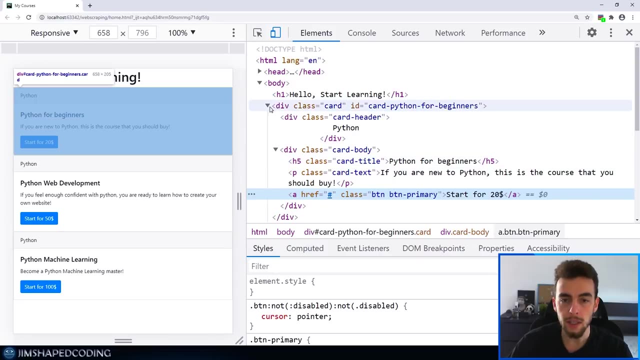 actually want to grab and store it inside our course cards. So if you noticed, let's go back to our courses fight page And here, if I just expand back there all the div tags, you can see that there is something that is common. 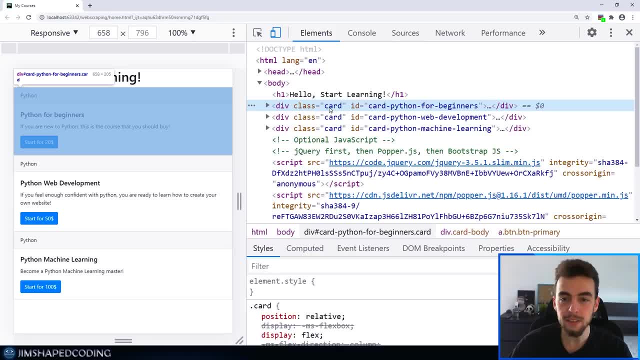 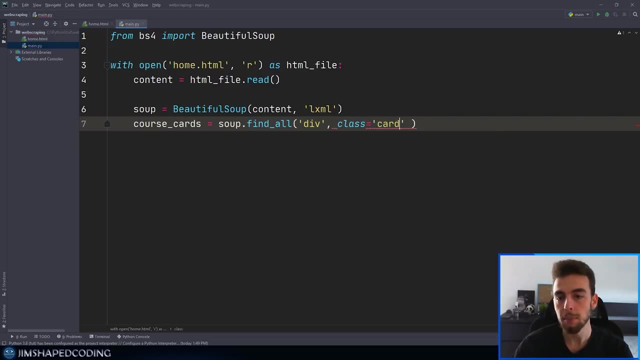 For all the div tags. their class is equal to card. So I can filter my div tags by this expression right there. So I go back to Python and I will write here: class equals to card. But now you can see that there is an error and it is quite important behavior to understand. you have to. 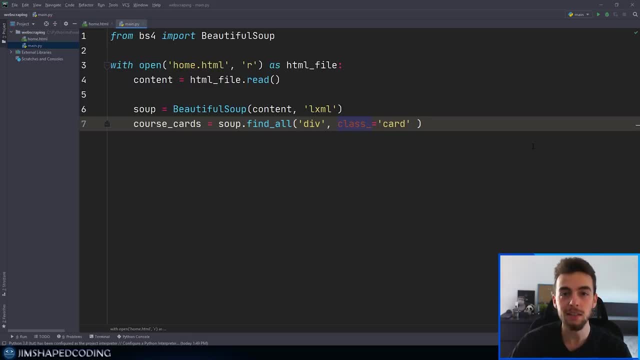 apply here the underscore, because the class is a built in keyword in Python where you create Python classes. So that is why you have to add the underscore over here And then the beautiful soup will understand that you are relating to the class of the HTML attribute. 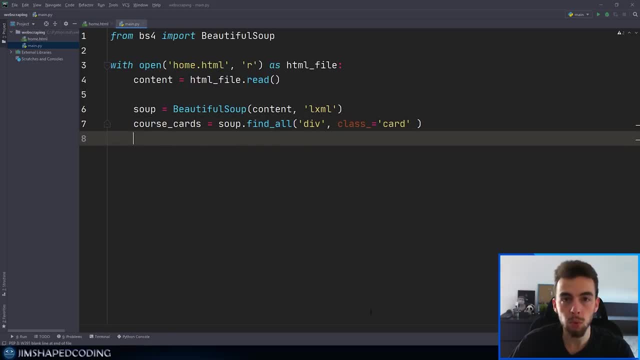 Okay. so it is important Now, since we have all the course cards stored right in this variable, then we probably want to iterate over this list and then search for the course name and then the course price. So let's see how we can do that for each of our course cards. 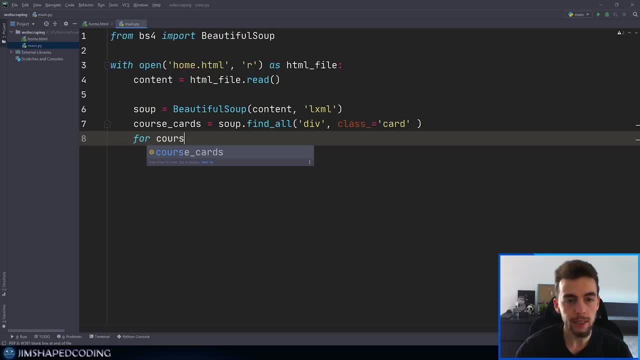 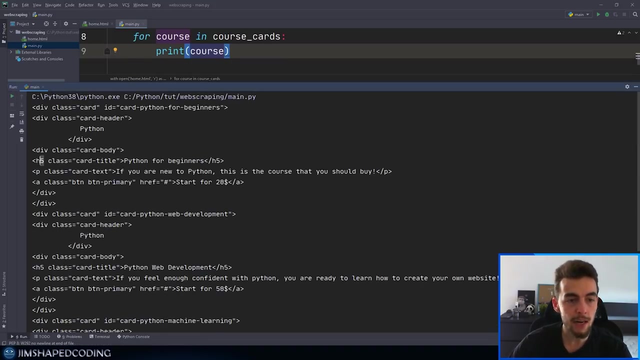 So we will start with for loop here And that will be for course in course cards. And before we go ahead and write some more code inside our for loop, let's actually remind you what is inside each of our courses And then you can see that we have h5 tags on each of our course cards And it makes 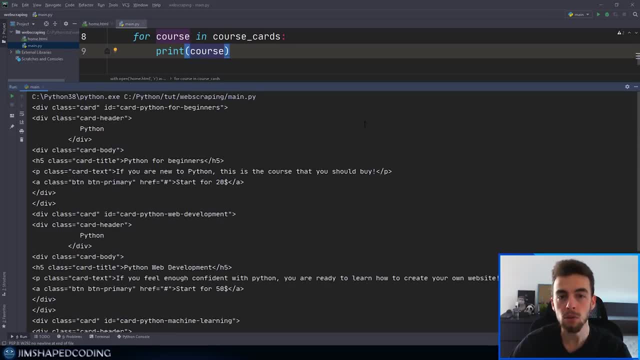 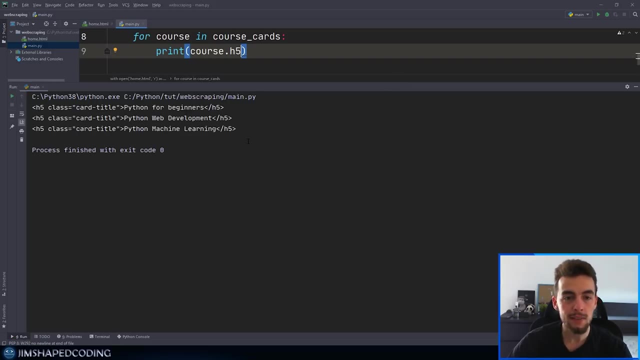 sense to access these specific h5 tags. So we can accomplish that by going here and then using the h5 tag as an attribute. So if I go ahead and press you dot h5, and rerun my program, then you can see that we were able to grab each of our h5 tags. 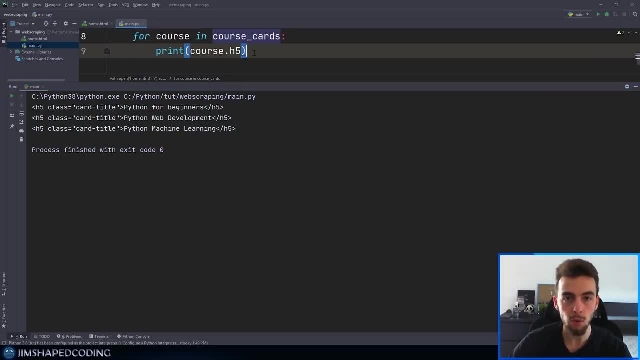 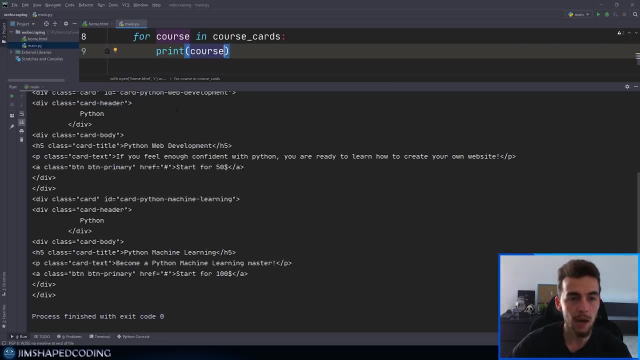 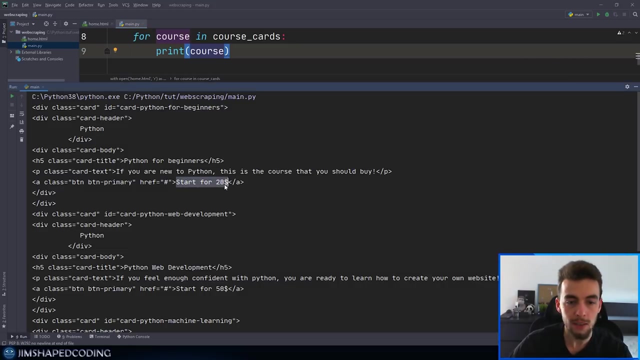 that are inside the course card. So it is a quite great thing. And now, if I revert this back to course again and run that out, you can also see that inside our a tags we have the for start for $20.. And that is repeated for all of our cards as well. So first of all, 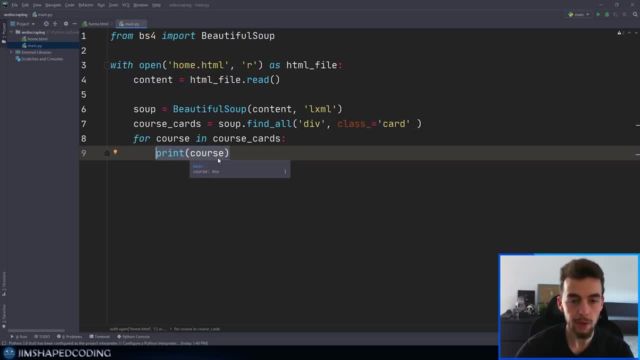 it makes sense to delete this again. And right here is something like: course name equals to course dot h5.. And then here we probably look for the text attribute of that h5 tag. So I will write here: dot, txt And then this course name will be responsible to store the. 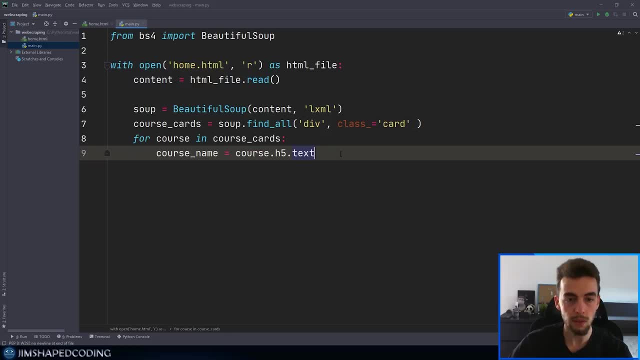 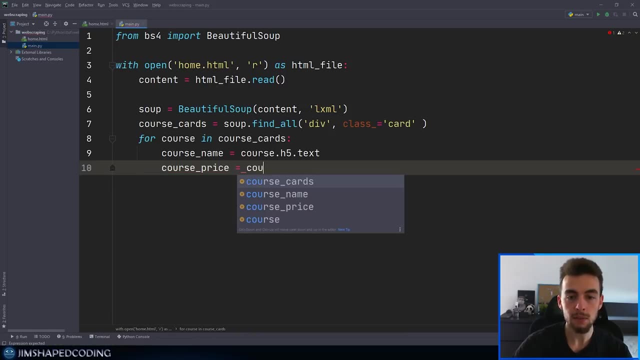 text on each iteration. So it is great, And now I can go here and write the course price And then this time I will search for course dot a, because the a tag stores the information about the course price. So until now, if I go ahead and print the course name and then 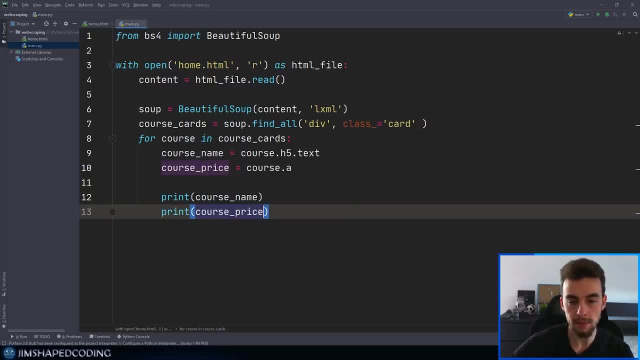 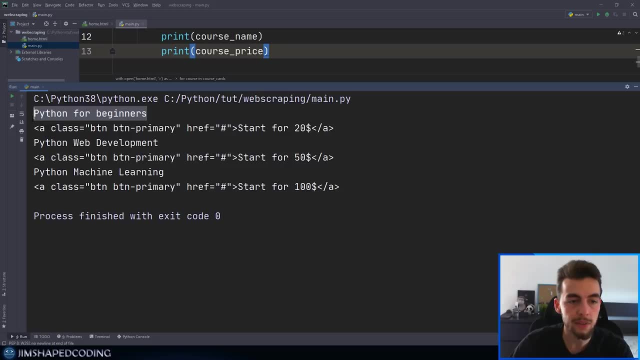 I also go ahead and print the course price. then we will see the results like the following: So you can see that we have Python for beginners And then we have the a tag itself, But in this case we look for the text of that a tag as well. So I will minimize my terminal. 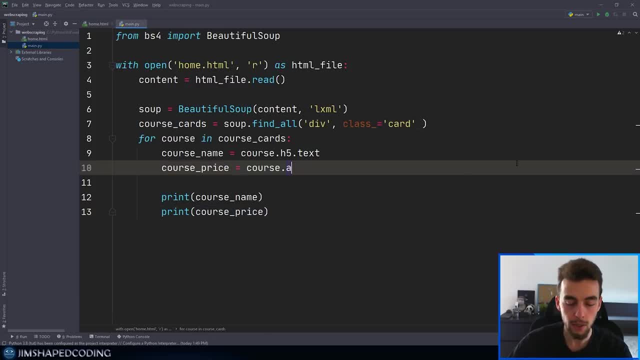 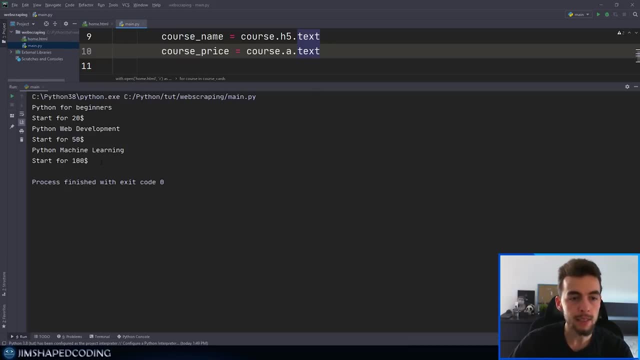 out And excuse me for that. I will delete that from here And then search for the text attribute over here as well, And now I will run my program And then you can see that we have Python for beginners and then we have the text for each. 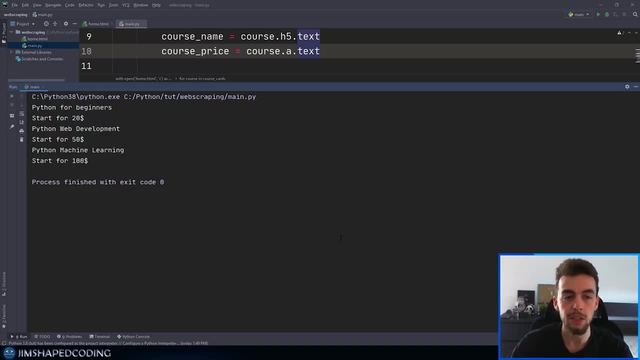 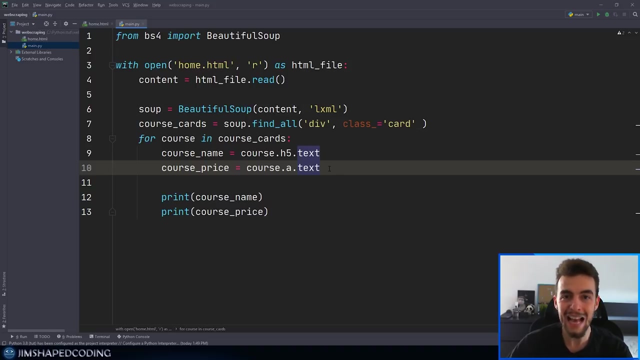 of our a tags, And now, since we reached this stage, it might be a greater idea to print a sentence like: Python for beginners costs $20, Okay. so the way we can do that is basically using the split method to access that last element of that text, because the price is. 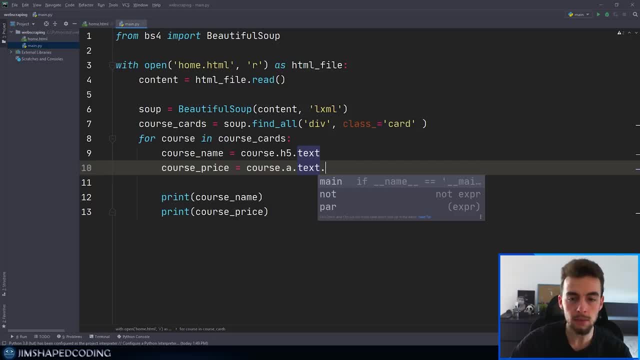 located as the last word. So it makes sense. it makes sense to go here with split And then we will split it by the blank. So we don't have to specify anything here And we want to grab that last element. So we are looking for minus one. 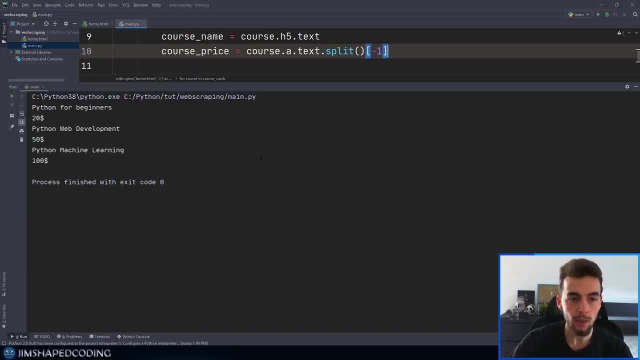 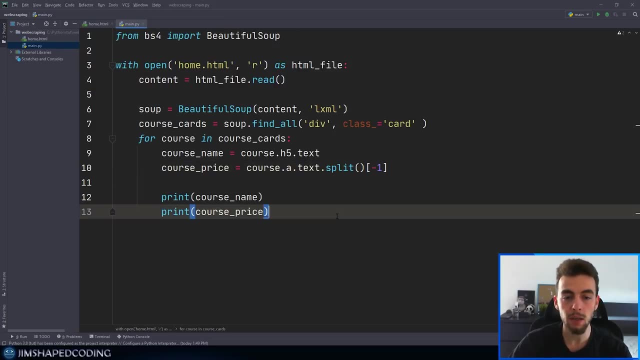 index over here, And now, if I run it, you can see that we have the price for each of our courses, And now it might be much nicer if we go ahead and use an F string to print a dynamic sentence for each of our courses. So we will go here with print And then we will open an F string And then 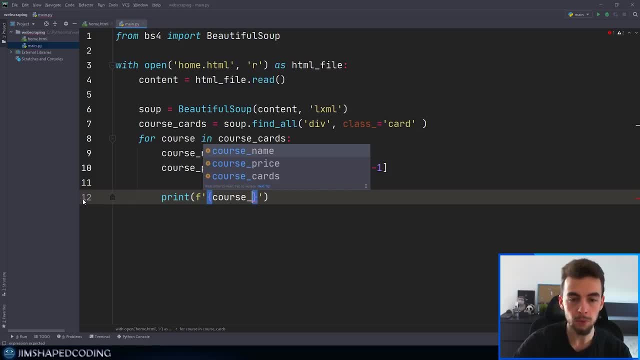 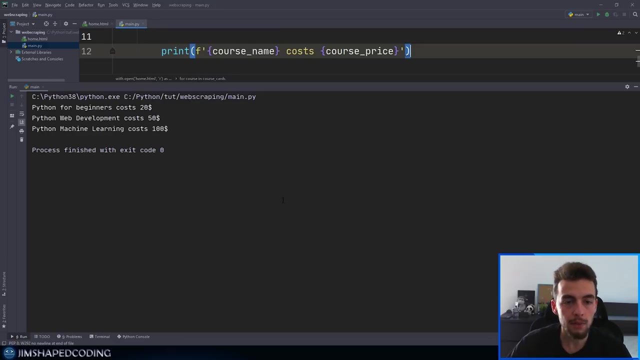 we will access the course name, So it will be course underscore name, And then we will write costs And then we want to display the course price, So it will be course underscore price. Now, if I run our program, then you can see that it displays a nice information about. 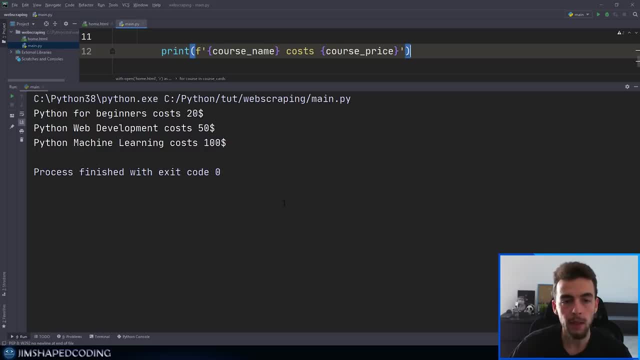 each one of the courses. Now, if you think about it, that is a quite nice behavior that we have applied here, Because if you scrape a real website like Udemy that keeps updating courses, then it might be a great idea to launch this program every certain amount of time, for example each week, and then you have the 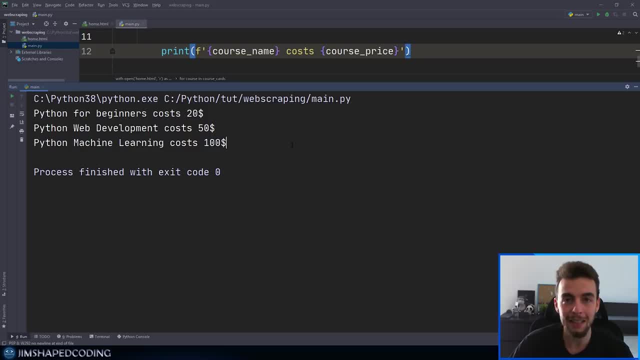 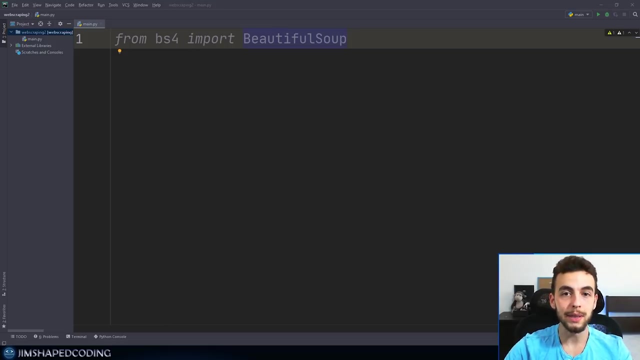 ability to be aware about each of the courses that Udemy has updated on the web page that you scrape on. So this is a quite nice behavior that we were able to reach here. On this one, we are going to scrape real websites with the requests library, So I'm going to 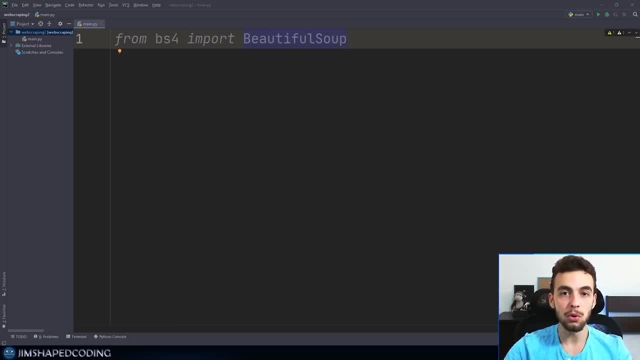 simulate this against the website that is going to search for job advertisements And I'm going to bring all the jobs from a specific website that their main skill requirement is Python programming language, And I'm going to write a program that is going to pull the latest published. 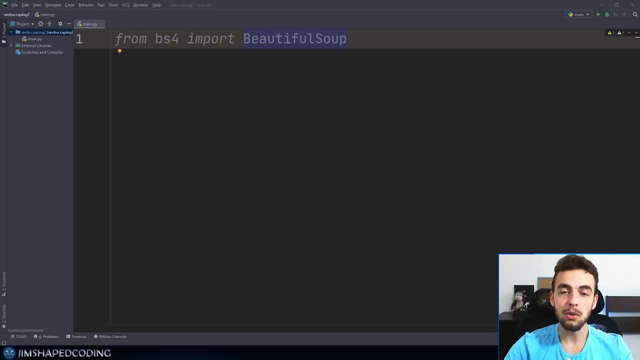 job advertisements from a specific website. So it is going to be very interesting, So let's get started. Alright, so one of the first things that we must do is to ensure that we have the request library installed, So I'm going to go down to my terminal. 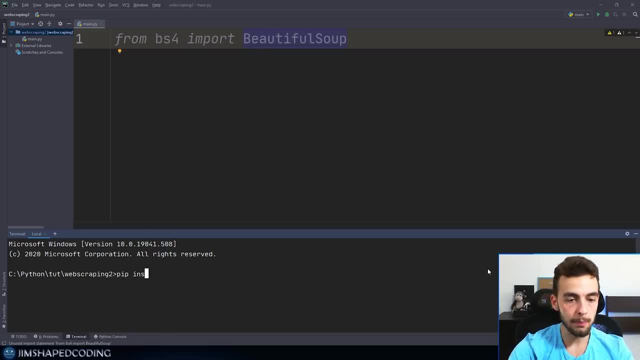 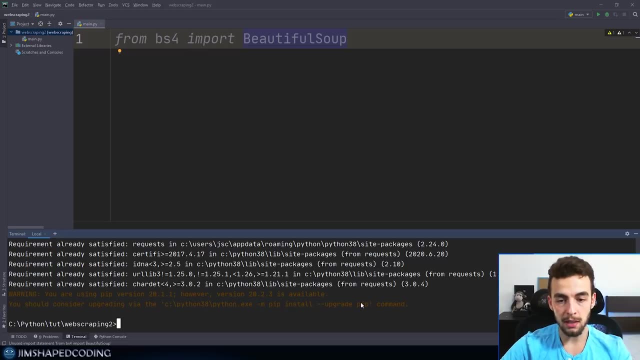 right in PyCharm And I'm going to write here pip install requests just to make sure that I have the request library installed. Now. the output for myself could be different than yours, because you may not have the request library, But since I already have that you. 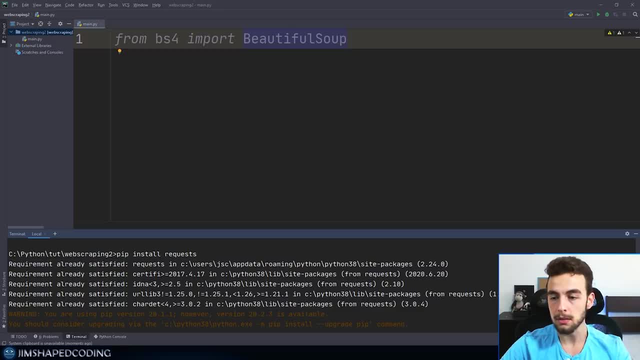 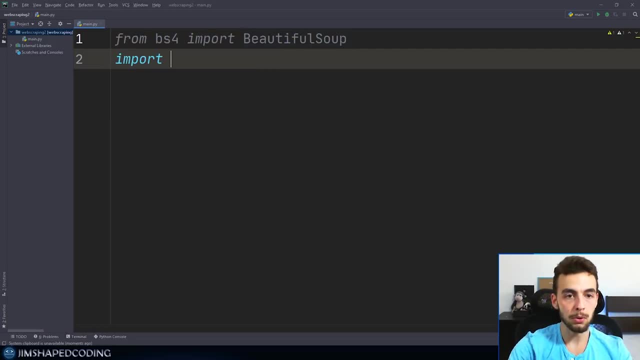 can see outputs like requirement: already satisfied. Okay, so it is quite important. Now I'm going to minimize the terminal And, right here, import requests. So we want to make sure that you do that after the installation of this library And the first thing that I'm going to do here. 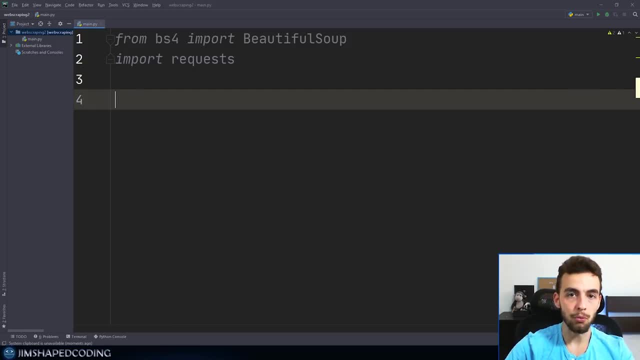 is to use the get method of the request library. Now, what request library is doing behind the scenes? it is just requesting information from a specific website. It is like a real person going to a website and requesting some information. Okay, so you can go with something like the following when it comes to request library: So it will be. 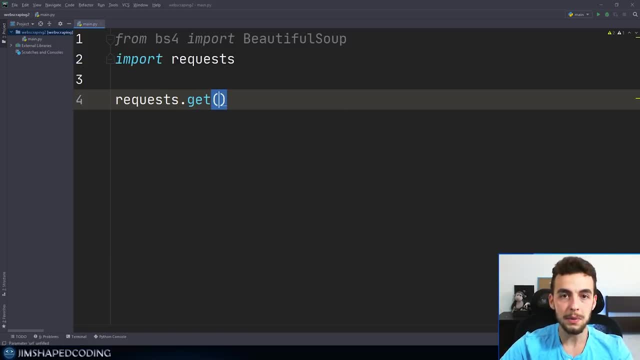 requests that get. so you want to get specific information from a website, And here we are going to provide an empty string string for now, But later on we are going to complete this string with the URL that we are going to web scrape against it And I'm going to assign this to an. 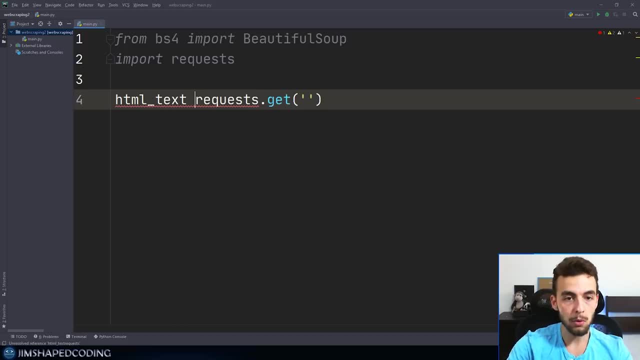 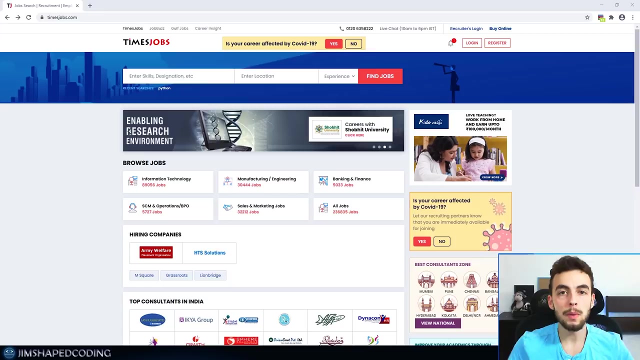 variable and I will call it HTML text, So I'm going to make that to be equal to this entire statement. Now let's go to a web browser and look up for the website that is going to include some job ads. Okay, so this is a time jobscom, And this website includes job posts about almost 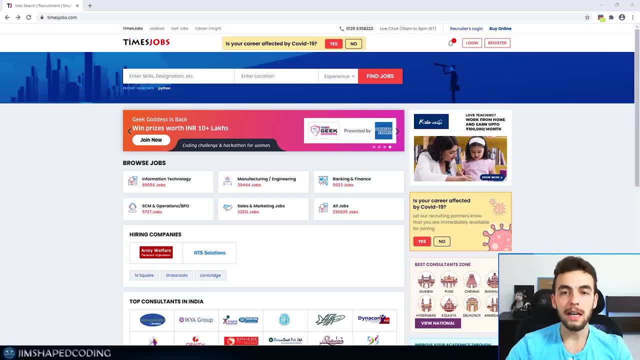 everything. So you can simply go down here and search for some skill that you own, And then this will search for your jobs that are requiring specific skills in that position. Now, this video is recorded a couple days before when I uploaded it, So if you watch this video after a couple of months, or even a year or two since the published, 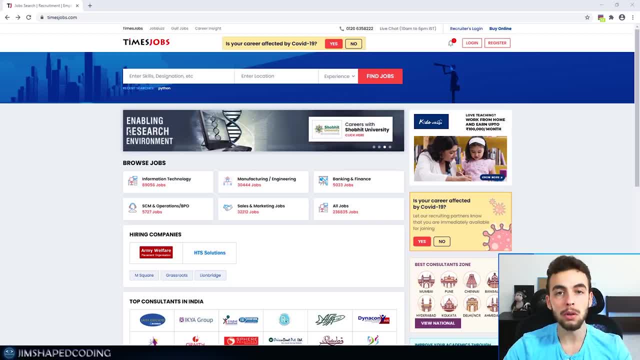 date, then there is a great chance that the HTML elements are going to be quite different. But the main point of this video is to teach you all the tools to pull information from a website just as you want, And then you can apply your own customizations and kind of doing. 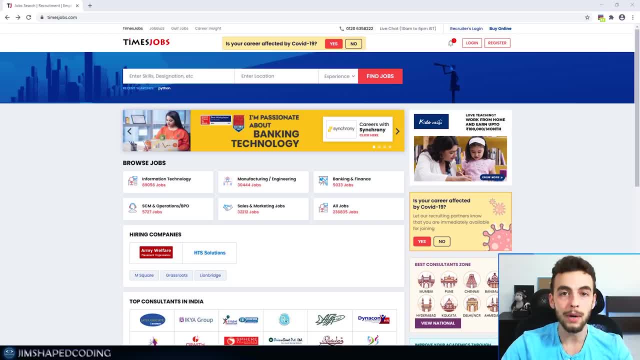 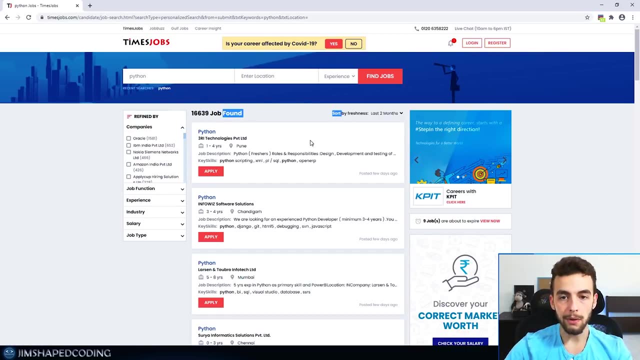 a reverse engineering to the code that I'm going to write through how this tutorial. great, So let's go here and write Python. So I will receive only job posts about this programming language, And you can see that we have this job found over there And we have a lot of jobs that are published. So 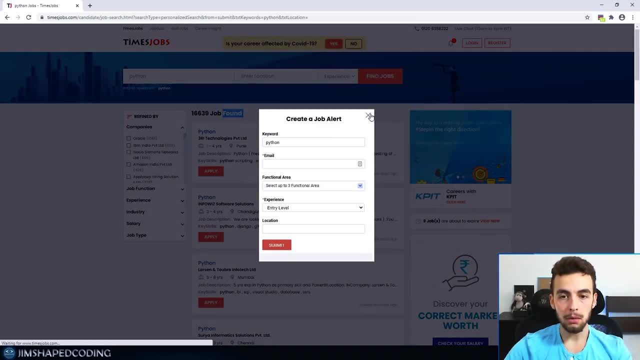 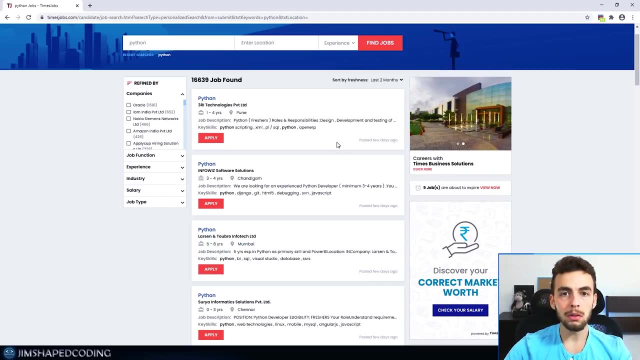 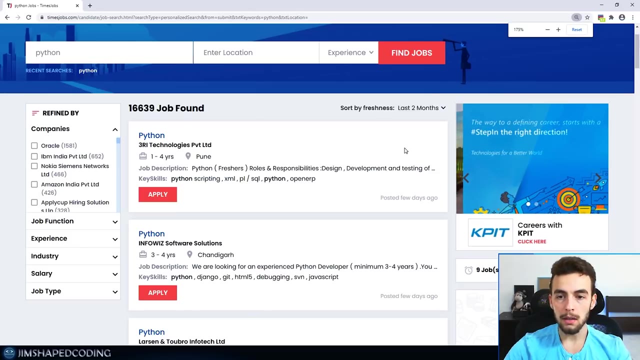 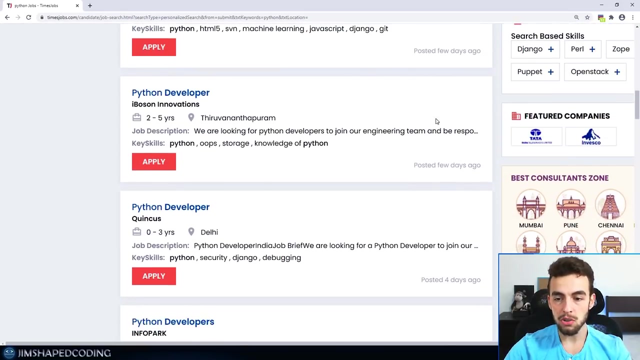 my goal here in this tutorial will be to let's get this closed. So my goal in this tutorial will be to bring all the jobs that are posted a few days ago. So if I am zooming here in then you can see that we have posted a few days ago for a couple of posts. But after I reach down here we have posted. 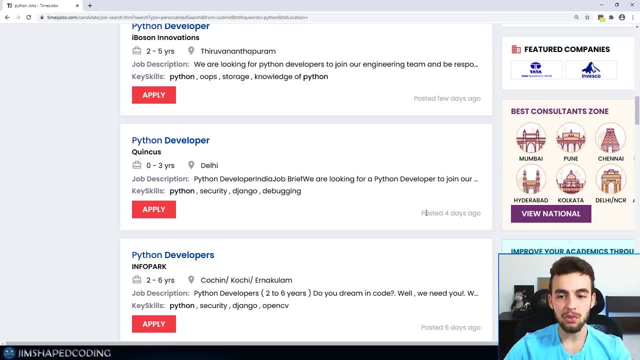 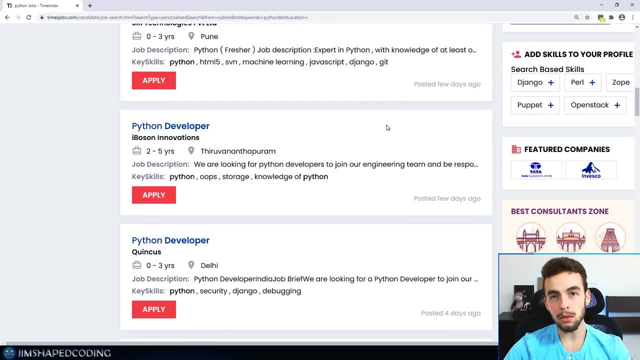 four days ago. So this might mean that this Job post is not the most updated. So I'm going to bring all the jobs and I'm going to condition my program to bring those elements with the posted a few days ago text only. So let's go back to here. 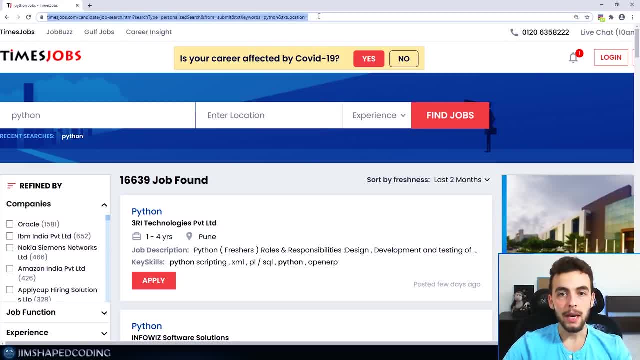 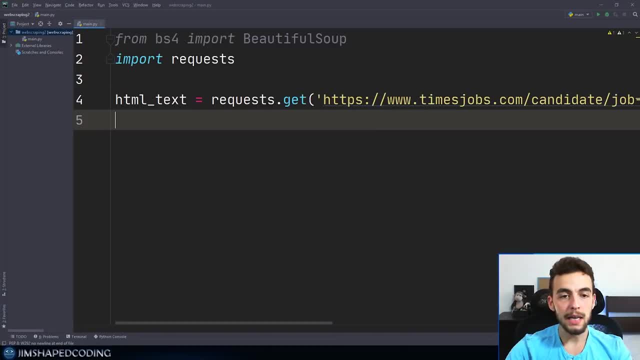 Now I'm going to bring this URL from here And I'm going to paste that in in the empty string that we created inside the requestget, And once I have done that, what is going to happen is that all the jobs will be in the same place, So all the jobs that are posted in the 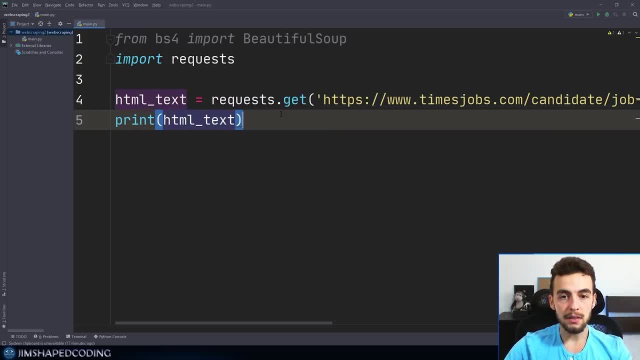 on inside this variable right now is simply the request code status. Okay, so if I'm going to print the- I mean if I'm going to run this program- then we are going to see the results like the following: So 200 is the convention number in web that the request is done successfully, But in 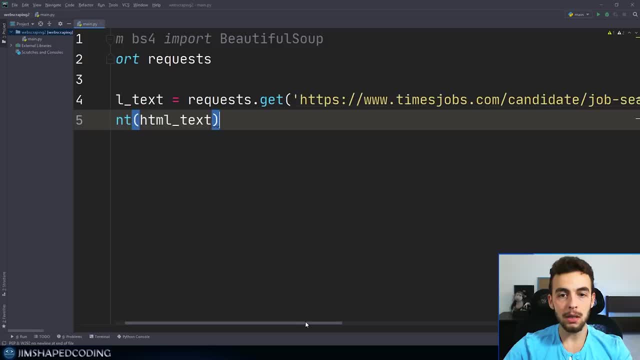 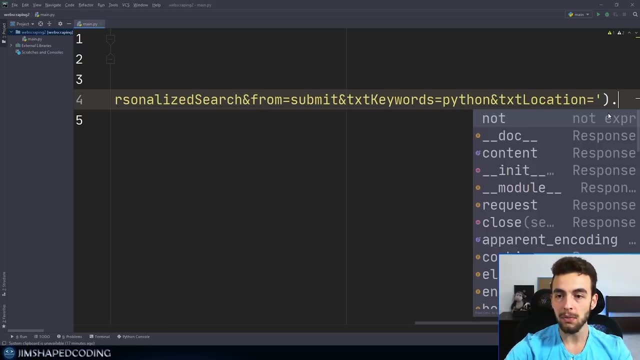 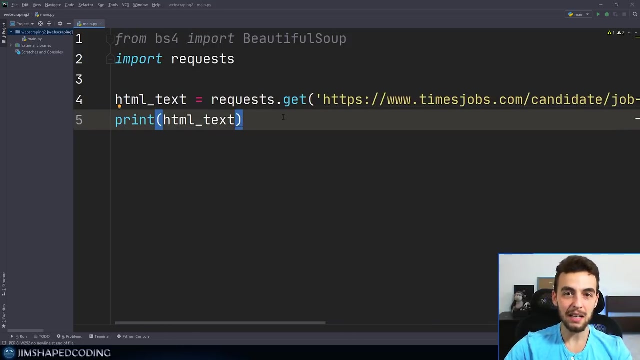 order to avoid the status code. we are going to go to here and I'm going to accept the text only, So I'm going to go here and then write that text. Okay, so this is what we have to apply here in order to bring the HTML text of that specific page, And now it makes sense to leave this variable. 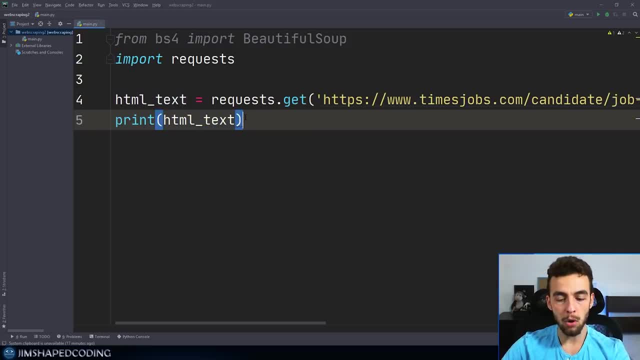 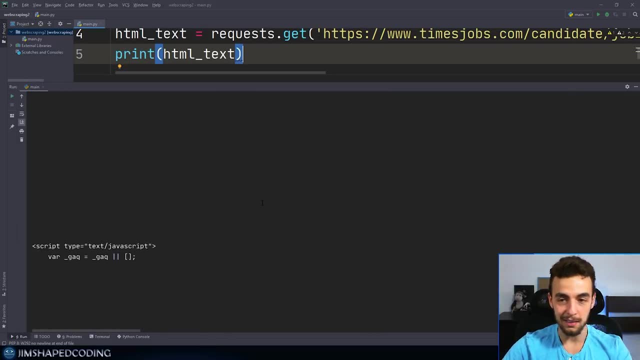 name as it is because it is storing the HTML text And I'm going to rerun this program And we will probably receive a large information of HTML. So right now it is not quite relevant, but I'm just. I just wanted to show. 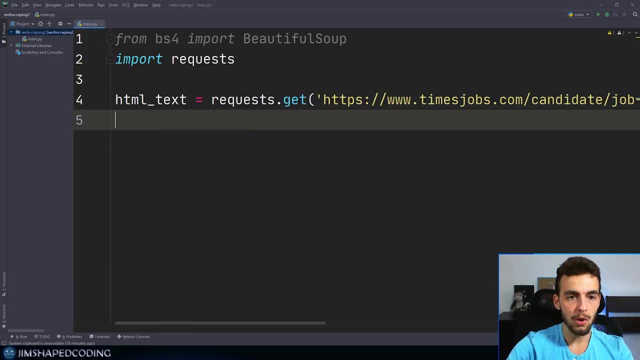 you the results. So let's continue from here. Okay, so, as you know, we are going to create a beautiful soup instance, like we did in the previous episode, And I'm going to provide the HTML as the HTML text variable. So it will be: soup equals to an instance of a beautiful soup, And then I'm going to write: 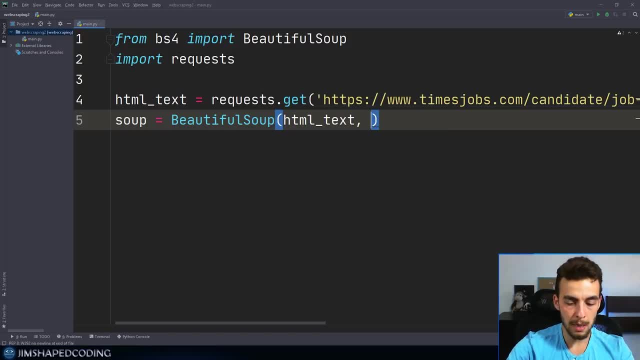 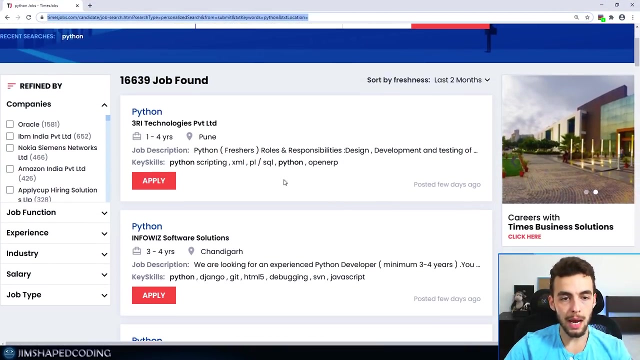 here HTML text as my information that I want to scrape, And we are going to use the same parser again, like the previous episode, So it will be L XML. Now, once I have done that, it makes sense to go back to our page and see how we can grab only this, each paragraph, from this website. So the 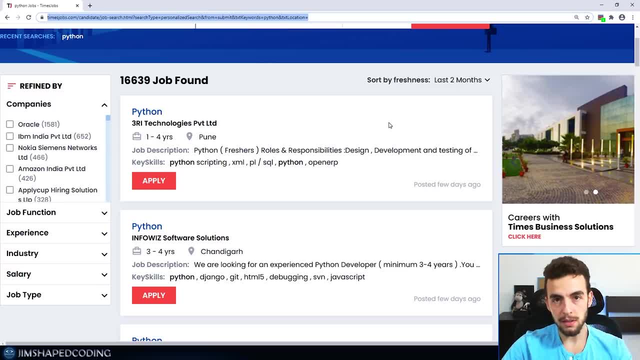 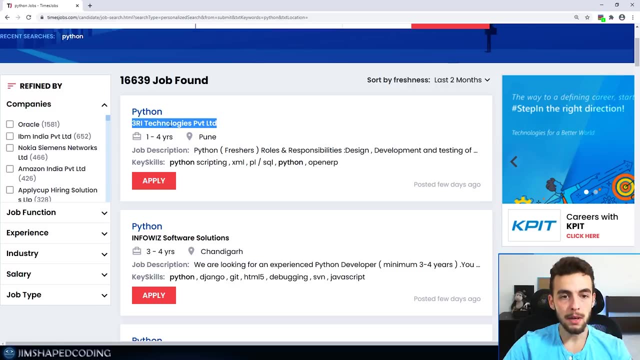 white boxes are kind of a list of elements that this page has provided here And I want to look for a method that is going to bring me all the job posts. So it makes sense to catch a certain element inside that post And right click on it and then click on inspect. 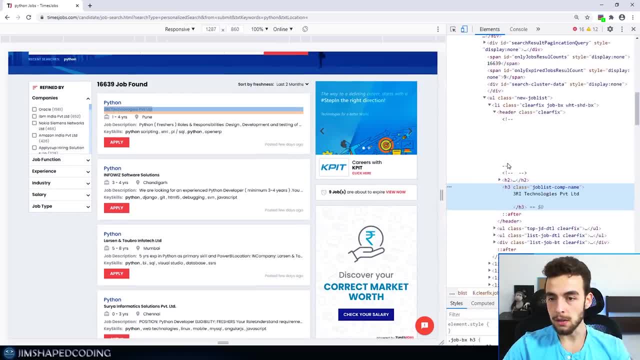 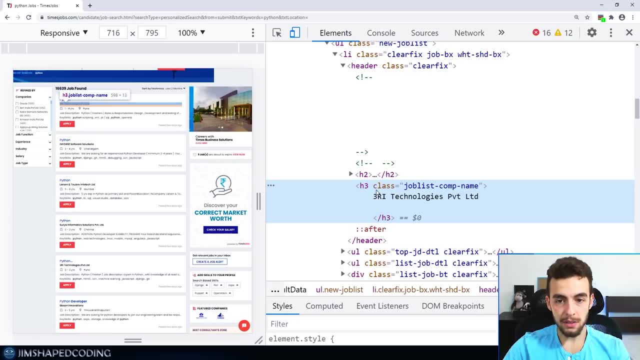 And once I have done that, you can see here. so I'm going to zoom in things a little bit So we can see that the h3 class is pointing to that text over here. I know that the text is not is a little bit small here, But just you can see that it has a gray mark And I'm going to go up. 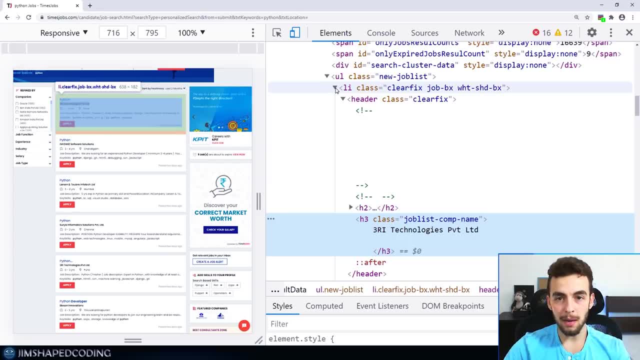 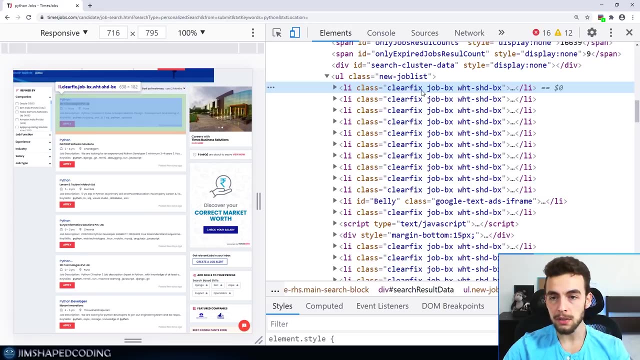 here And then you can see that those elements are opened up as well. So if I hover my mouse here, then you can see a green background wrapped in the article over here I mean the paragraph- And then if I close that up you can see that we have a lot of clear fix job dash p, x and something like that. 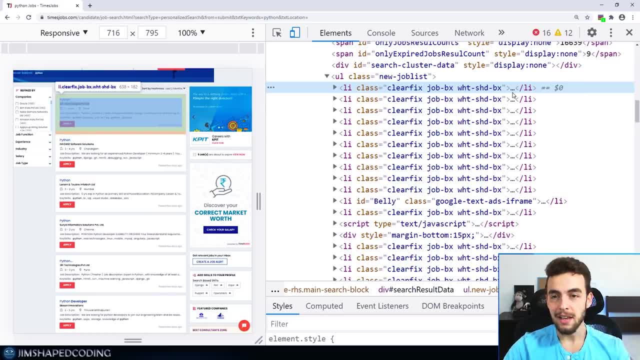 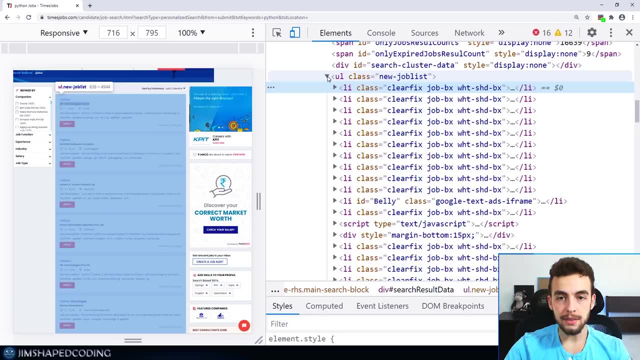 that its name is the class And our HTML element here is called Li, So Li stands for list, And then you can see that it is inside a UL tag. So this is standing for an ordered list and it is containing a lot of list tags inside that UL. So you can see. once I close that. 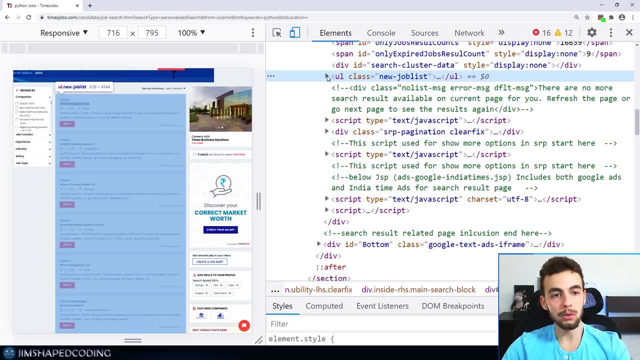 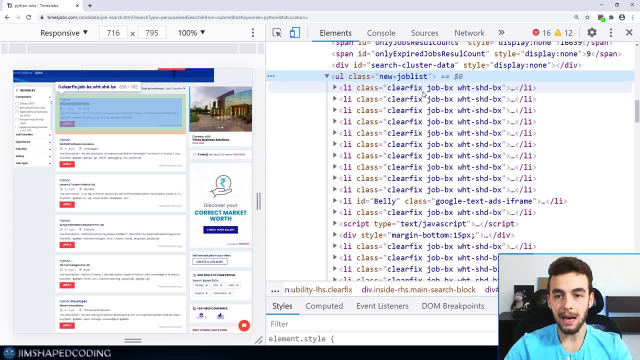 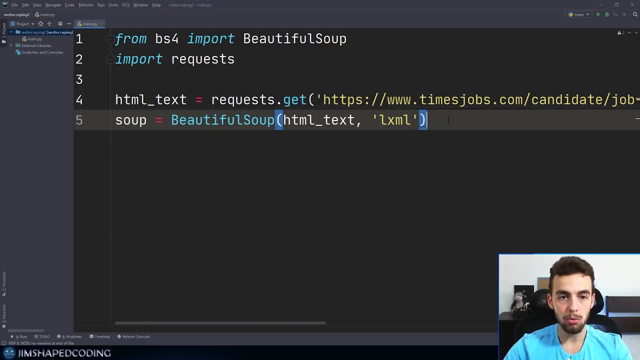 then the entire list of all the posts are marked with a blue background. So I'm going to search the element of Li with that name of class, So I'm going to copy the name of the class here And I'm going to go back to my Python And I'm going to write here: jobs equals to. 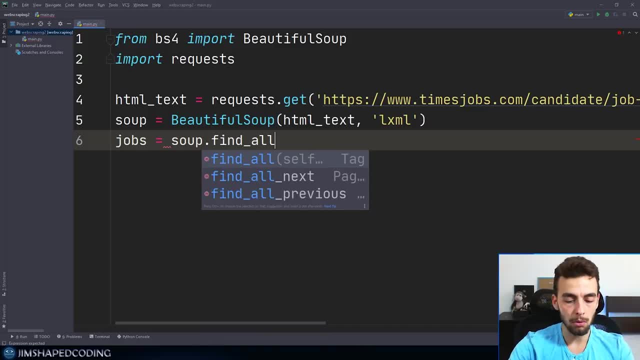 soup dot find underscore all And I'm going to search for all the allies. And as the second argument, it makes sense to pass your class underscore equals to, and then, inside that string, I'm going to paste that in the class name. that we have copied from the page itself. 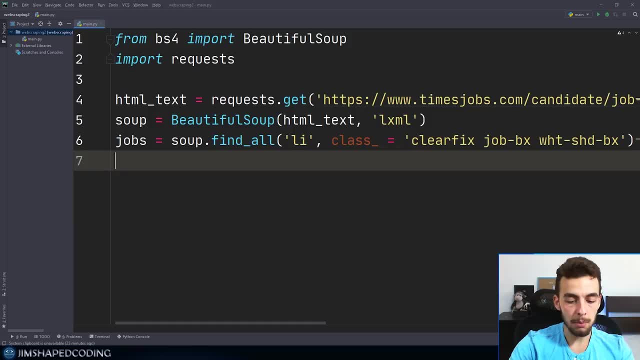 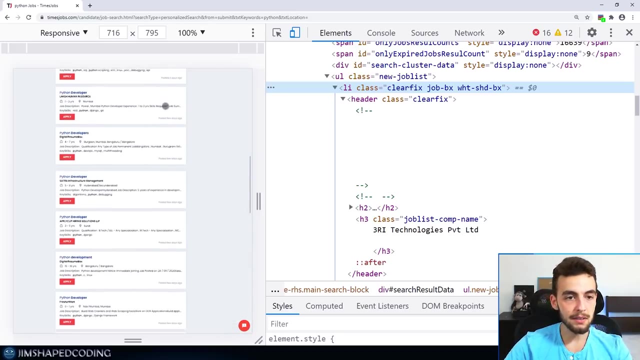 So once I have done that, then we will probably see the results of all the jobs in that page. Now, this doesn't mean that it is going to bring back all the 16,000 jobs, because you can see that this page is being paginated, So that means that it is going to bring. 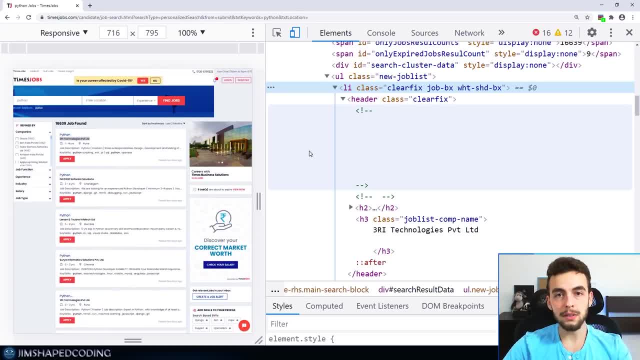 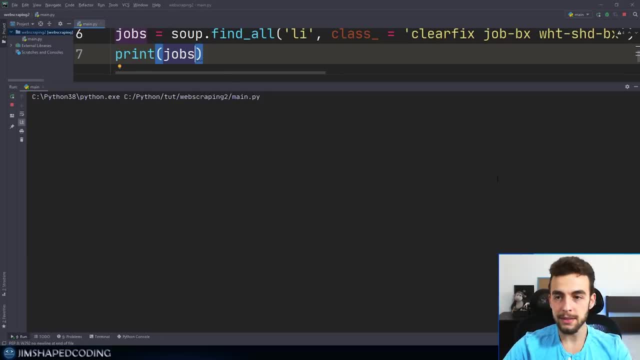 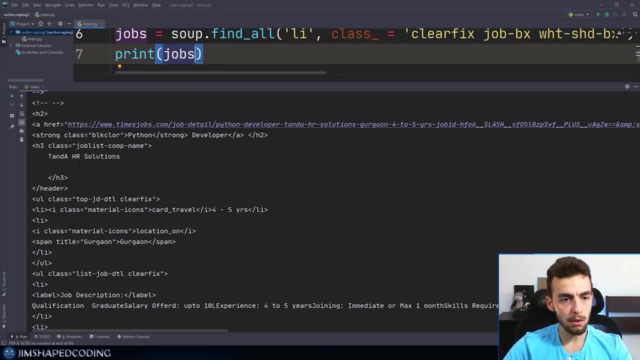 the results only for the first page, So this is not going to take extremely long. Now if I go back to here and paste the jobs, then let's see the results before we continue on, just to make sure that everything is okay, So we can see that we receive the results And then we see that we have 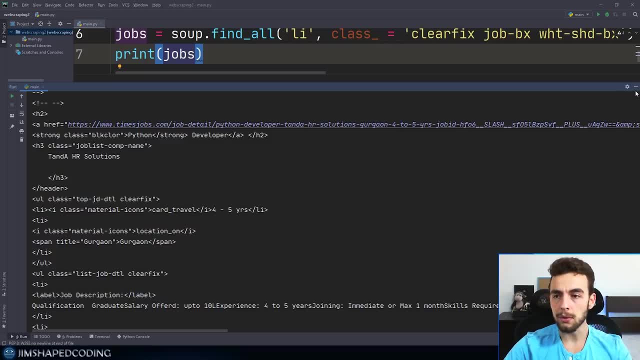 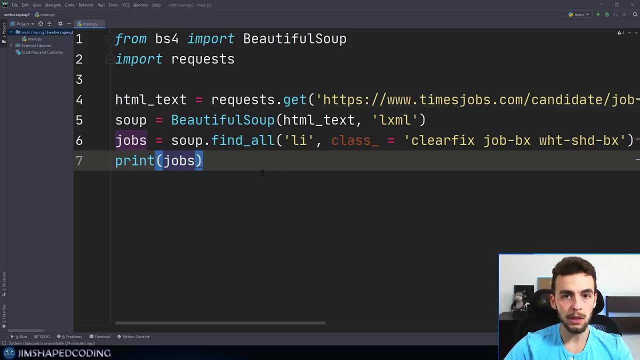 some company names And I think that everything is quite great here. Now, in order to work with this scraping project, it makes sense to only work with only one job element, So I'm going to delete the underscore all from here And what this means. 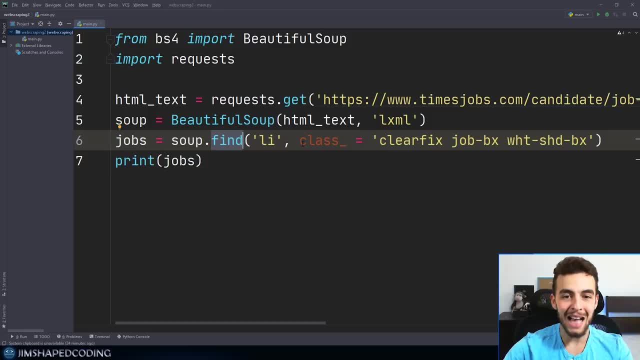 it means that it is going to bring the first match that sees the li tag and then the class name as this string over here. So let's change this variable name just to job, for now. Okay, just in order to develop our program slower relying on only one job post. Okay, so once we 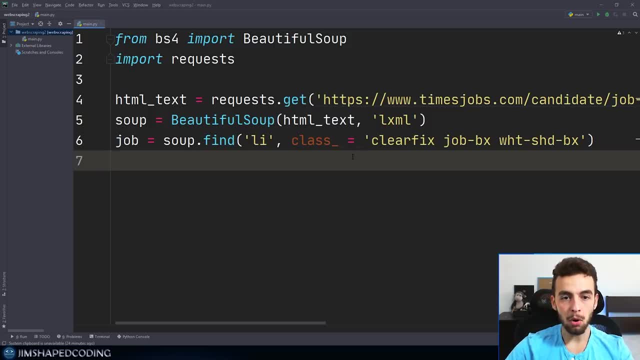 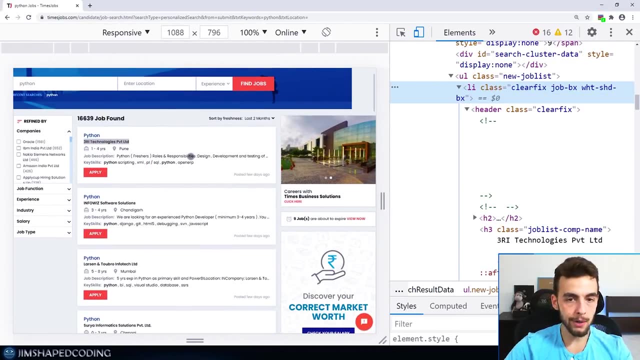 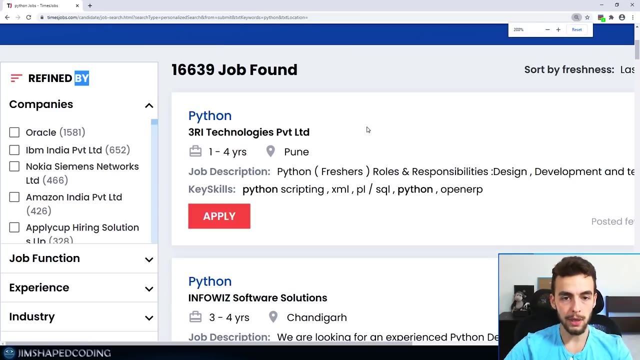 done that, we probably want to search for the company name of that specific job post. So I'm going to go back to here And I'm going to make things bigger over here, And now let's actually go here and try to inspect what is going on here again. So let me zoom that out, Great. 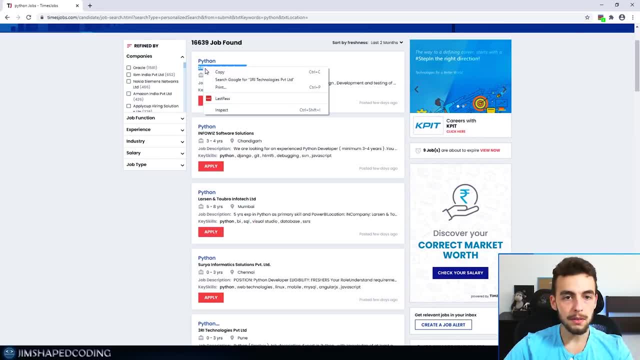 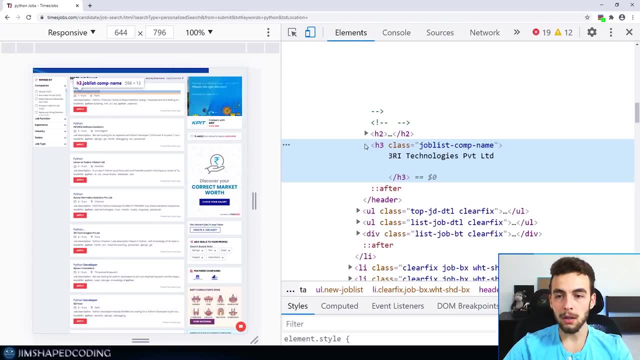 Now I'm going to try to inspect this text over here again And then we can see that it is inside the li tag for sure. But we can also see that it is inside an h3 tag And it has the class name of job list- comp name. So I'm going to search for that class in the entire page as well. 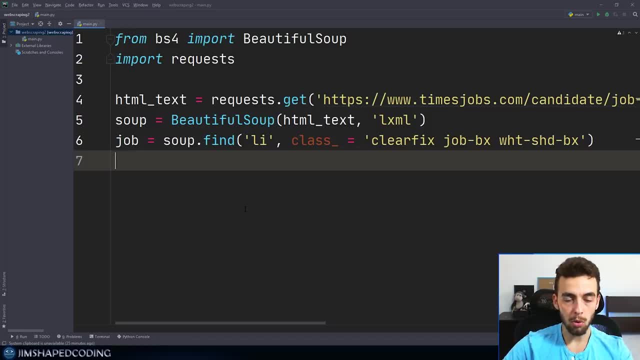 But speaking about the entire page. so let's go to our Python. you want to search for that specific element only inside the job itself. So you'll see, it doesn't make sense to search for an h3 tag in the entire page again. So you can basically go with job dot find. 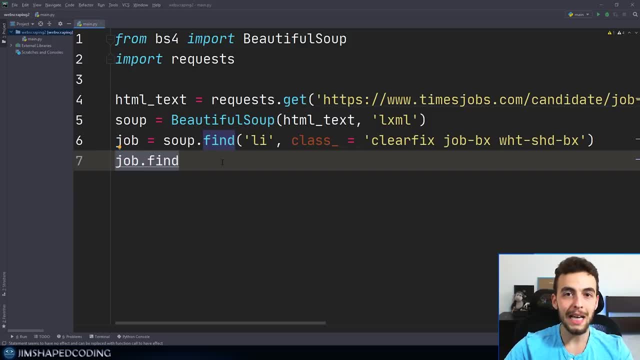 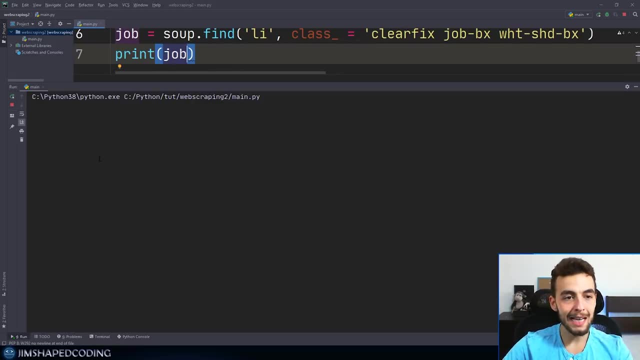 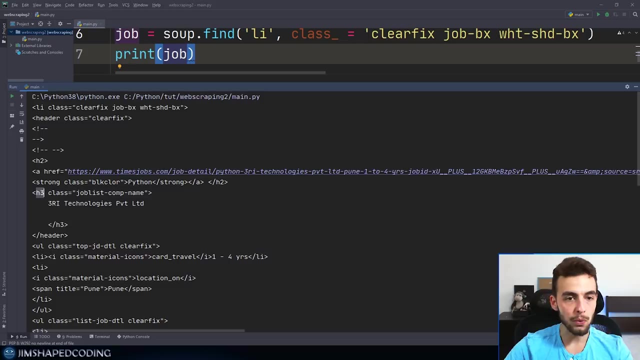 besides soup dot find, because we want to search for that h3 tag only inside our job. So if I go ahead and print the job here, then we can see that it only includes an HTML code about only one job And I'm going to search for this h3 tag. So let's create here a new variable And I'm going to 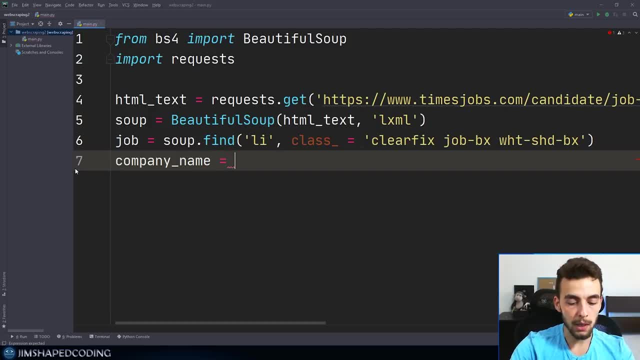 call that company underscore name And we are going to use job dot find And we are going to accept here as an argument the h3. And then this time the class underscore is going to be equal to whatever this h3 tag includes as the class name, which is the job list comp name. Now to debug this: 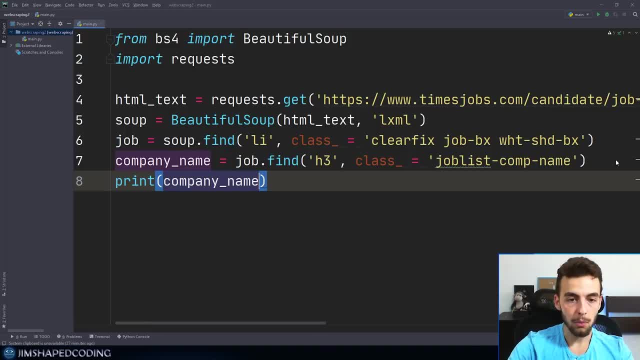 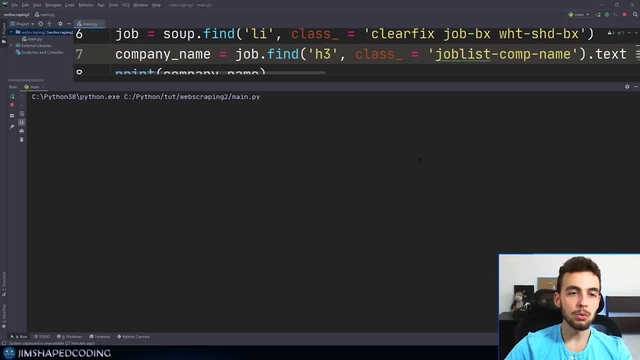 out And to ensure that the results are great, we are going to print the company name And then you can see that we receive this, this element, back, And I'm going to use here the dot text method just to bring back the text itself. Now, once I do that, we are going to see a weird 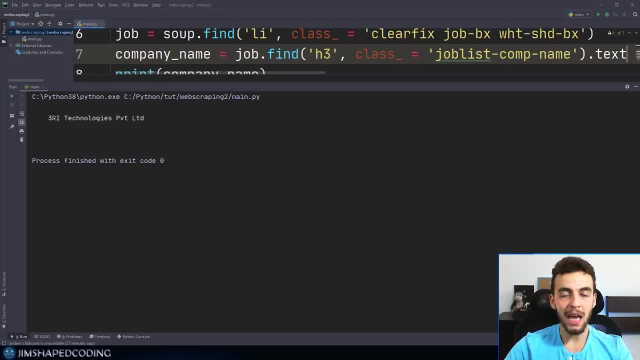 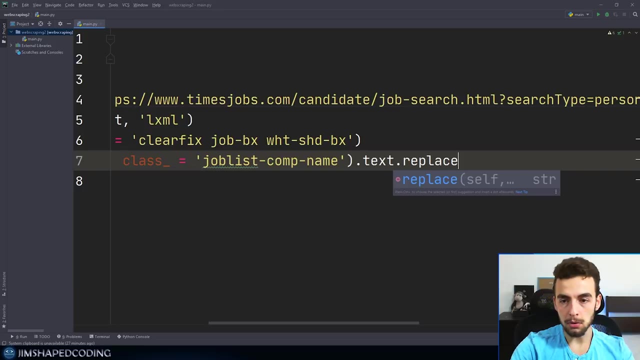 result here. Now you can see that we have some white spaces, So we kind of want to replace our white spaces with nothing. So in order to do this one, I'm going to go here And I'm going to use the replace method, And this trick is going to avoid having this not necessary white spaces. 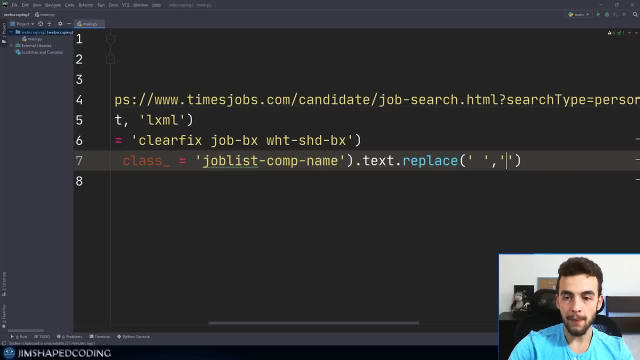 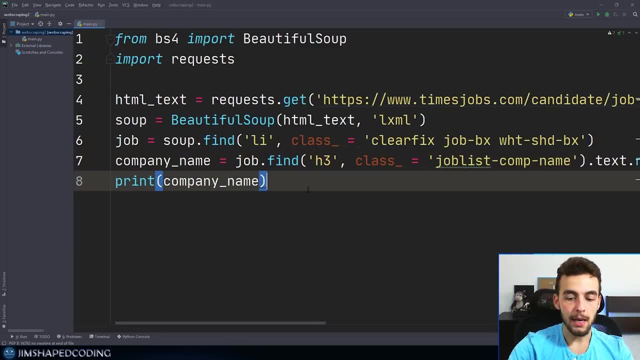 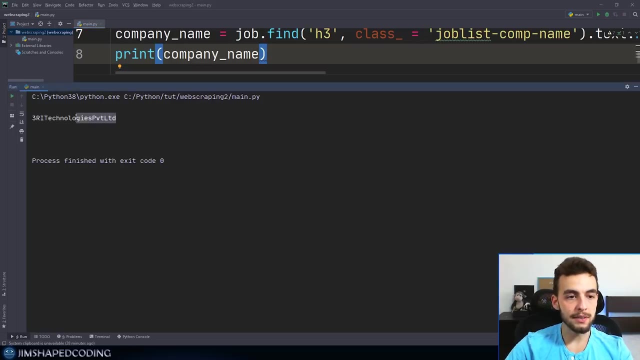 So I'm going to replace the spaces with nothing, So I'm going to just write here double quotes twice- I mean single quotes twice- And once I have done that and rerun our program, then you can see that the result is going to be quite different. As you can see, this text is fully aligned to left. 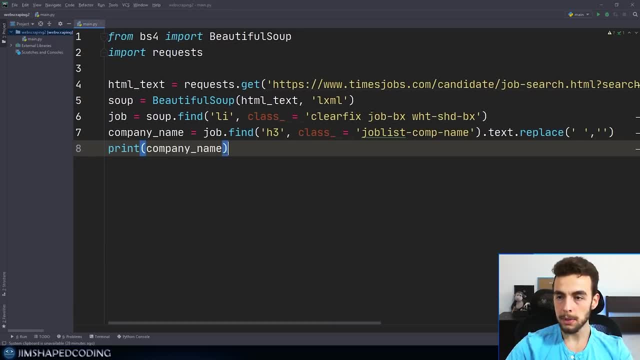 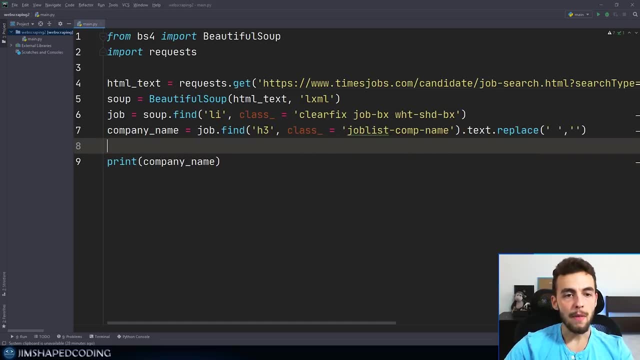 continue from here. Now we're going to zoom out a little bit the code here. just we can see the important points, like the replace method. And let's continue from here Now. it also makes sense to bring the skill requirements other than the Python programming language. 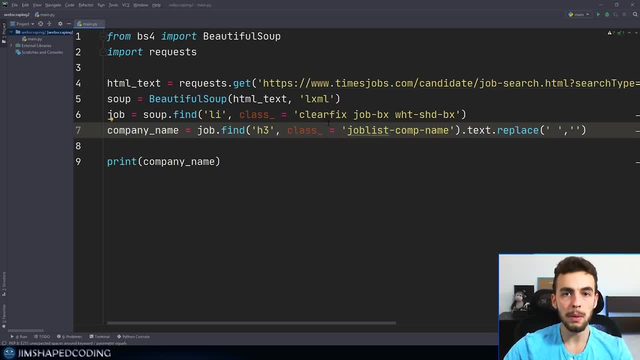 because we know that this job is only for people who are good with the Python programming language. So I'm going to go here And I'm going to repeat myself in the same process Again and I'm going to write here: job dot find And we are probably looking for an element. 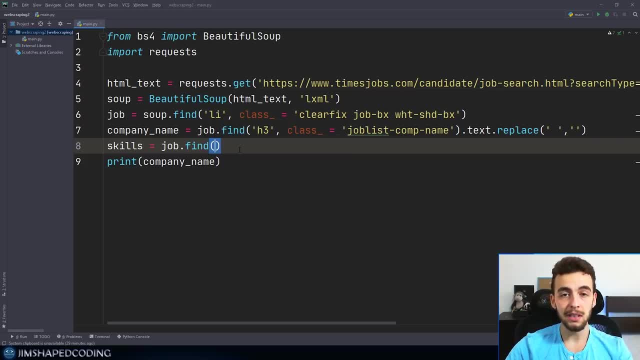 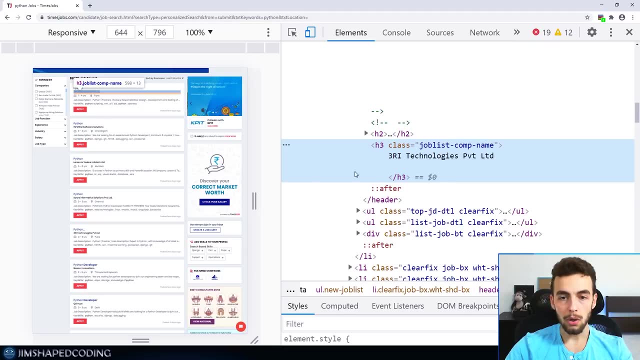 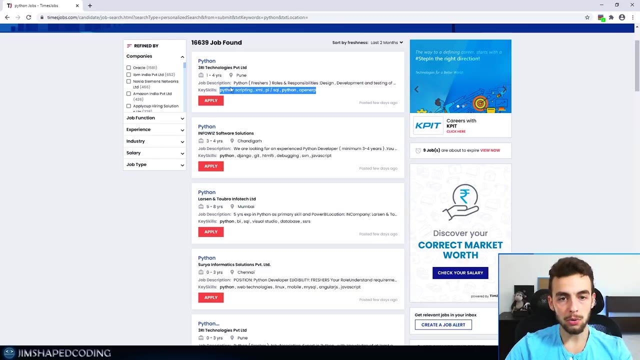 that is including a text about the skill requirements. So let's search for that, Okay. so let's go back to our website again And I'm going to go here and check out what HTML element is including the skills. So we are talking about this one, So I'm going to inspect inside here. 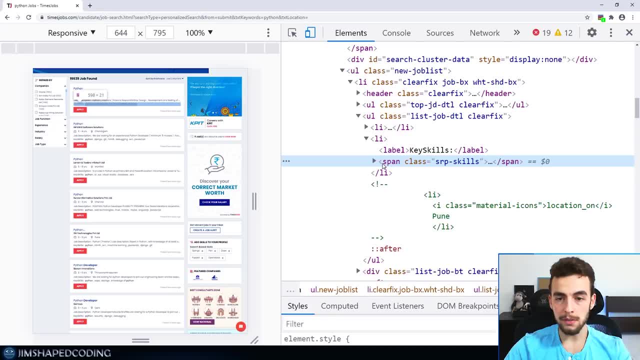 And we can see here that this text is inside a span class with the class name of SRP skills. So I'm going to copy again this class name And that time I'm going to search for the span elements inside my job post. So I'm going to 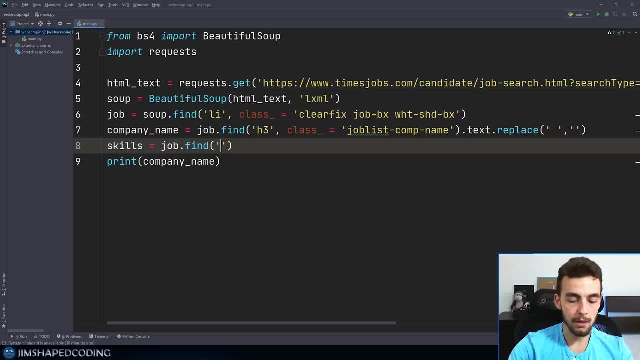 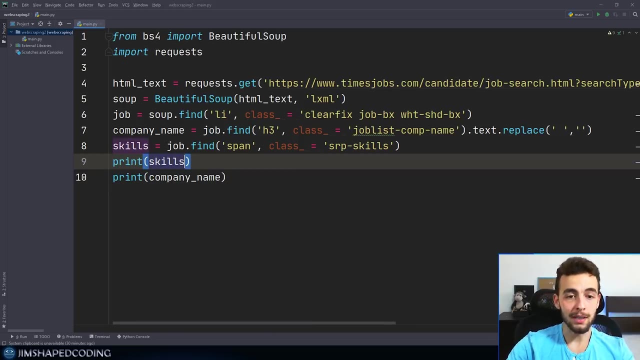 go back to Python again And I'm going to write here span. So this is the HTML tag that we are searching for, And again I'm going to write class underscore equals to that SRP dash skill. Now I want to ensure the results over here Once again. so you always want to quickly. 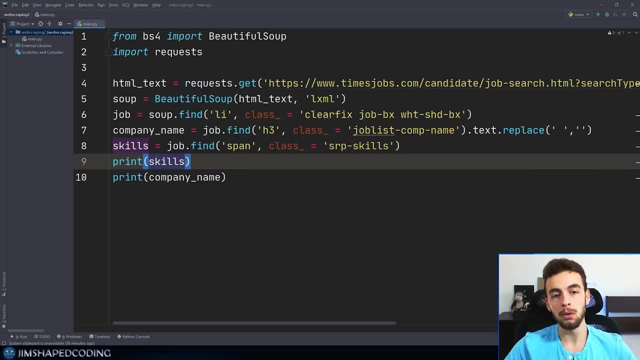 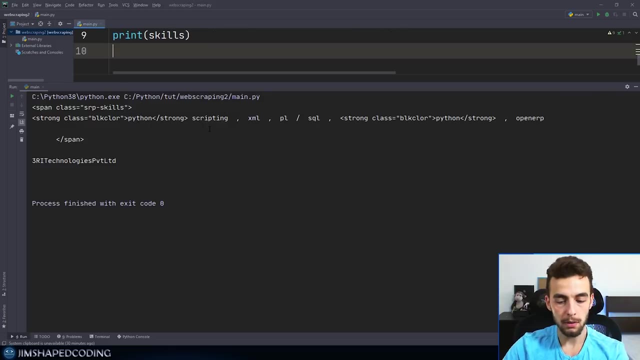 print the results of whatever HTML element that you want to pull to see what other methods you have to apply to prettify your result. Okay, so let's run our program again And it makes sense to delete the print company name. So let's re execute our program And. 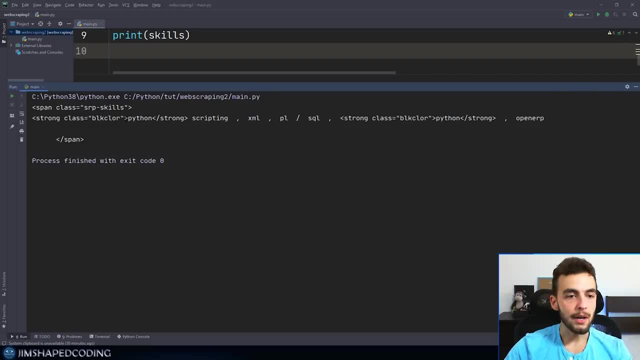 then we have another file as well, And so let's run our program. Let's try again to ouni, pop in, And now we're talking about our sponges And it's working in Python, So let's. And then you can see here that we have some span tag, And then here we have a strong tag. 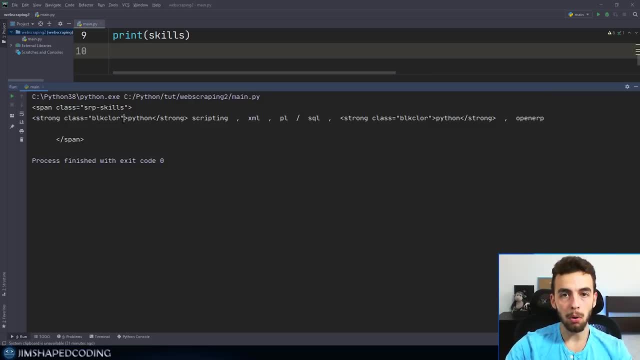 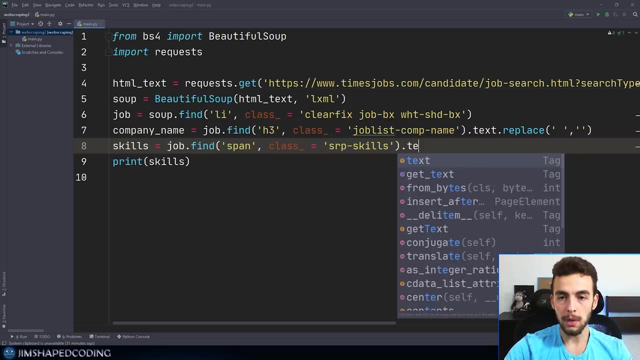 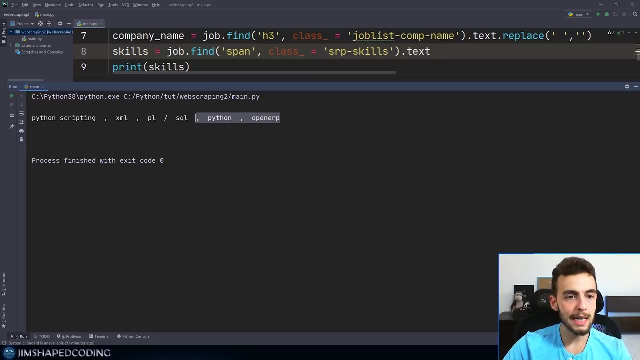 which is basically created to make our text bold when we want to type in something. So I'm just going to guess here that I'm going to only write here dot text and then I expect for the results to be fine. So let's check out for that, And then you can see here that 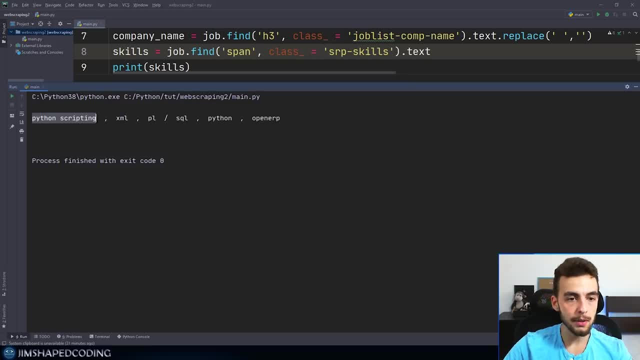 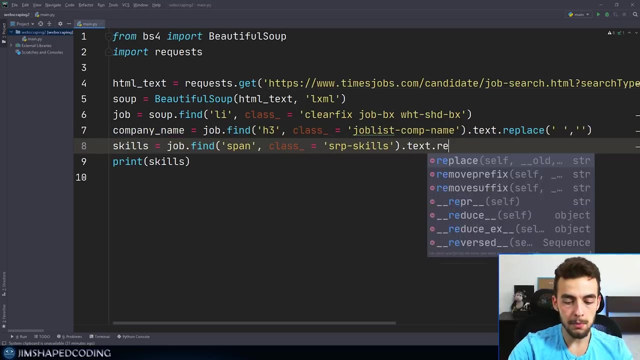 the results are quite great. So we have the Python scripting, And then we have some more requirements that are divided with colors and a lot of white spaces again. So I'm going to apply the same method of that replace once again, like we did with the company name. 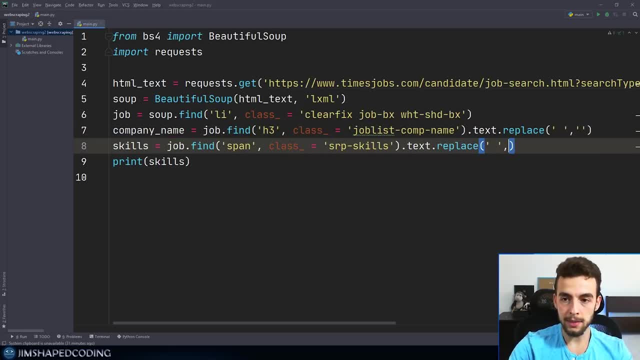 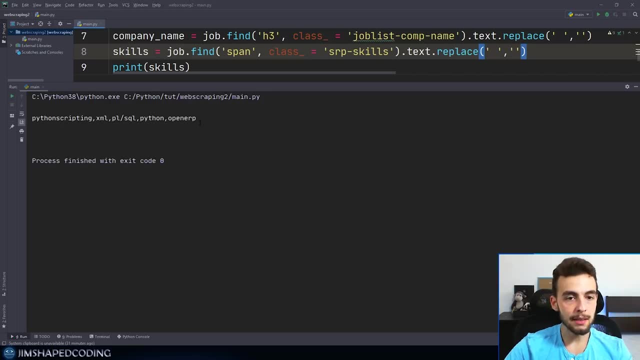 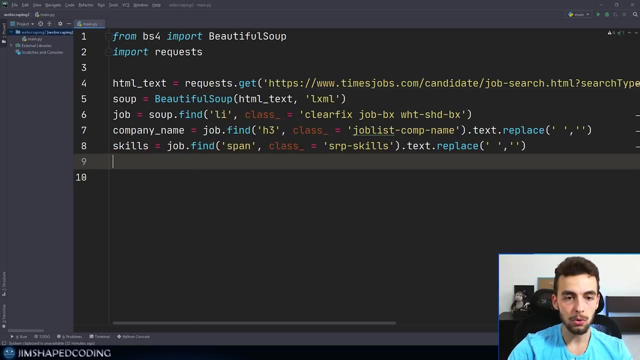 So let's write here that replace- and I'm going to replace- white spaces with nothing. So let's re execute that out, And then we can see that the result is quite like we want. And now we were also able to grab the skills as well. So this is quite nice Now, if we want to. 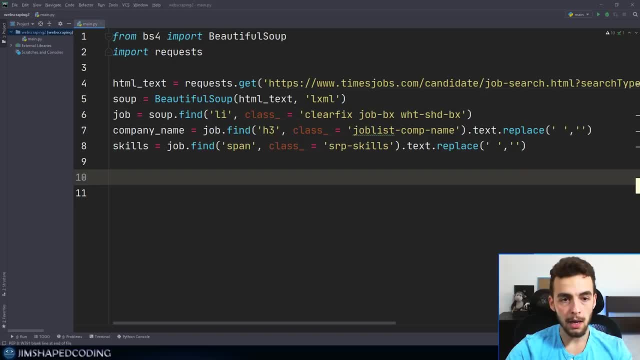 display a nice information about the job until now, then we want to go with a nice print message here. So let's try to create a nice message. So we will use an F method here And we will also use the triple quote method, just to allow us to write some text in separated lines as well. And I'm going 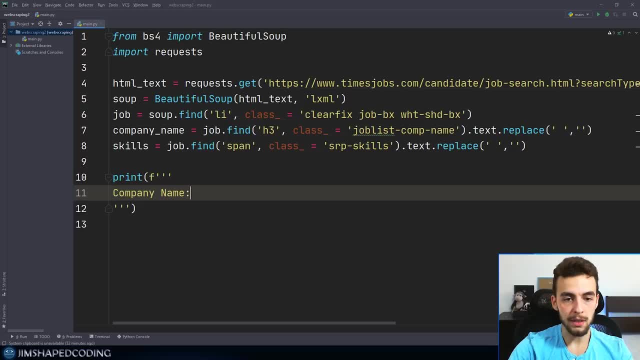 to write here company name like this. And then I'm going to write here company name, So I'm calling the company name value by writing it inside a curly brackets, And I'm going to repeat the same process for required skills. So it will be required skills And then I'm going to make that. 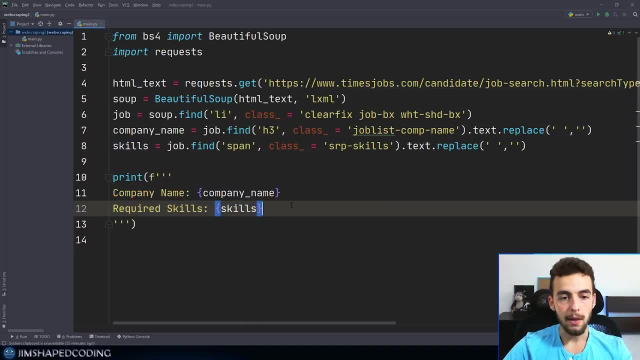 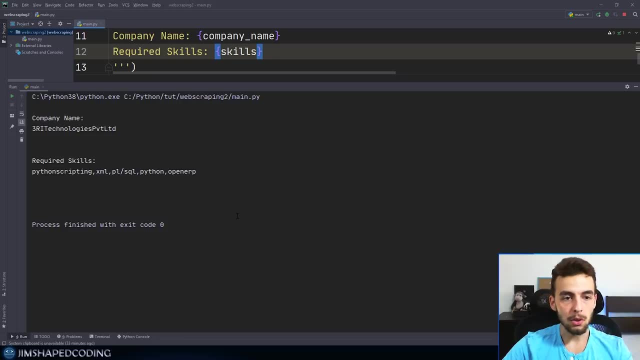 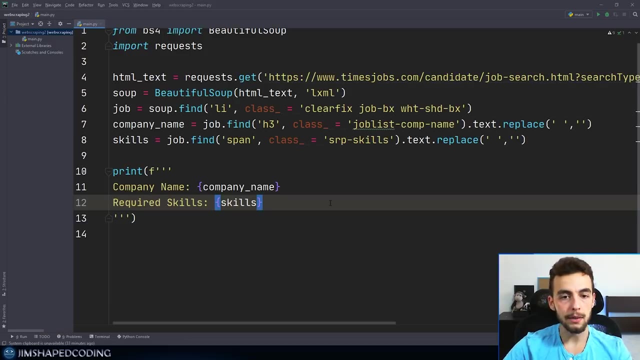 to be equal to skills variable. And now, if I go and execute our program, let's see if the results are quite nice. Yes, so we kind of receiving a nice information about the job, info. Okay, so this is quite great. Now if we go back to here, 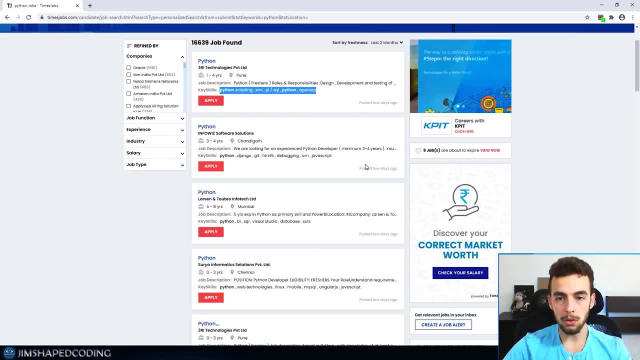 then we want to search for one more element. So you remember that I told you that we only want to grab the job posts with the text of posted few days ago. So we for sure want to write some extra code to apply this functionality. So I'm going to go here. 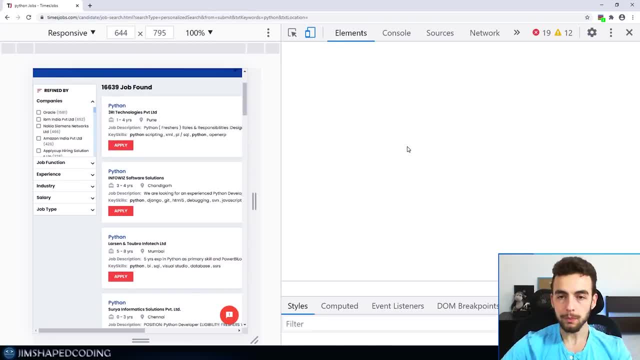 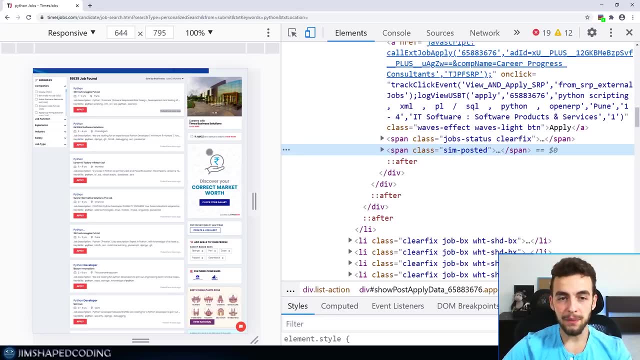 and I'm going to inspect for that element again And then we can see that it is inside a span once again. But I can also see that this job post including some more span tags, so I have to filter out the results again with the class name itself. So I'm going to search for that. 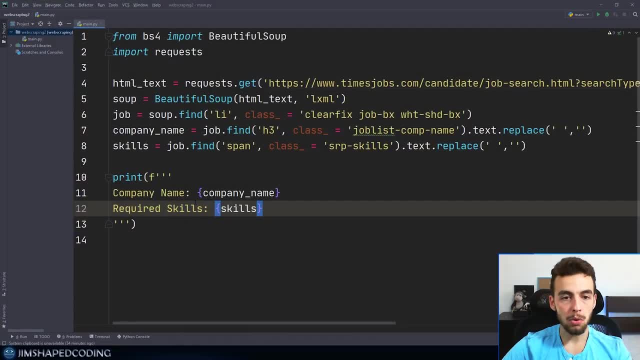 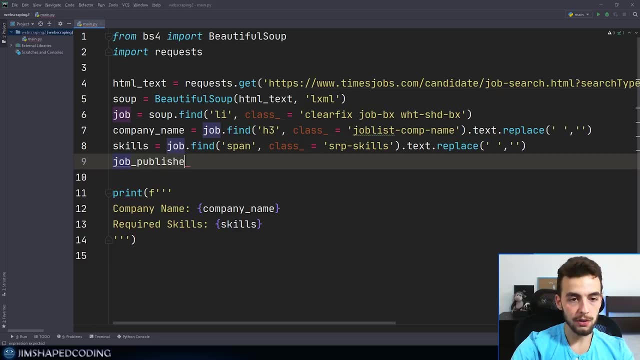 si M posted class name and I'm going to go back to here So we will write this time: job published date. So it makes sense to delete the job, excuse me. so it is just going to be published date And I'm going to go here again with job dot find And we will search for the span And then this: 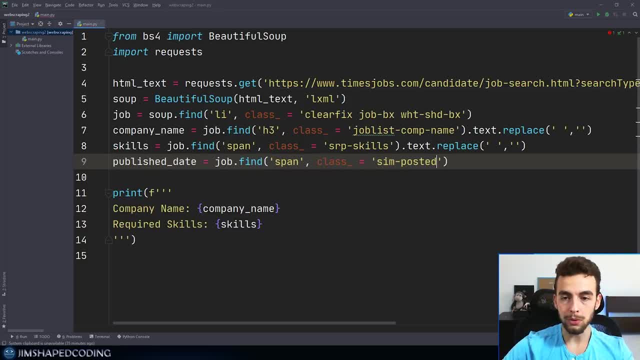 time the class underscore is going to be equal to the text that I just copied And I'm going to repeat myself with printing the published date, But that time let's just avoid printing this print line. So I'm just going to comment out those lines And let's see what the published 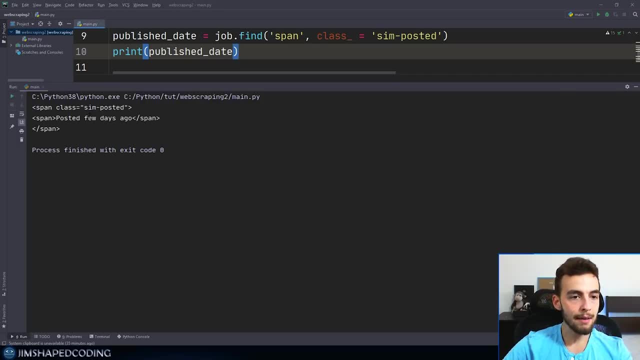 date, date text is looking like And you can see that we have here something a little bit weird. So we have the span here And we have also one more span inside of the text of it. So what means? it means that we have to take some different action than what we did previously. So this time, 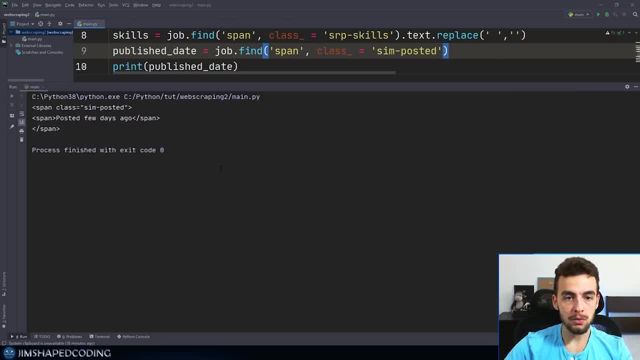 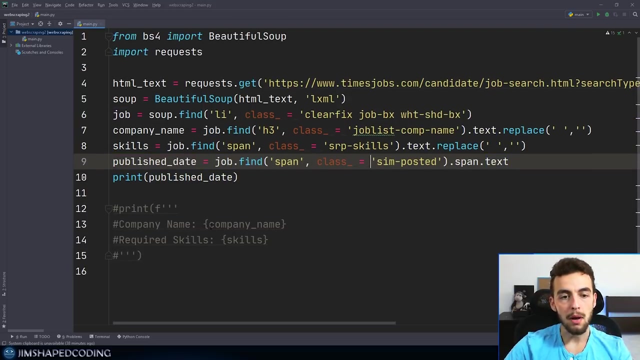 I want to search for the attribute of span just to get inside that tag over here, And then right after it I want to look for the text of that span tag. So this will give me the published date of this specific job, But I'm not going to include the published date inside my print message. 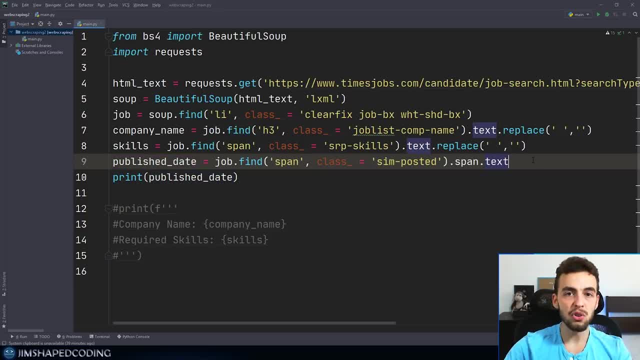 because we only want the published date for this specific job. But I'm not going to include the published date inside my print message because we only want the published date for this specific job, date for the functionality to stop our execution if the published date text is not including the. 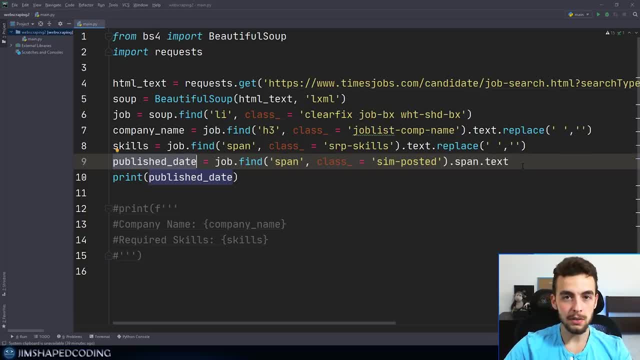 word of few, and I'm going to code this functionality just in a second, So you will see what I mean by what I said. Alright, so what I'm going to do here is take a tricky action that is going to bring me all the jobs from the first page. So if we paid attention, then all the 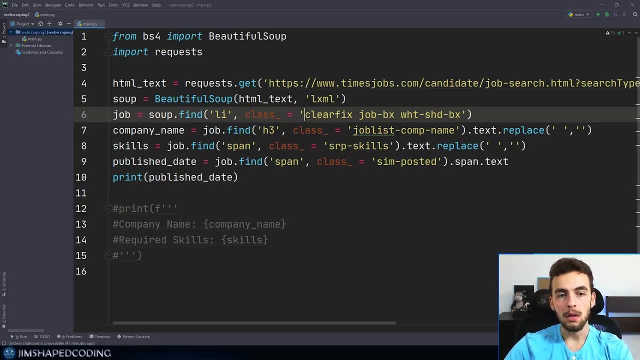 job posts including this class name. and then, let's say, I added a little bit more, more variable here, which is the value of the content that we're going to use is going to be the job post. So what I can do besides the find, 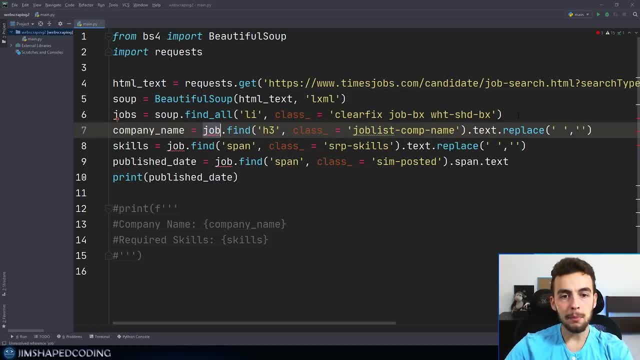 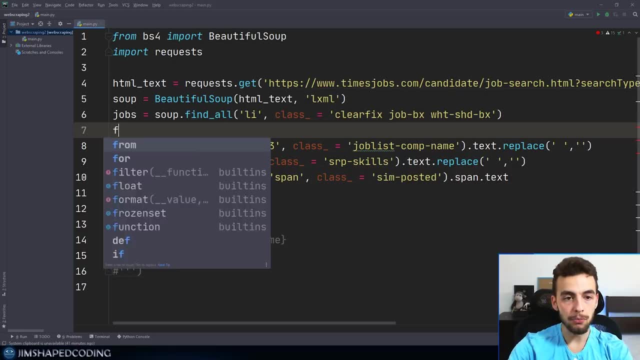 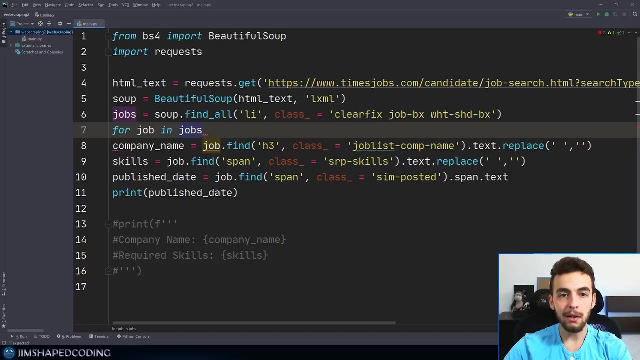 is: change that back to underscore all and change this variable name to jobs. And I know that just now it just raised an arrow here And I'm going to use here a for loop that is going to iterate over each element And I'm going to write here for job in jobs, and then I'm going to create an indentation. 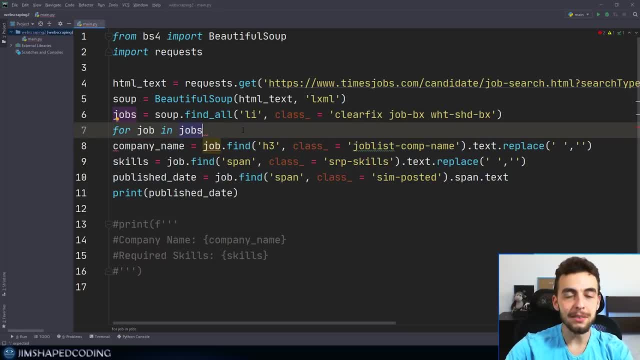 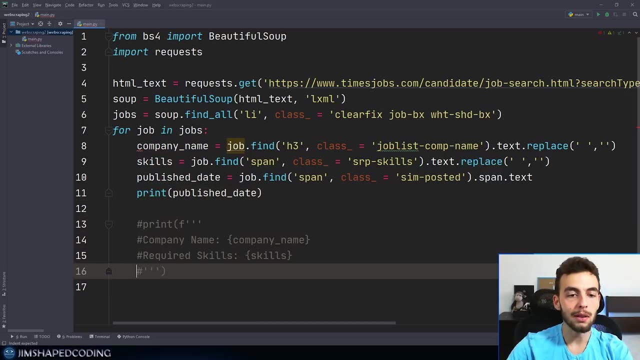 right there. So the results will be applied for all the jobs that are posted in the first page of the web page that we scrape. So once I hit here the colon sign, then I'm going to create an indentation for each of our lines like this, And then the results are going to be quite the same. So let's. 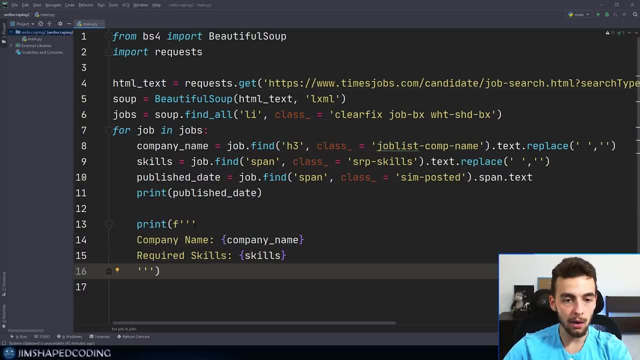 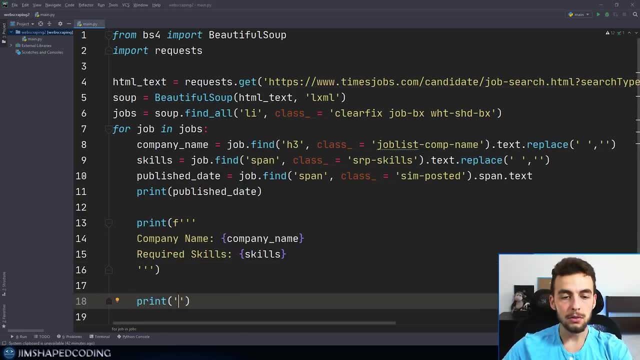 test that out. Okay, I'm going to uncomment our print line over here And just for comfort reasons, I'm also going to print here and empty lines, So we can kind of see a division between the different jobs, And then I'm going to delete the published date for now. So if we execute our program, that 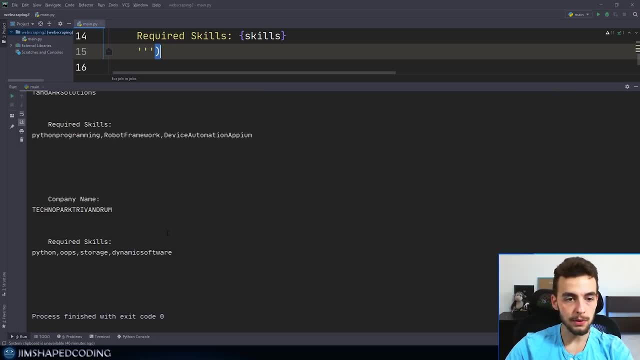 time, then we are going to see a nicer results, And this is going to contain all the job posts from the page that we scrape Again, so you can see that we have a nice paragraph for that job post And then we have also another. 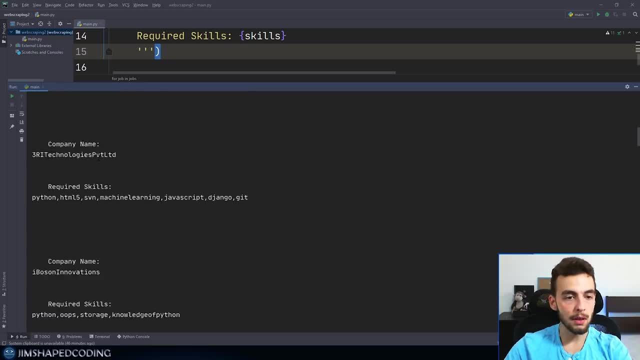 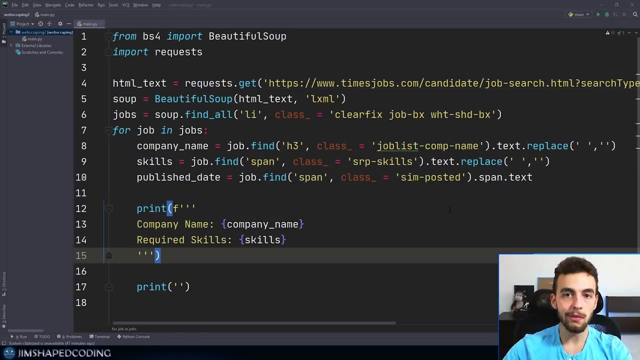 one here, And if I keep scrolling up, we can see a lot of them in that output. So this is quite great. So, if you remember, we wanted to filter out the job posts that are not including the word of few inside the published date, Because what that means? it means that this job could be. 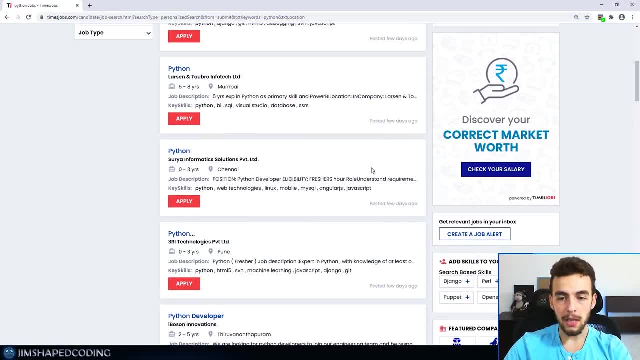 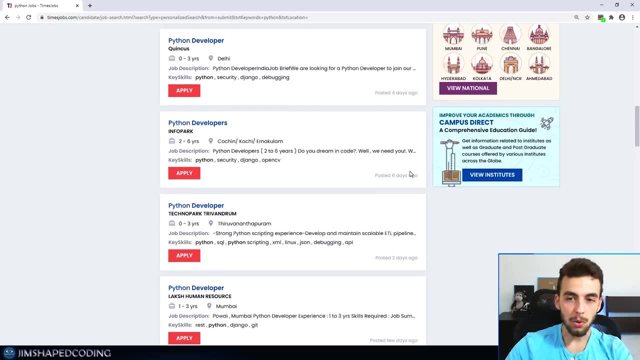 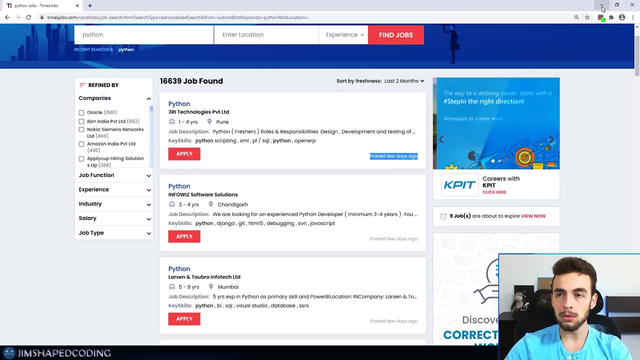 outdated. So if I go to our page again, then we can see that as I keep scrolling down, we have some text like posted six days ago, And I wanted to filter out only the jobs that are containing the text of posted few days ago. So in order to apply this, I'm going to change the orders here a little. 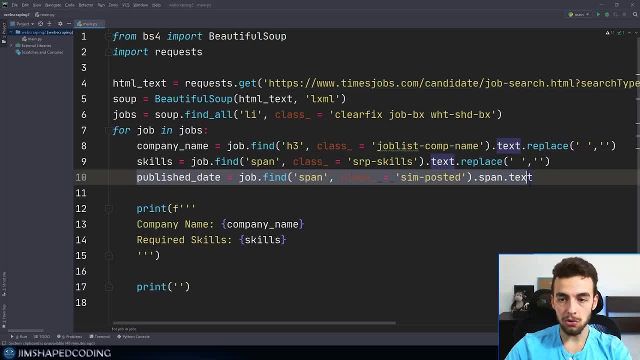 bit Okay. so I'm going to cut this searching here And I'm going to paste that in as the first line inside my first line. So I'm going to paste that in as the first line inside my first line And I'm. 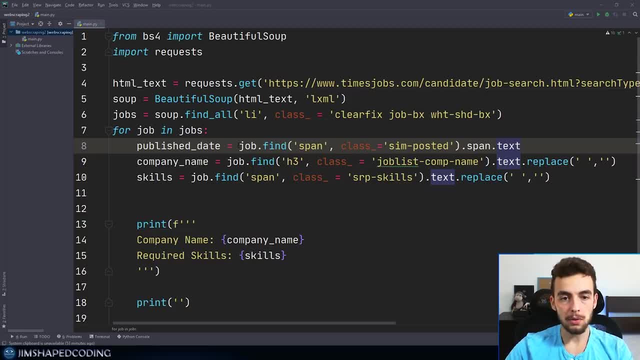 going to run what. let me время check of what got in for loop. Now, the reason I'm doing this: it is basically because I don't want to continue on scraping for that post if the publish date is not matching my condition. So it makes a lot of sense to play this code as the first line inside. 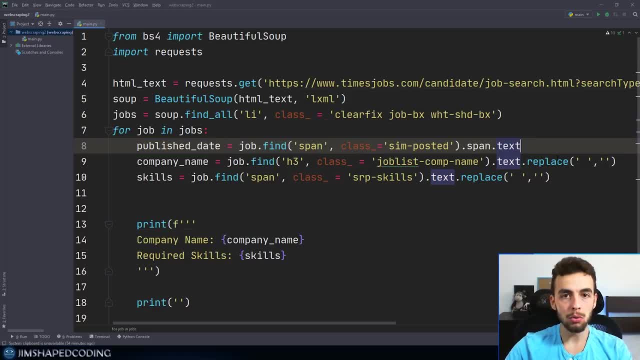 my fourth loop. And then right here I'm going to write a condition that is going to check if the word of Phil find enough ads without the condition in a form you can hold possible census. If so, I will send this survey Next day. I will close the dareBut before that sometimes I 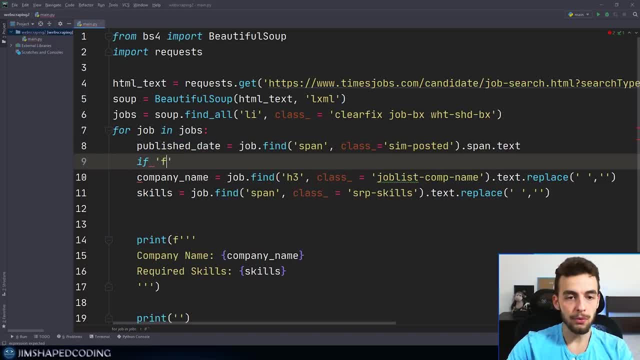 accidentally click the bar here. if the number or number of me, like our, get chance to place my を will slow down the text. So it is browsed very well, way and moment by way of time. so it makes a lot of sure. So it will be if few in published date. 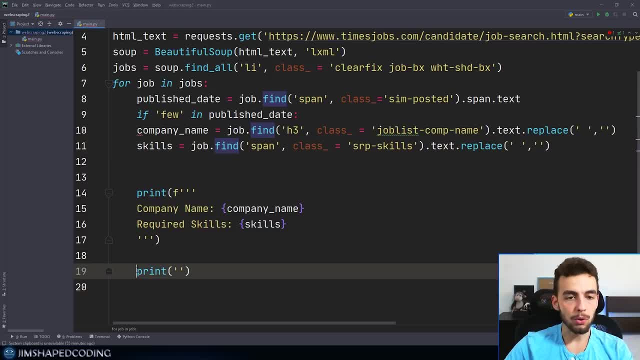 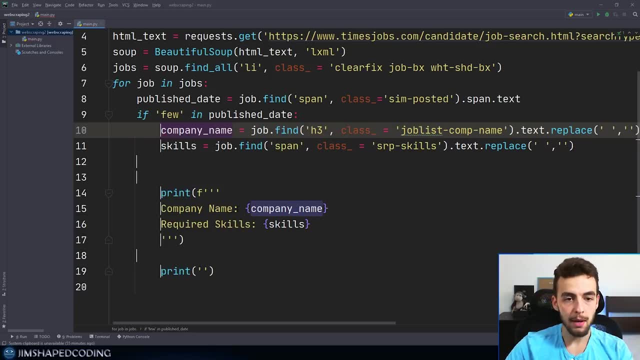 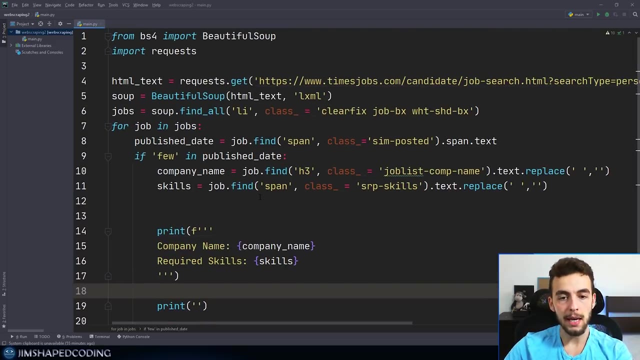 and again, I'm going to create an indentation for the entire code here, So you can do that with the shift, alt combined and then you can just press tab and all the lines here are being indented. So right now, if I go ahead and execute our program, 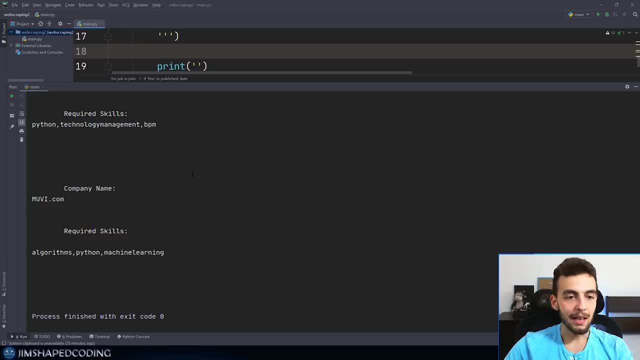 then we should see the results again, like almost the same. but we also see here that the F string is not quite nice. but I can live with that, Okay. so it is great that we were able to receive the posts only that have been published few days ago. 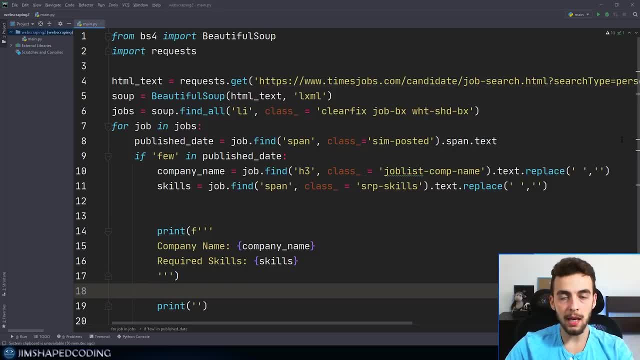 Now there is no limit for what you can do when it comes to web scraping and what you can filter in or filter out, But basically this program deals with how to how to grab some job posts with the filters that you want to apply that maybe sometimes may not be available. 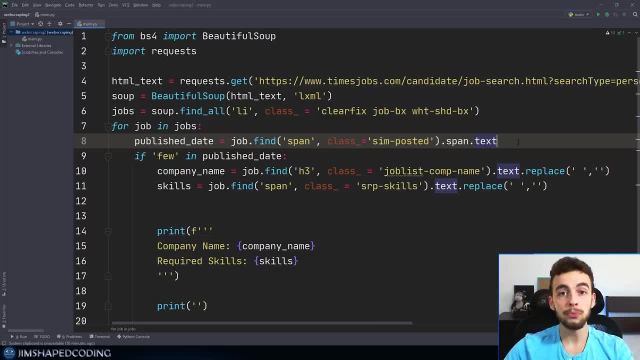 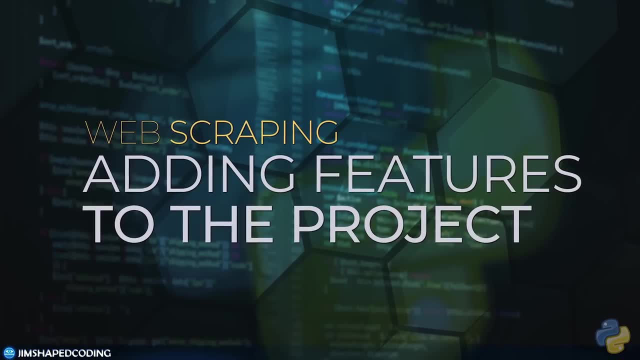 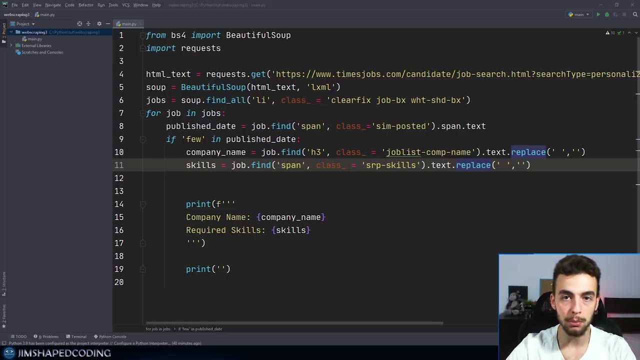 from the website itself, So you can write your own filtrations on your Python code while you scrape some information from a specific website. So I'm going to do whatever it takes to turn this program into a very useful one, And I'm going to do that. 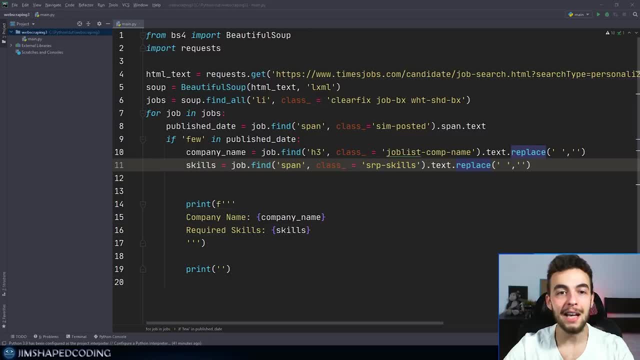 by applying some special functionalities, such as wrapping this entire program in a while loop and executing this project every certain amount of time, and also apply some filtrations to filter out the job posts that are not meeting the skills that I own, And also I'm going to throw the results. 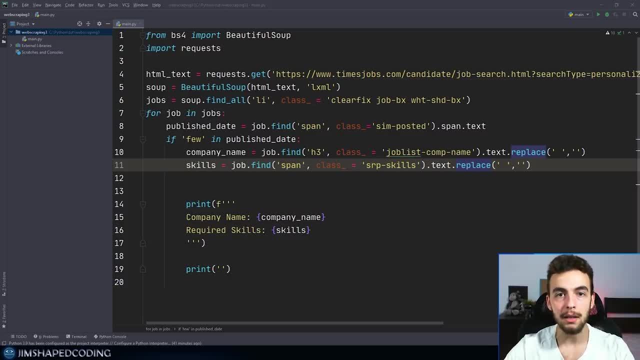 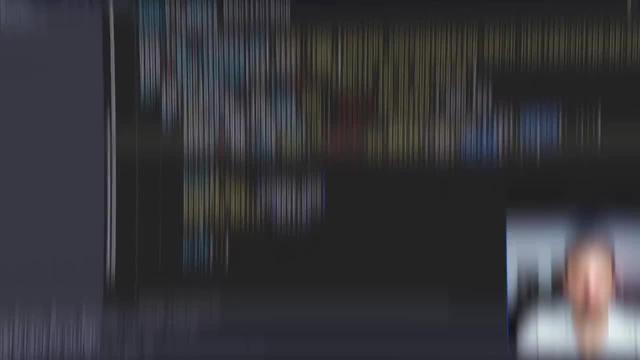 of the different job posts into a new blank file, So I can be aware of the posts that are being posted every certain amount of time. So let's get started, All right then. So let's start with a kind reminder of the results that we got until that point. 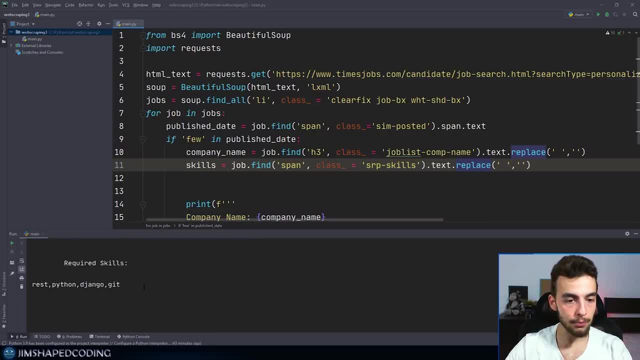 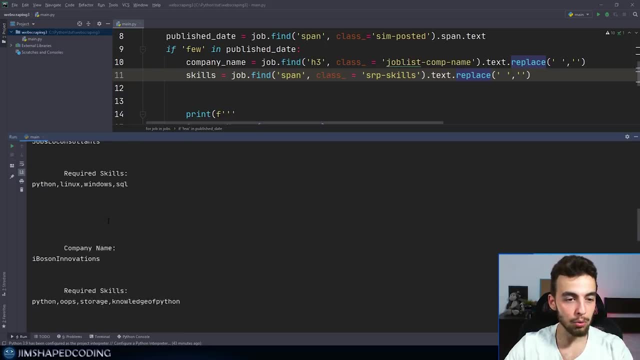 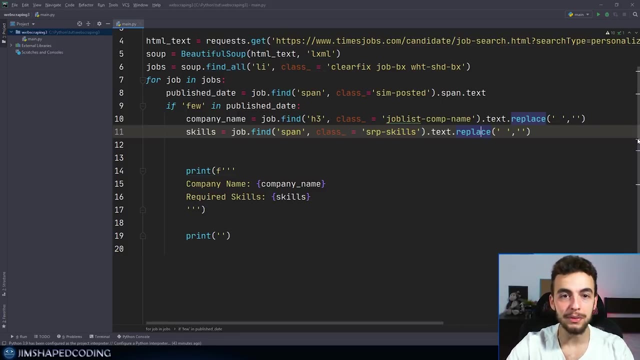 So we run our program now and if we show it right here, you can see that those lines are not aligned well. So I'm going to change that And I'm also going to provide some extra information that will show us the exact link of the specific job. 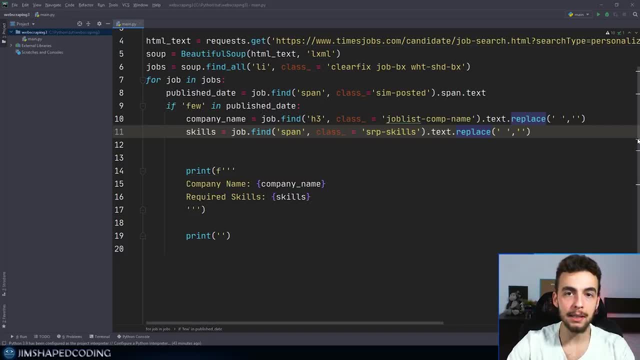 that we are iterating on. So that way I will have the ability to just click on the link and then see more information about that job. So as a beginner, I will get rid of the formatted string in that case, because doing a formatted string with a triple code? 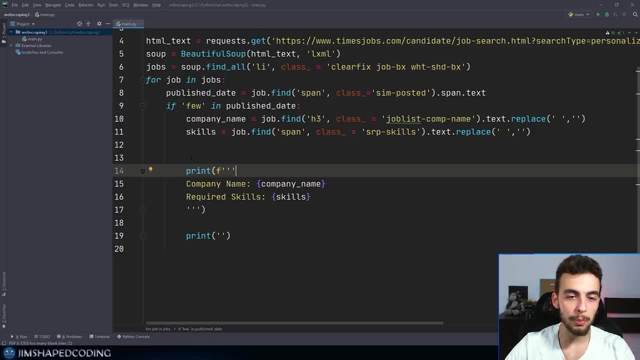 might not be a great idea when you execute it with a for loop because, as you can see, that it also includes the indentations right here. So I'm going to delete this entire code here and I'm going to write two more new formatted strings. 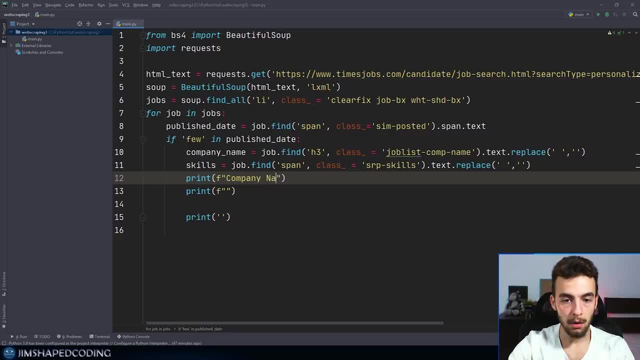 And we will start with company name. make that to be equal to company name. So make sure to add a column here so it will be more friendly, And then I will write here required skills as well, And then we will write here the skills variable. 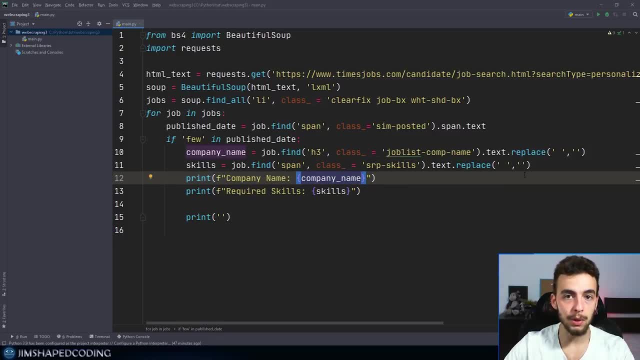 Now there was one more issue with the result that we showed a minute ago, and that was the blank spaces that are being shown as well. So we can get rid of the spaces by a special method That is called strip, And it is a special method that you are allowed. 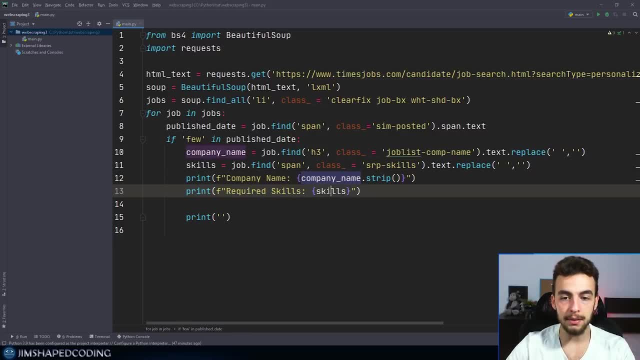 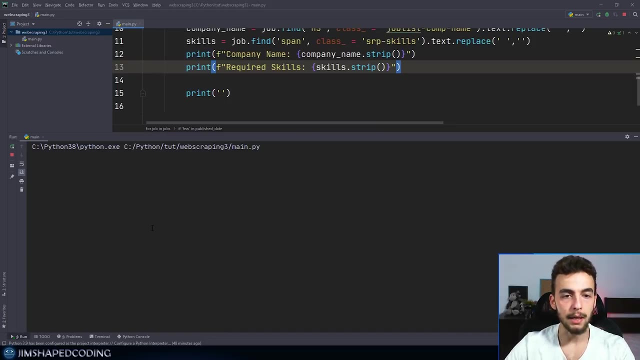 to use inside the strings, And since the company name and the skills are strings by default, I don't have to convert them to a string, So I can just call that method like this. okay, And now I will show the results of something like the following: 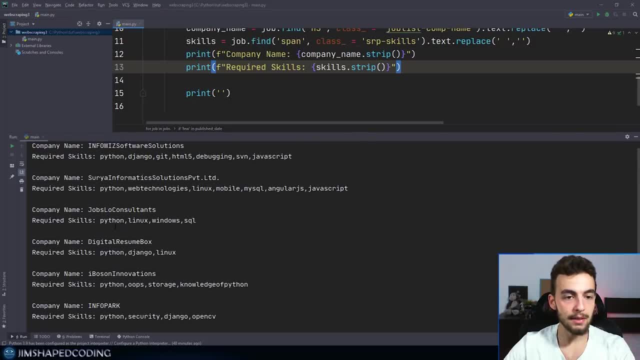 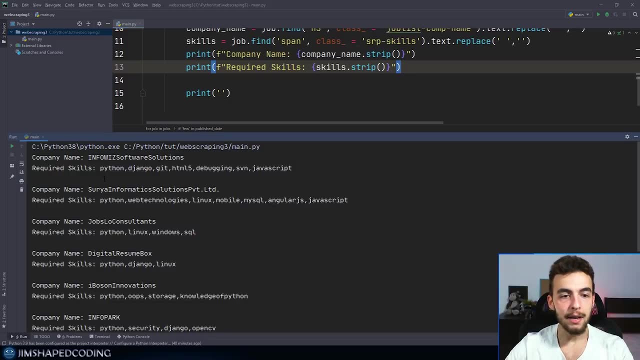 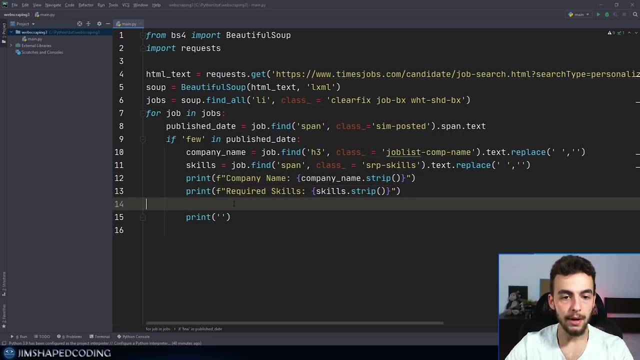 And in a few seconds we will see that this is aligned way better than what it was. I'm going to add here more information line that will show the link of the job post, So let's do that. Okay, let's go here and write this functionality. 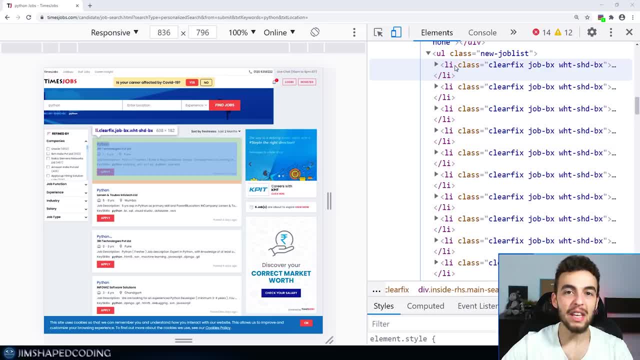 Okay, so we had a unordered list that inside of that we had some different HTML tags that are called LI and that stands for lists, And they are actually different job posts that are divided into different elements inside an unordered list. And then, if we hover our mouse, 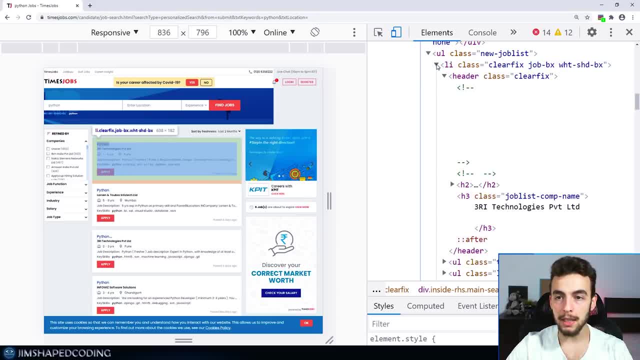 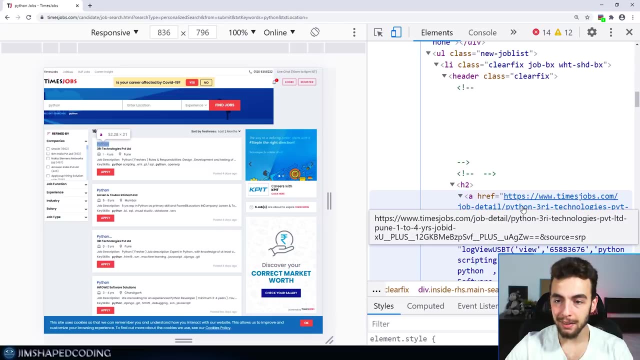 you can see that there are different jobs. Now, if I go inside one of them and I go inside a header tag, that is actually the first header of the LI tag, And then I will go inside the H2 here And then you can see that we have a link. 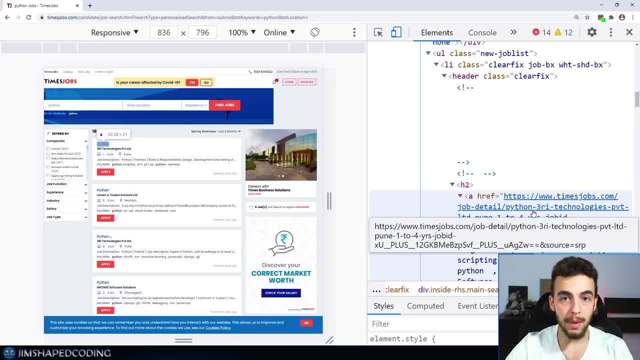 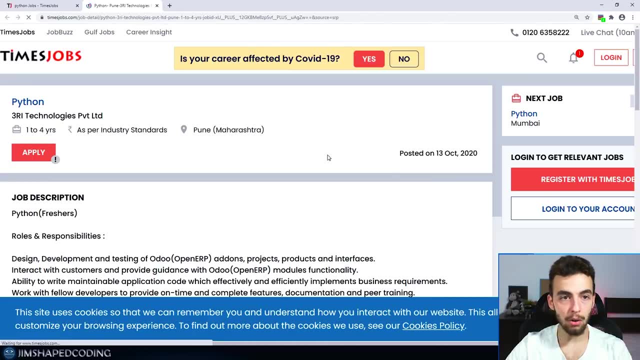 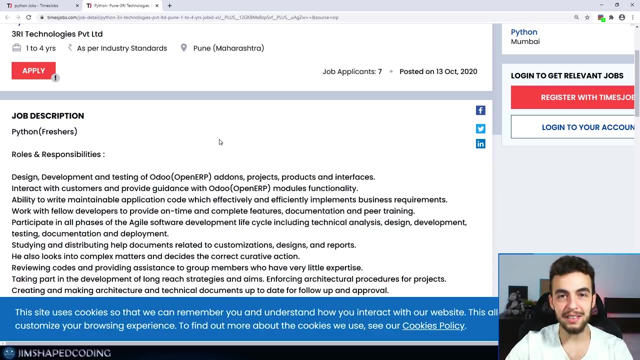 that could lead us to a link that provides some extra information about that specific job. So if I actually go here and click on here, you can see that we receive the job description right here. So what we have to do in order to access this link. 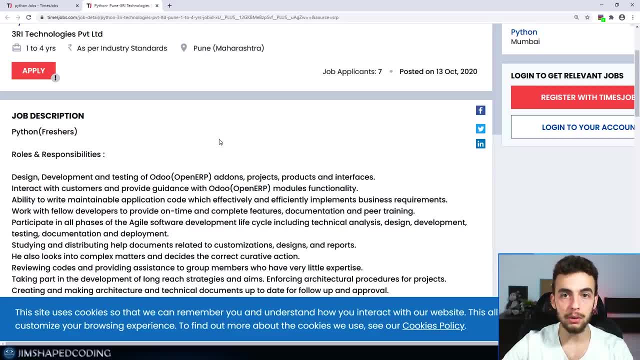 in each job post that we are iterating on. the Python code is actually going inside and header and then going inside one more tag with a kind of H2, as you saw me doing that, and then access that A tag. So let's do that. 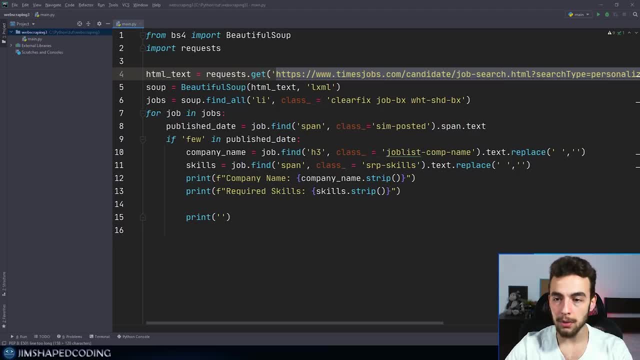 Okay, I'm going to go back to PyCharm and apply this functionality, So we will go under the skills and then we will write here more info And that will be equal to jobheader, because this was the first tag that we want to go inside of it. 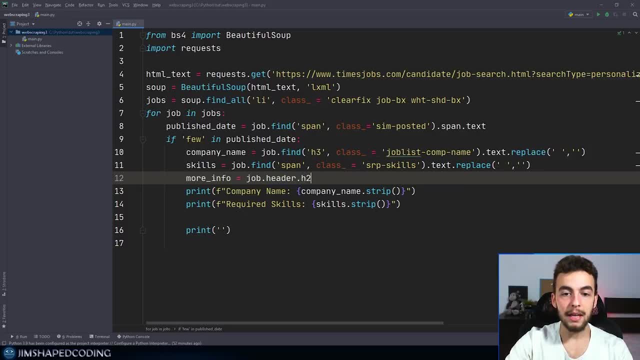 And then we want to go inside the H2.. And then, inside that H2, we want to go inside the A tag. Now, before we go further, let's test ourselves that we have done a great job. So let's print the. 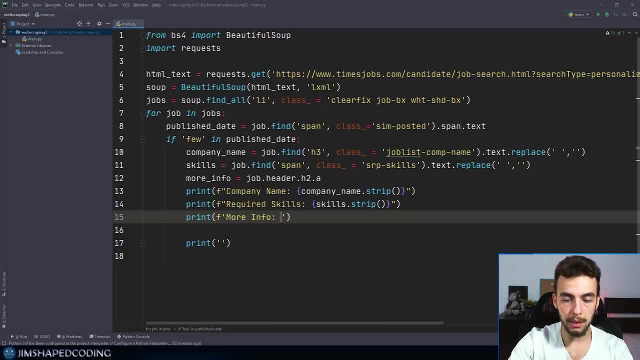 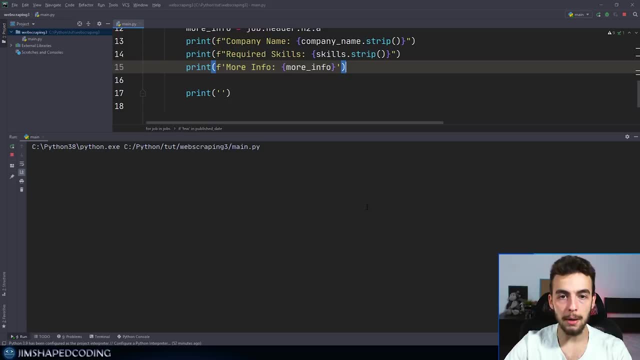 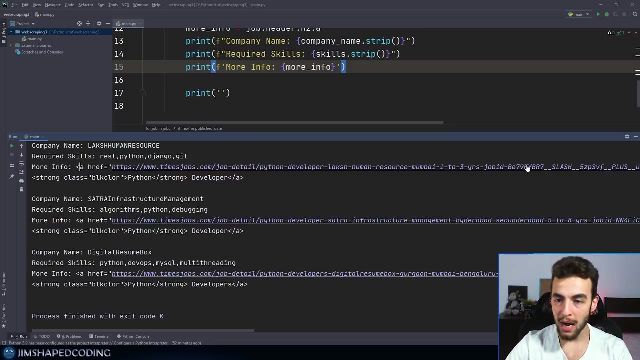 the more info in the following way: So it will be more info and then we will call the variable in a formatted string. Now let's execute our program And then you can see that inside the more info we have the Ahref. 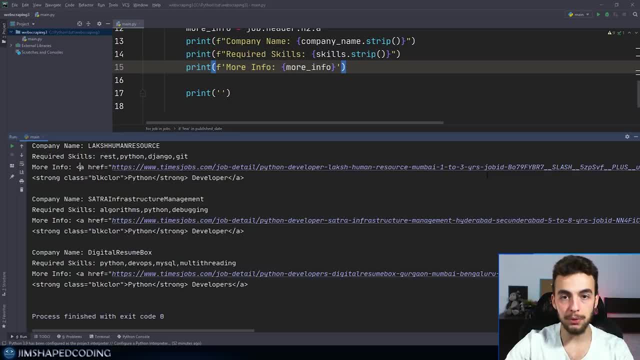 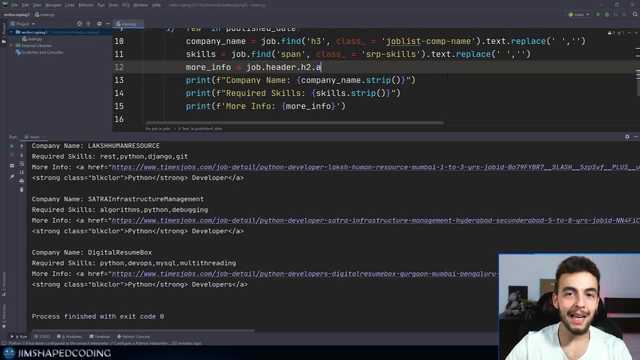 which gives us the link about the specific job that we are iterating on. So all I have to do here is going back to my more info and then call that Ahref, and then I'm going to do that with a square bracket, like in dictionaries. 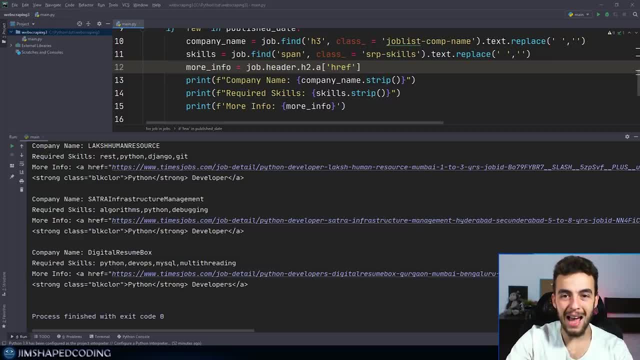 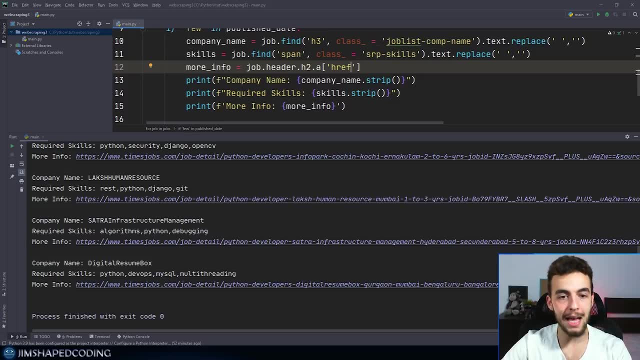 And then I'm going to write here Ahref, so I will receive the value of that attribute. So if I run that one more time, then I should see the link only, And that is what exactly happening. So the result is quite great. 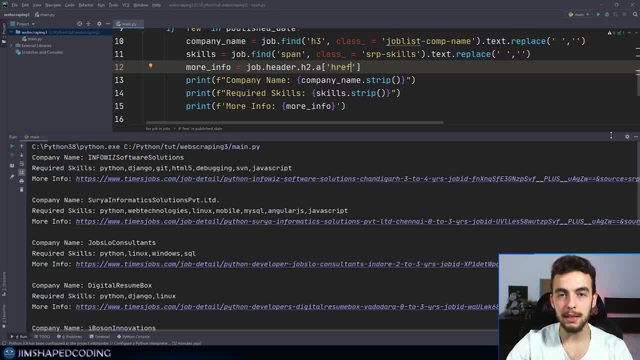 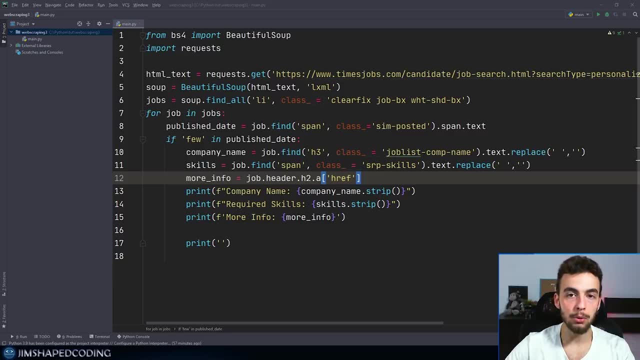 And then you can see that this is already better than what we did in the last episode, And we will continue from here. Okay, so what I want to do now is giving the operation opportunity for the user that executes this program to filter out some skill requirement that he does not own. 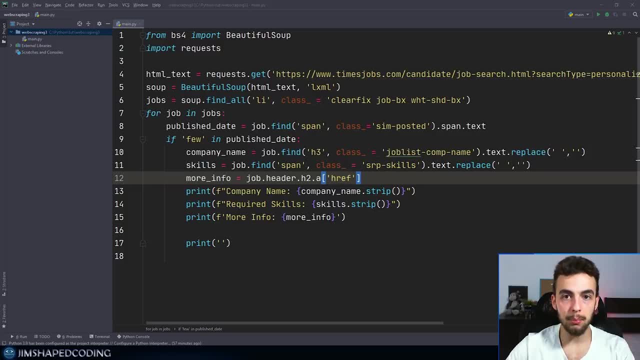 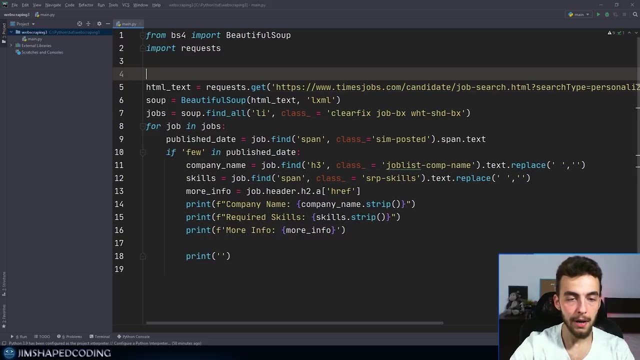 So we will use the input function for that, And then, whatever the input is equal to, we will filter out the results from the jobs that we are finding right here. Okay, so let's write this functionality. So, to apply this, I'm going to create a new variable over here. 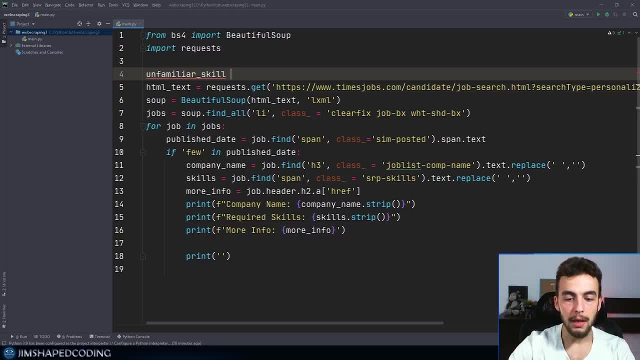 and I'm going to call it unfamiliar skill, And I'm going to make that to be equal to an input, And then I'm going to write here something like this: Okay, so the user could understand that he has to provide some information in order to execute this program. 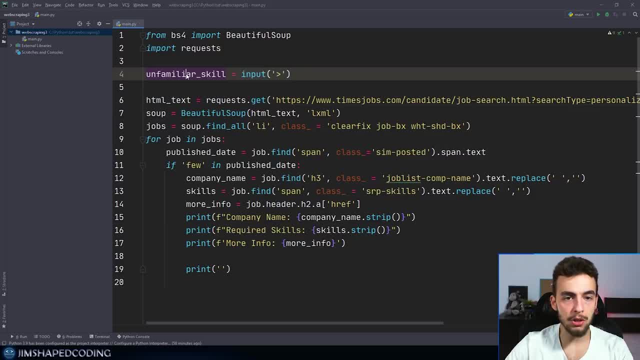 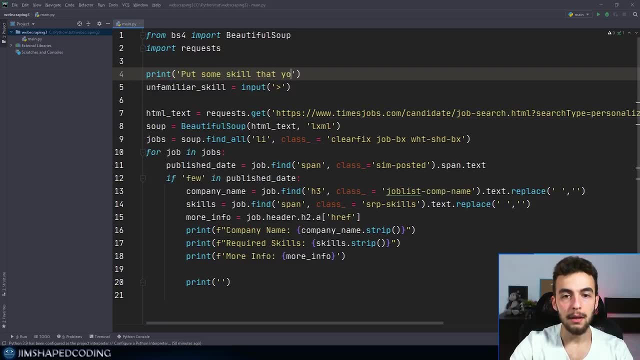 And actually it might be a great idea to print some extra information before that input function. So it will be: print, put some skill that you are not familiar with And then, right after the unfamiliar skill input, I will write here filtering out. 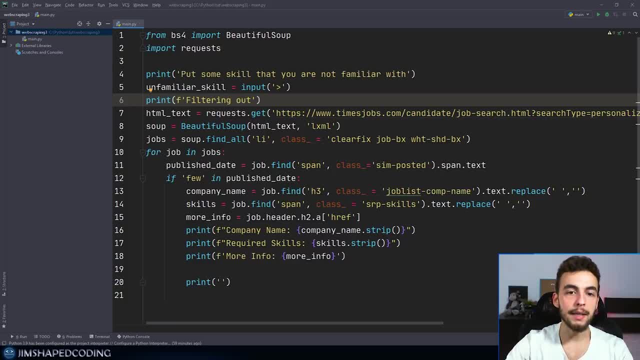 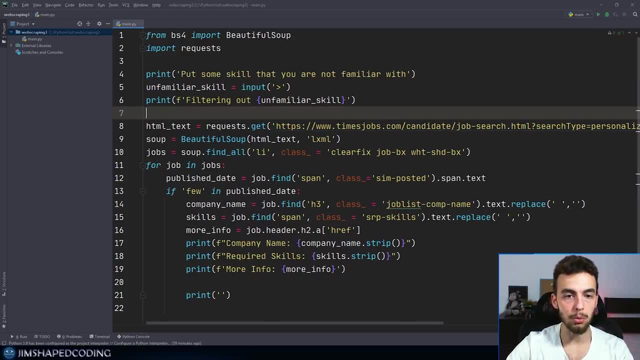 and we will actually make that a formatted string, And then we will write here filtering out, and then whatever the unfamiliar skill is equal to. Now what are we going to do with this unfamiliar skill variable? So that is quite easy, right? 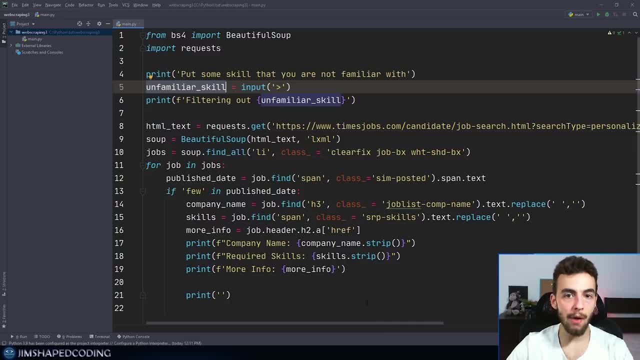 We have to search for a condition that will filter out the job post that is included, including that word that we are going to provide here as an unfamiliar skill, And what we can actually do is search for the unfamiliar skill word inside the skills string. 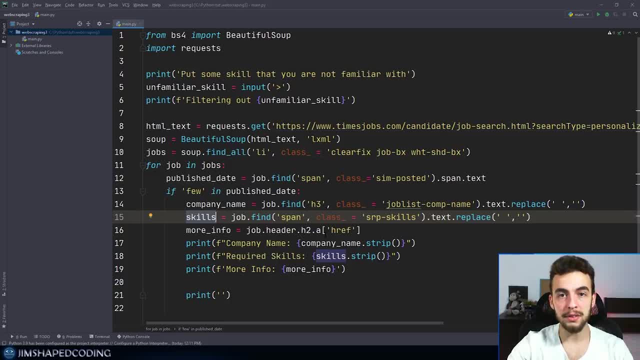 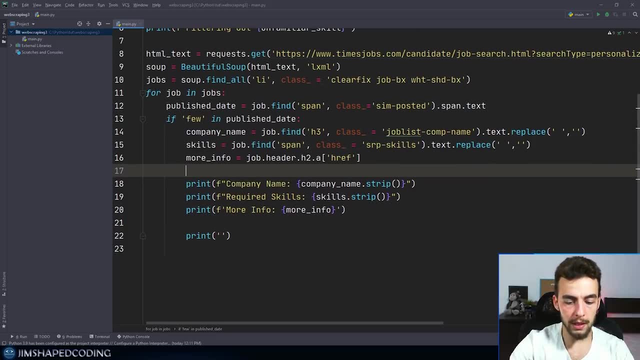 So, if you remember, the skills is a long string that is divided with commas. So we can go with a condition like the following: So it will be, if unfamiliar skill not inside the skills that we are grabbing in the each job post that we are iterating. 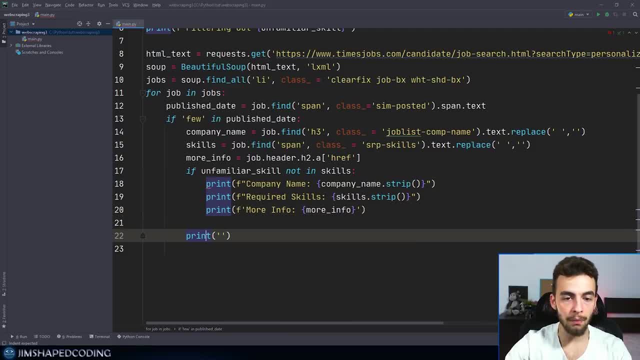 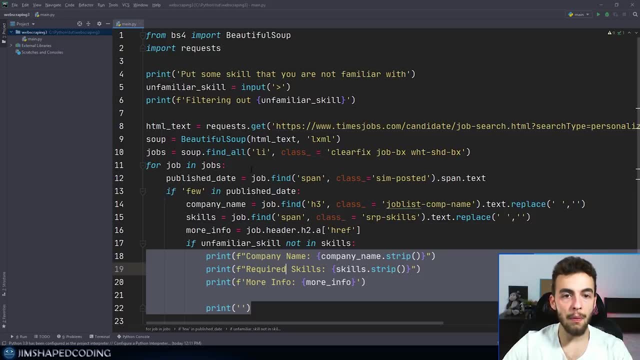 And now all what we have to do here is creating the indentation for the different print lines. Okay, so now I should see the job posts that are not including the unfamiliar skill that I'm going to provide. So just to test that out, let's run our program twice. 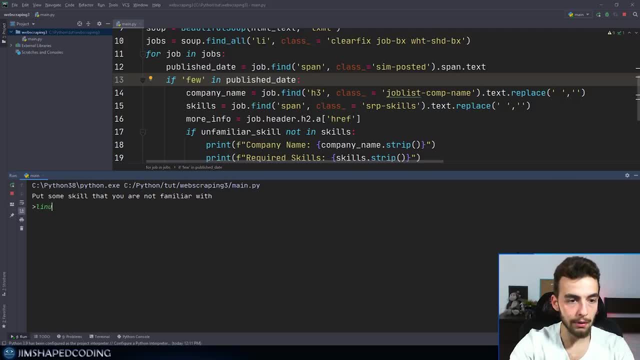 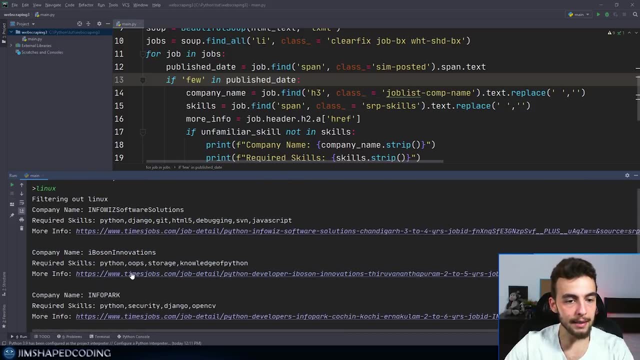 Okay, so in the first we are going to write here Linux as a skill that I'm not familiar with, And you can see that we don't see anything that is including the keyword of Linux over here. But let's actually take that to a next level. 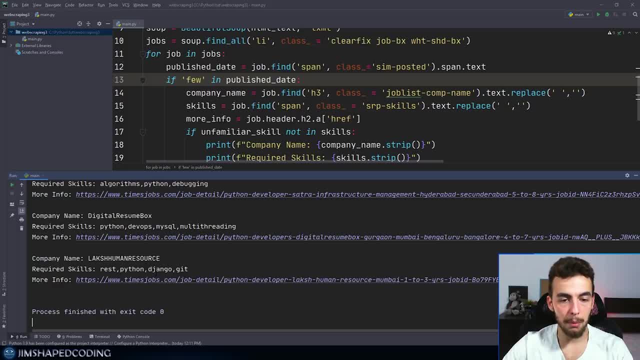 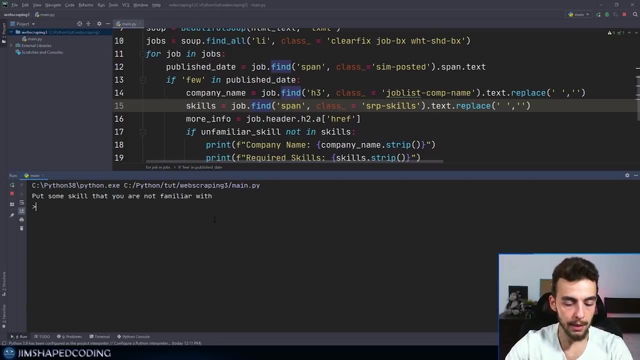 and test that out. So we see here a specific job post that is including Django. So let's say that I am not familiar with Django and see next time if I see that job post with this company name. So let's re execute our program. 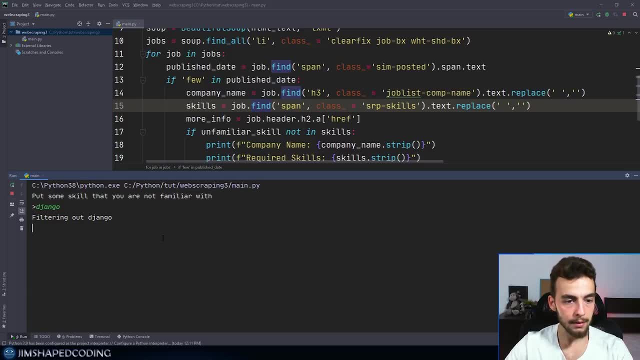 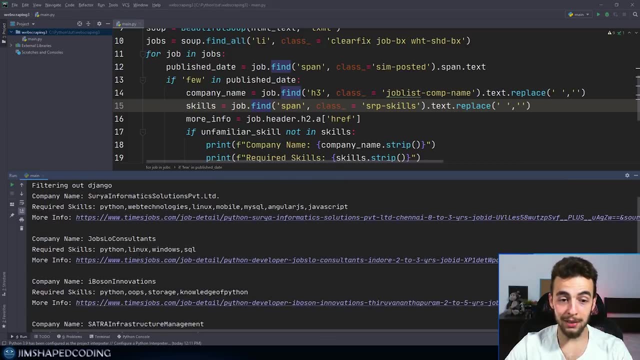 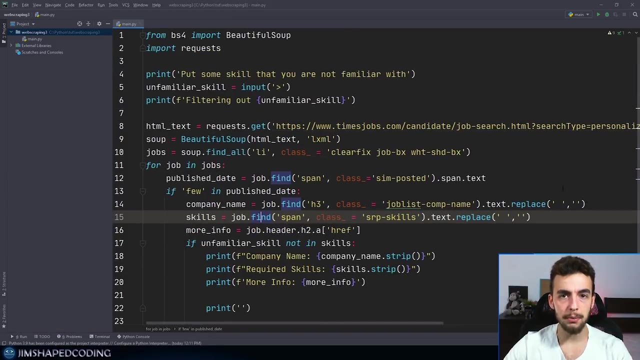 and that time I will write Django and let's see the results. So we can see that we don't have any job with Django, but we do have Linux that time. So this condition works well and we will continue on to next step from here. 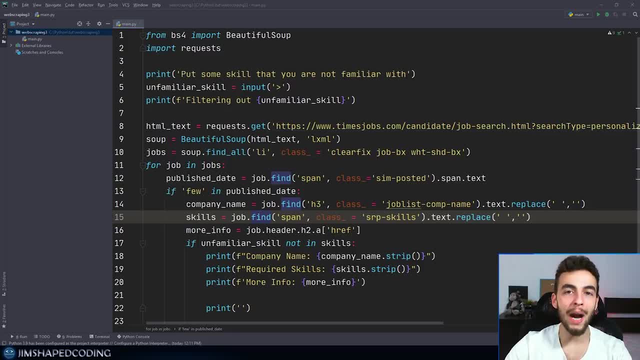 Now what could be an exciting challenge for you guys is to write an algorithm that will accept more than one. unfamiliar skills. So you want to accept multiple inputs from a user, and it might be more challenging, but I think you should try to spend some time. 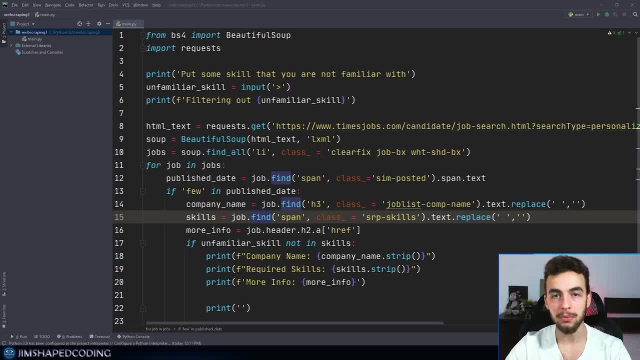 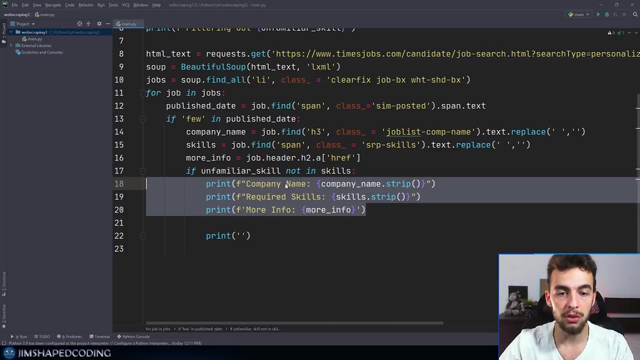 on something like this because I think this could be an amazing challenge for everyone who is watching this video. All right, so now we are going to save each job post in a different file, So besides printing this in the terminal, then we are going to write this entire information. 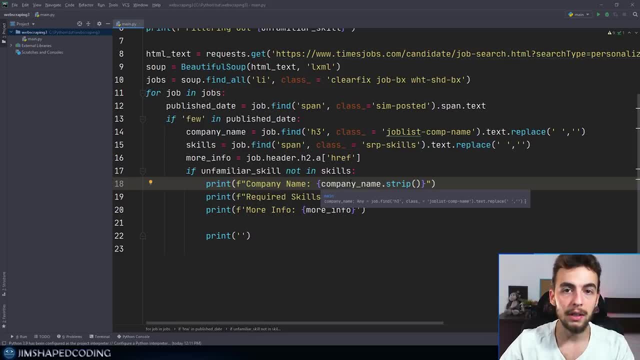 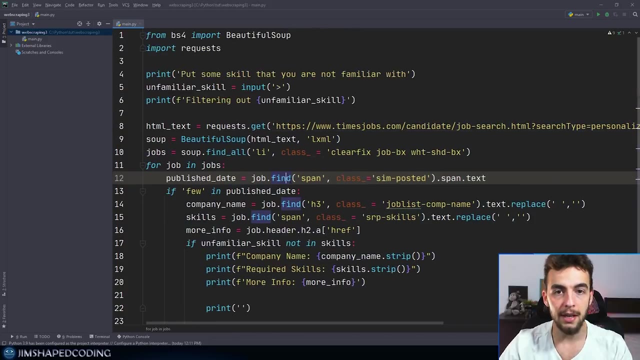 in a separated file, And then I will also allow this program to run every 15 minutes, or every 10 minutes, Up to you, And I will show this logic as well. So, first of first, it makes sense to wrap our entire program in a function. 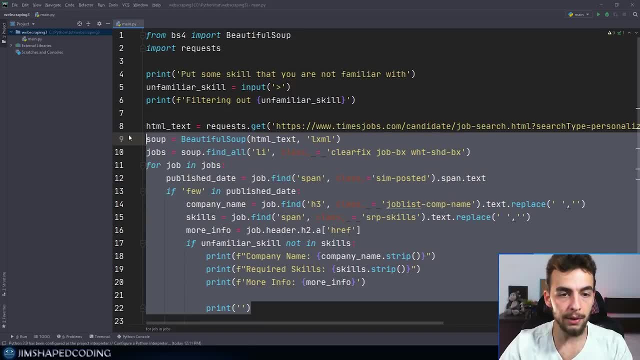 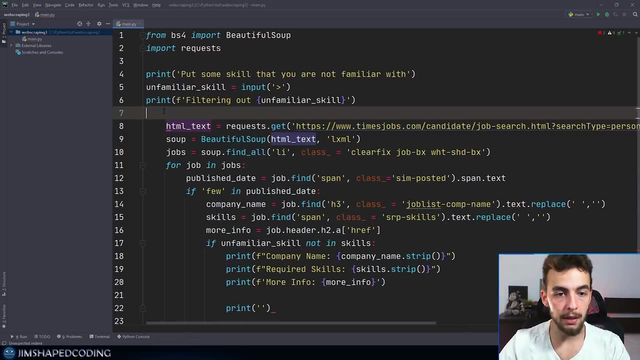 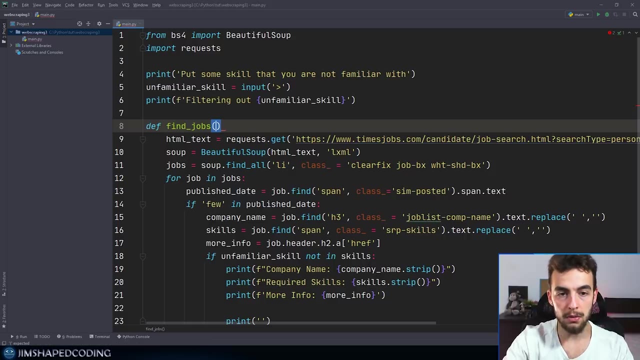 And I'm going to do that by collecting everything. that is kind of pulling the information from the website, And I'm going to indent everything one step aside And then I'm going to write here: def: find jobs. okay, So that way. 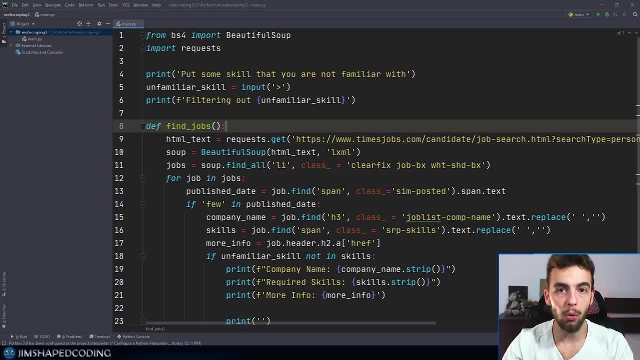 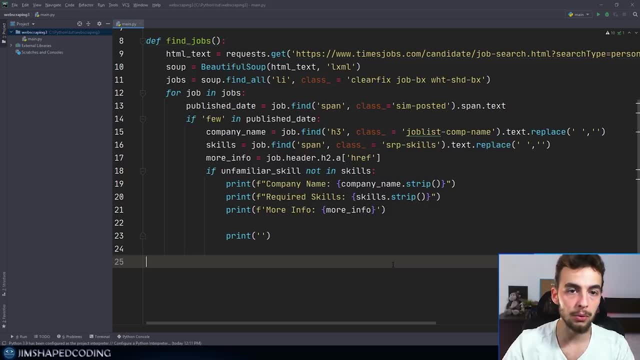 we have one function that executes our main program, And then what I'm going to do here is using the logic of if double underscore name is double underscore main. So that way, if you want to extend this program, only if this file is ran directly. 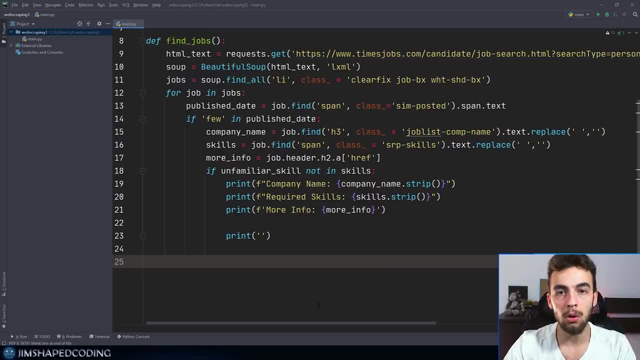 then this function will be executed. Now, if you don't know what I said about if double underscore name equals double underscore main, then I have a video that explains this condition, so you can check that out by the suggested link above. So let's write here: if double underscore name, 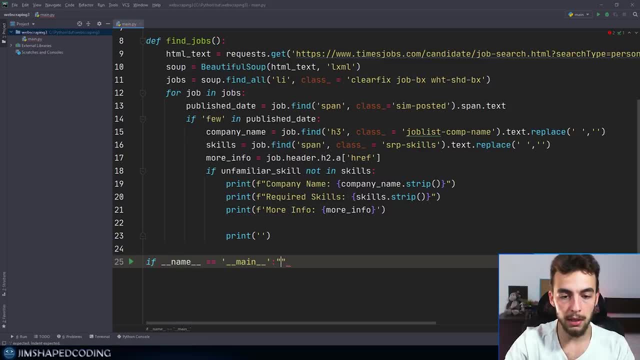 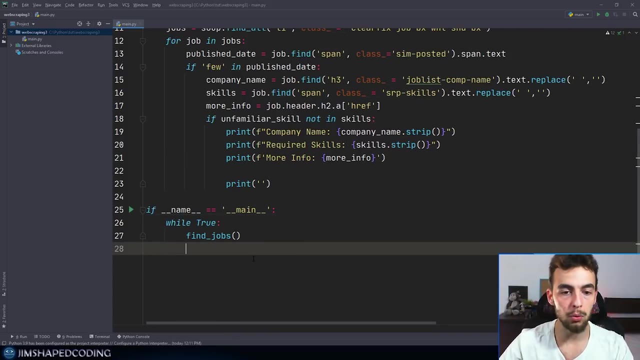 equals to double underscore, main inside a string and then right here while true. So I want to run this program forever And then I will call the find jobs And right after it, since I don't want this program to being executed like every millisecond. 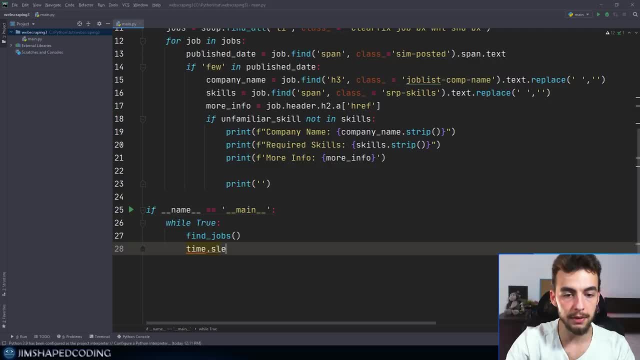 then I'm going to write here timesleep. So timesleep allows your program to wait certain amount of time that you decide, and you can provide its argument by seconds. So I'm going to write here 600 just to make that program to run every 10 minutes. 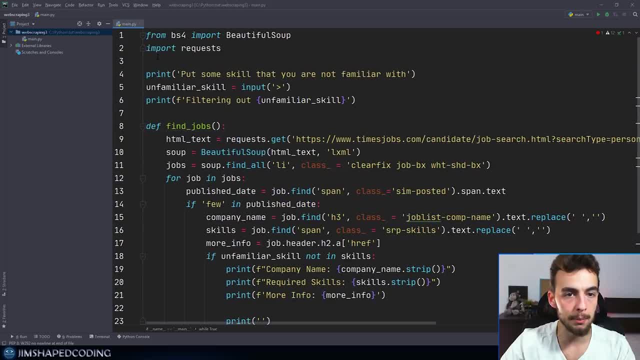 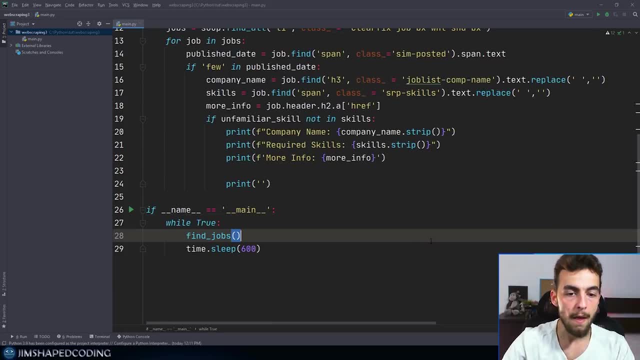 But you can notice how we did not import the time library, So let's do that by import time, okay, And then this program. this program should be okay. Now, to make this more dynamic, I actually prefer to make some variable here that will be equal to 10.. 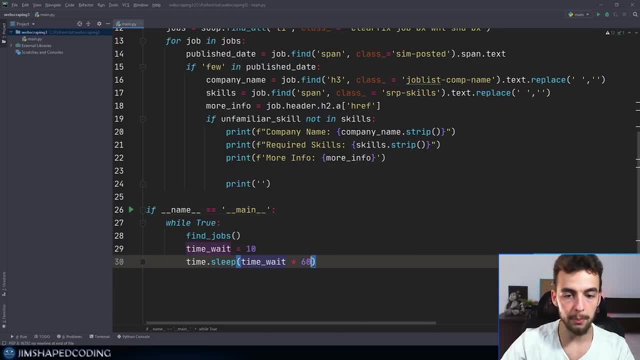 And then I will just make that to be equal to time weight multiplied by 60. And right after it we can provide some extra information. Excuse me, this should be over here And we can write here waiting. Let's make it formatted. 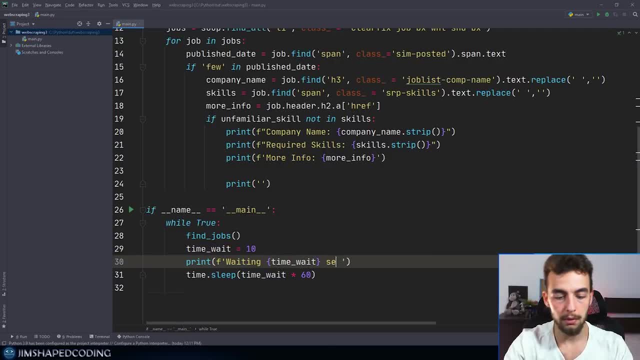 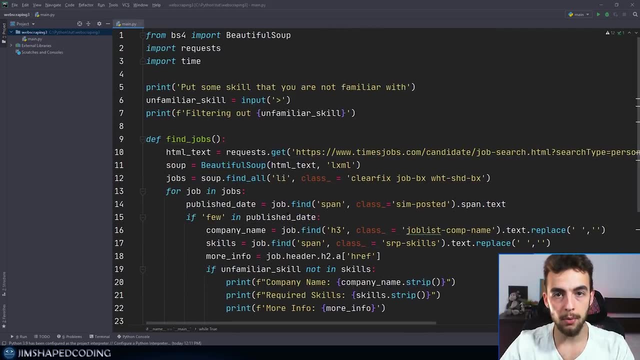 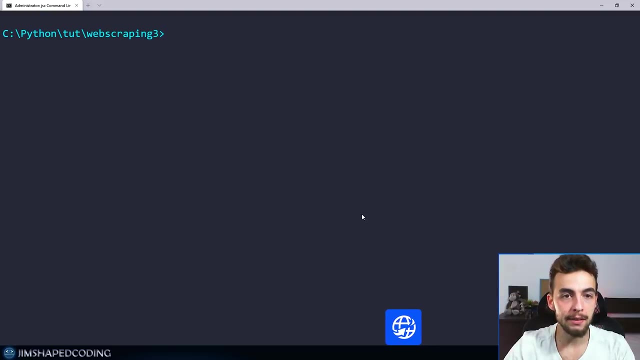 Then we can write here waiting time, wait seconds. And let's write three dots here. Great, so this is great. So if I'm executing this program, I expect to see this program running every 10 minutes. So I'm inside my command line interface. 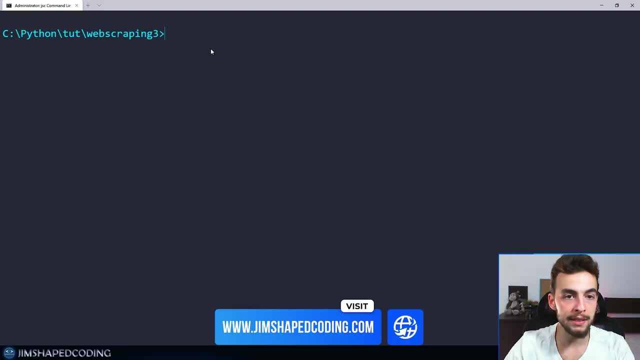 and you can see that my directory has been already set to the directory where we worked. So I can go with Python and then execute the name of the file by calling it, So it will be mainpy, And then, once I run that, you can see that we receive this output. 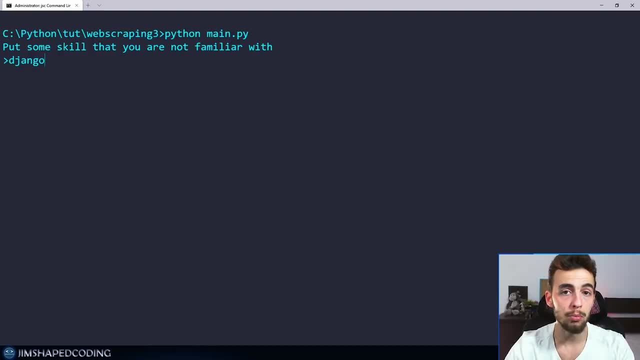 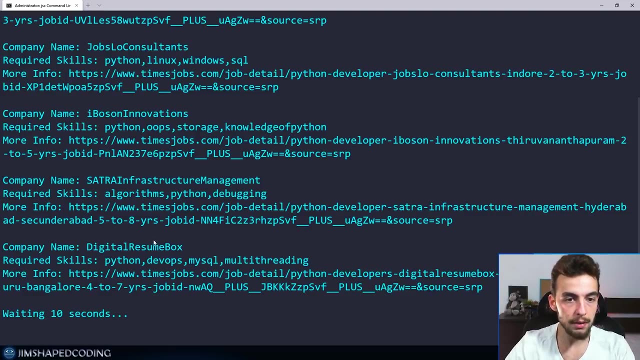 And then I have to provide some information that is going to be filtered out, And then let's write here Django again And you can see that we receive the results successfully. But, more important, we see that waiting 10 seconds, which is not great. 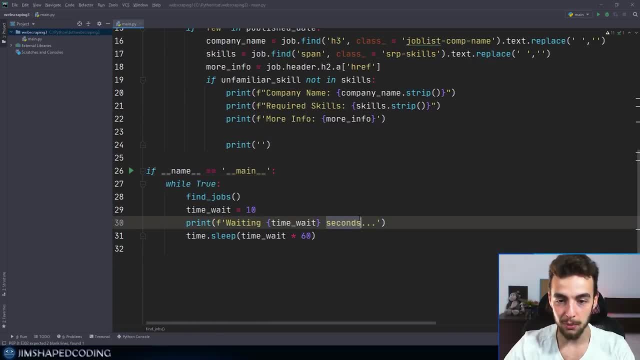 We have to change that to waiting 10 minutes because we are waiting 10 minutes. So we are waiting 10 minutes, But the program works great. It was just my mistake by writing here seconds, So it should be minutes for sure, But I'm not going to wait 10 minutes. 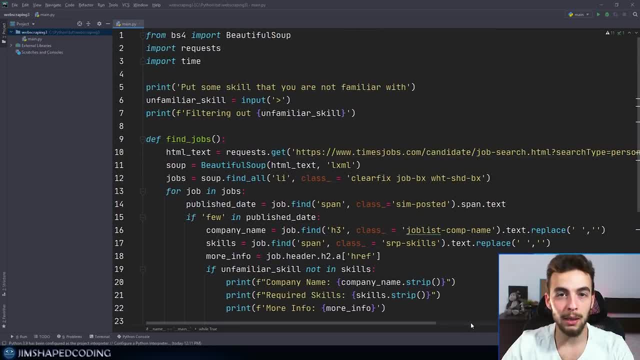 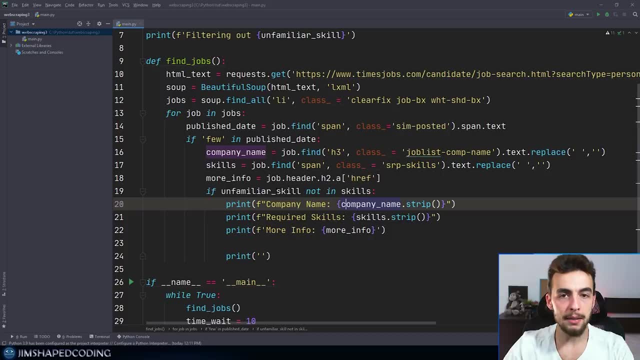 until this program is running one more time, And so I will allow myself to move on to writing this information inside file. So it makes sense to write this kind of information in a separated directory. So I will go inside my web scraping tree file. I mean folder. 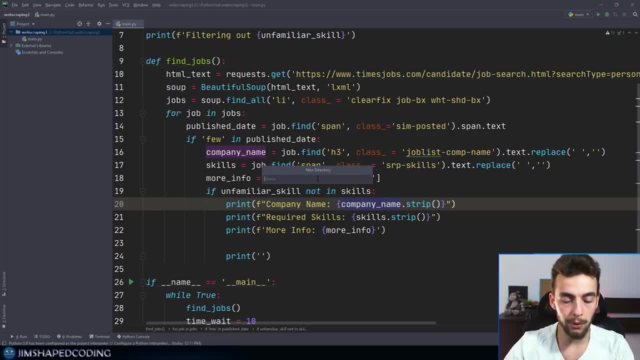 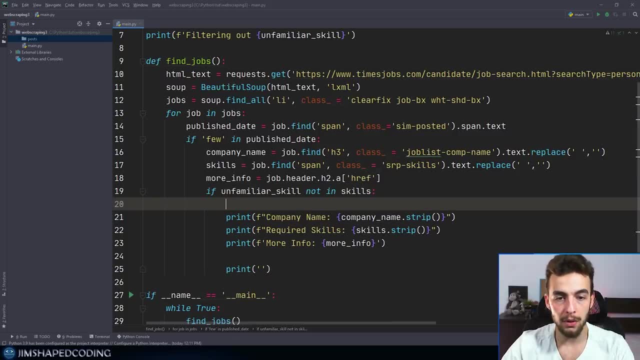 and then I'm going to create here new directory, which is going to be named as posts, And then I'm going to write here some extra functionality that will create files- I mean text files then- and then inside each text file I'm going to write this exact information: 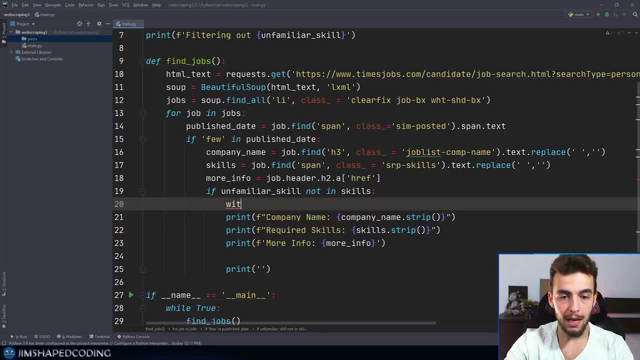 So you can do that by with open. I already show you how you can do that in the first episode. Now I know that I don't know how to do that. I don't have any separate tutorial about working with files in Python, But you want to consider? check out my channel. 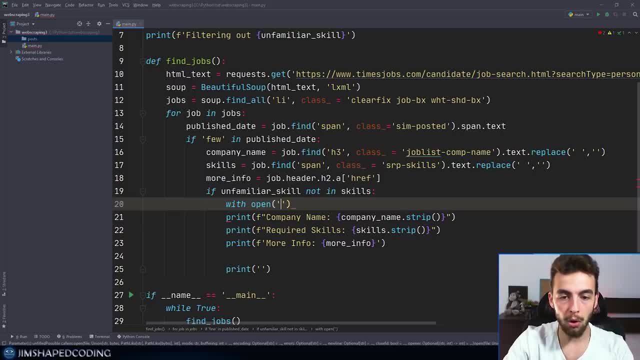 maybe I will upload very soon So you can go here, and that time I want to put here information and I will call my post directory And then inside here I have to provide my file name that I'm going to create Now before I move on here. 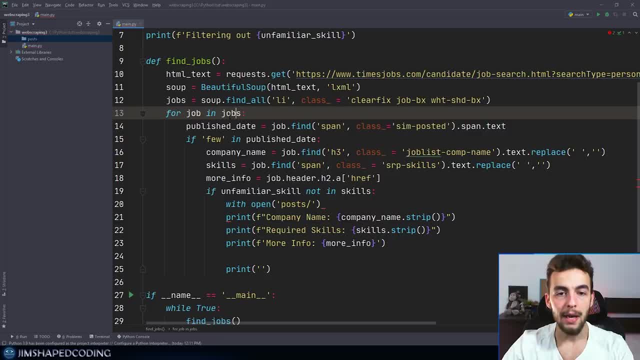 I thought about changing my for loop here And use the enumerate function. Now, enumerate function is going to allow us to iterate over the index of the jobs list and also the job content itself, And so I have to provide here one more variable like index. 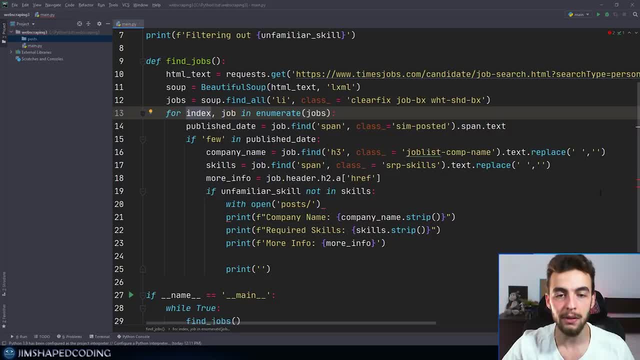 So the index is going to be a kind of counter for the job that I'm iterating on, And then the job variable will relate to the job Beautiful sub object itself, And so it makes sense to name our files with the index of the job that I'm iterating on. 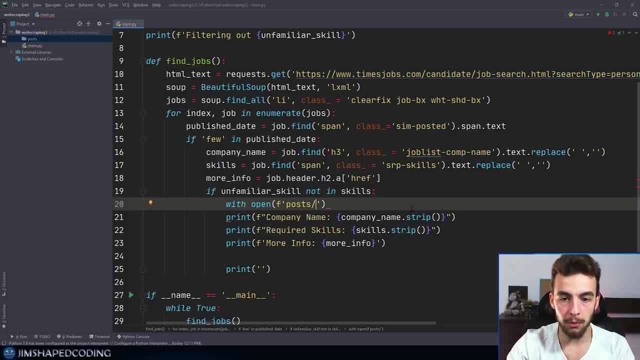 So I will change this into a formatted swing And then I will write here indextxt. So it will be something like the following: And I expect each my text file to be named like zerotxt or onetxt and so on. Now the second argument will be the permission level. 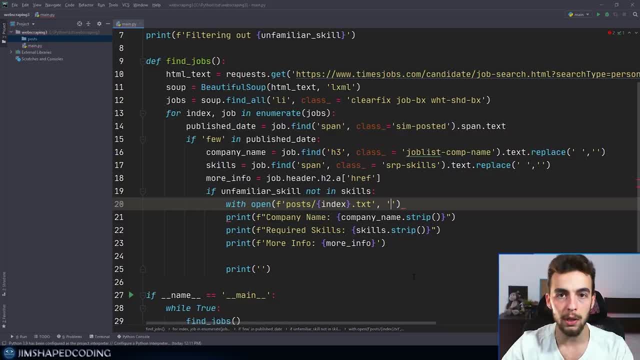 Now the second argument will be the permission level. Now the second argument will be the permission level that you want to give when you create or open a new file. And this time I'm going to write here W, and that stands for writing inside a file. 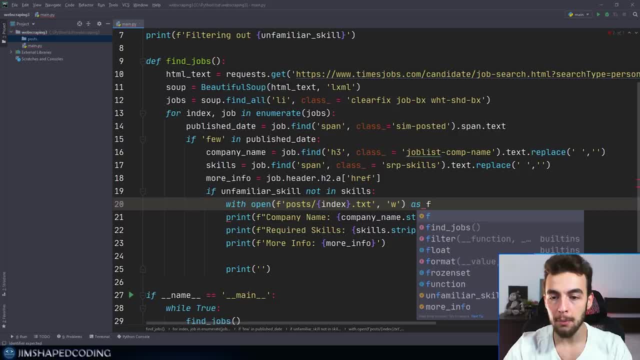 And then I have to use the as statement and I'm going to use the F variable. So inside that block I can write to a file with the F variable And I'm going to go inside my with open and I'm going to create intendation. 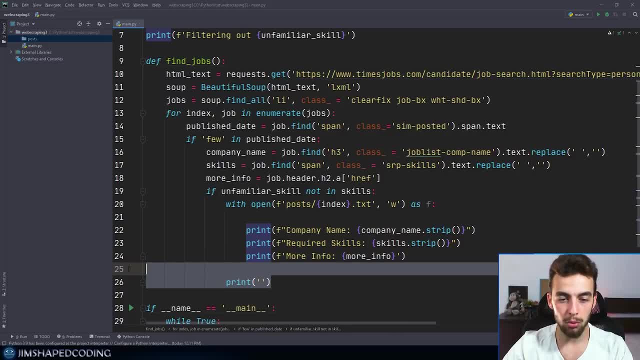 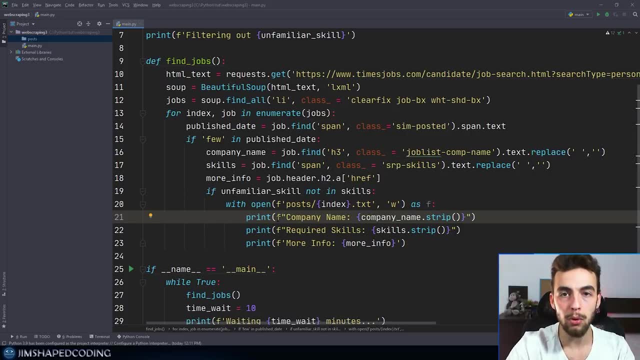 And I'm going to create intendation of the prints And I'm going to delete this print line here, And it makes sense to remove this blank space as well, And all I have to do here is changing this print statement to F dot write. 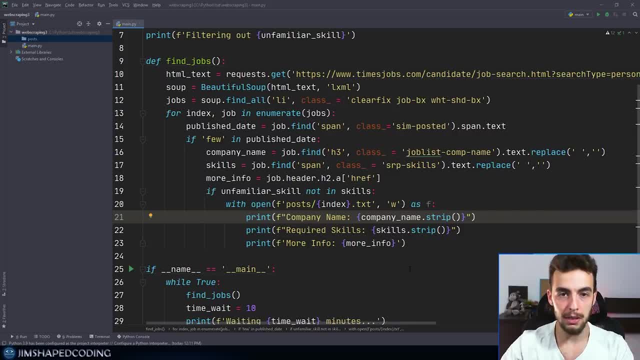 And then that time I'm not going to print the results in the command line interface. Besides, I'm going to write the information in a new file. So I'm going to use the combination. So I'm going to use the combination of old shift here. 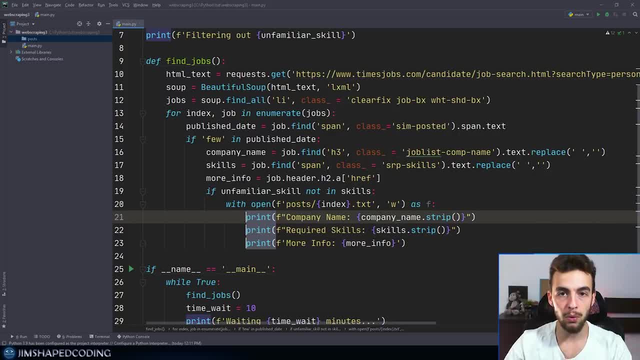 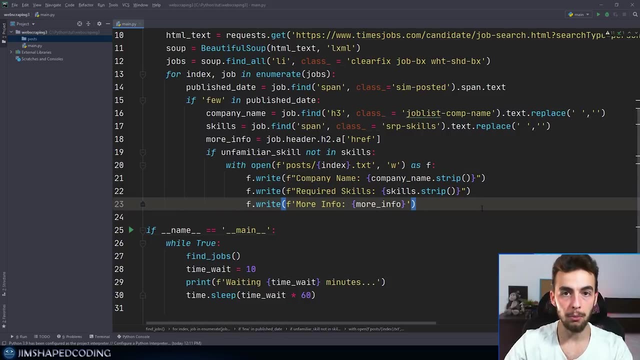 And I'm going to change those entire three prints to F dot write okay, And then I'm going to open the parentheses So it will be closed by those, And then I expect for each job to being written inside a file, And once I do that it might be a great idea. 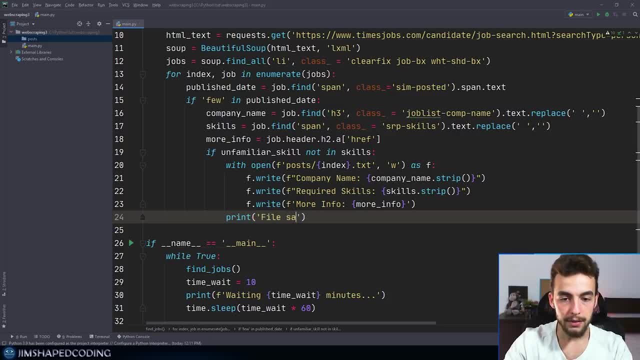 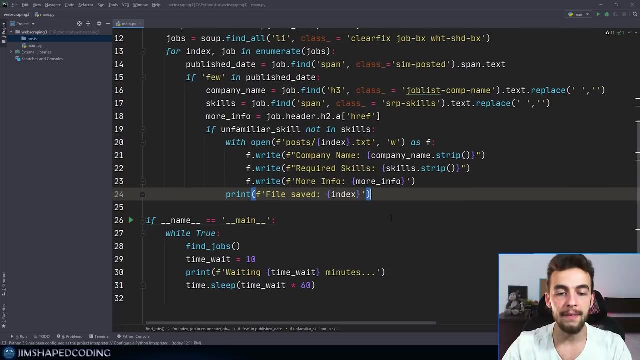 to print a sentence like file saved, And then you can provide the name of the file as an extra information. So I will create one more time formatted string And then I will relate to that index variable. And now our program is complete, So let's check it, okay. 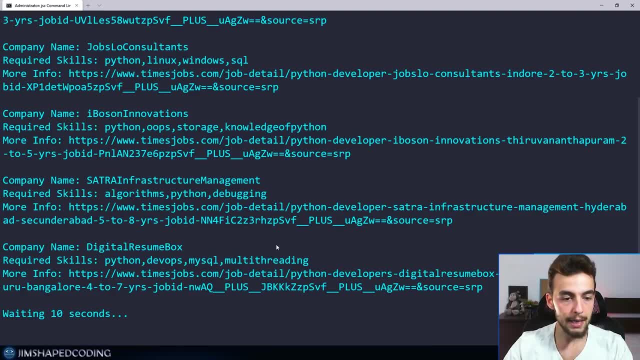 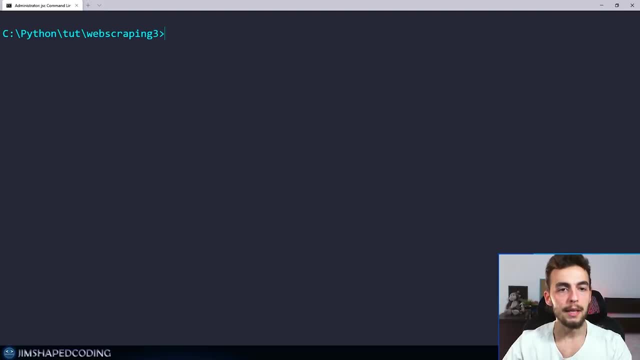 Let's go back to our command line interface And let's actually control break this program And let's write CLS to clear our terminal, And then I'm going to read this, And then I'm going to read this, And then I'm going to re execute my program. 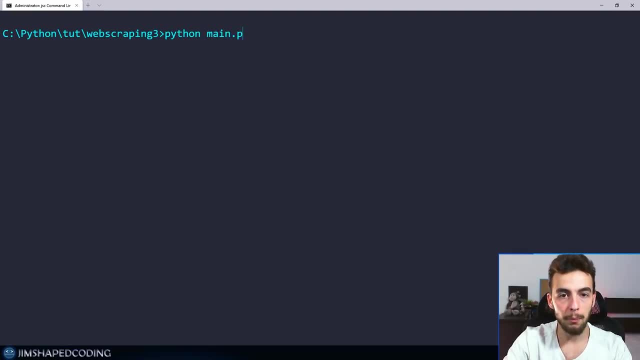 So it will be Python mainpy And then I'm going to execute it. So let's see, this time I'm going to write Django as well, And that time I don't expect to see output for the information. besides, I expect to see this: okay. 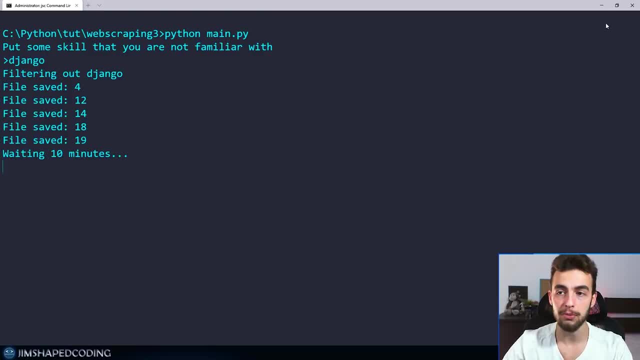 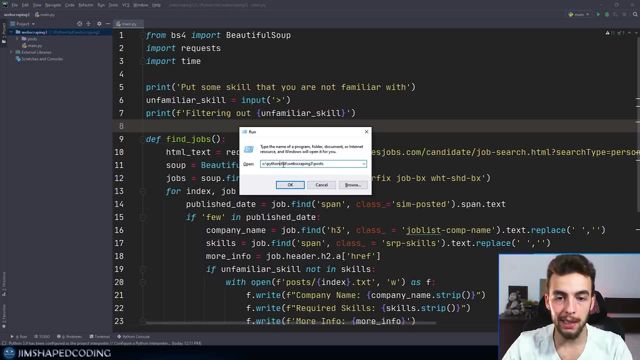 So let's see what is inside each of our files. So let's see what is inside that posts directory. So let's see what is inside that posts directory. So let's see what is inside that posts directory. Okay, so I'm going to go inside my cpython tut web scraping tree. 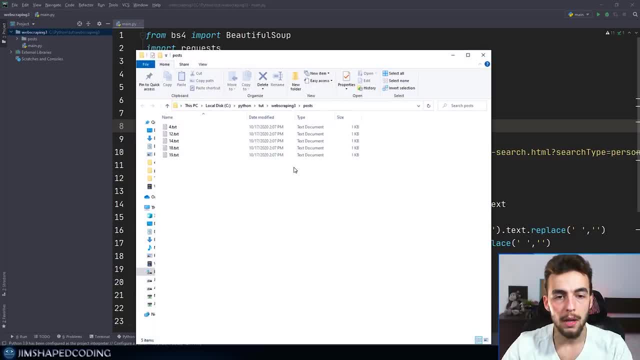 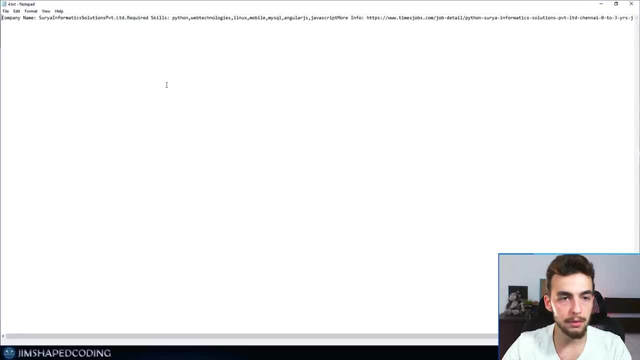 And then the posts directory that we created a few minutes ago, And you can see that inside of that we have our text files. But if I go here inside, let's see if the results are okay. Okay, so I'm not quite satisfied with that. 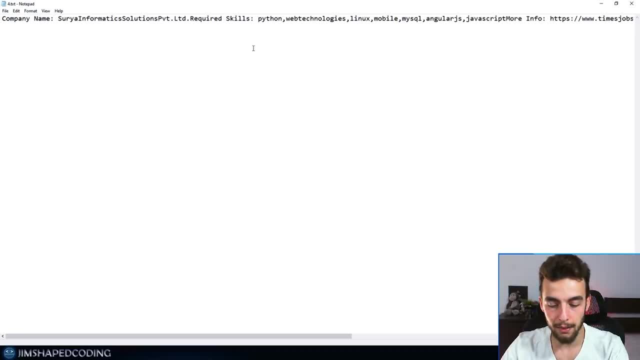 because it might be a greater idea to see that like, I mean like this: okay, So you might want to create your own post directory. Okay, so let's see if the results are okay. Okay, so you might want to create your own post directory. 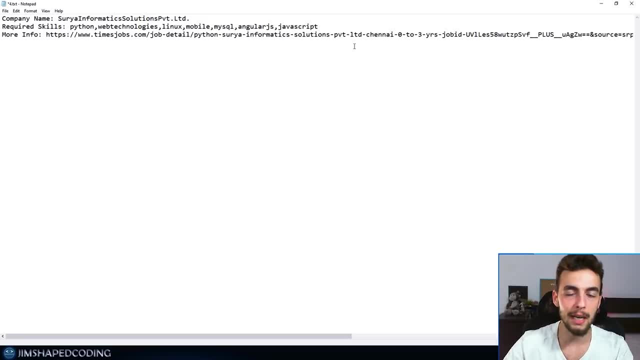 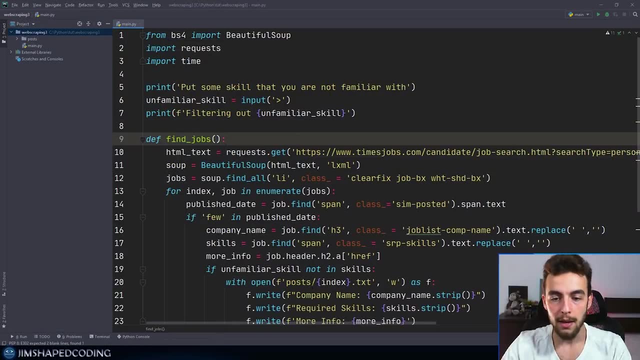 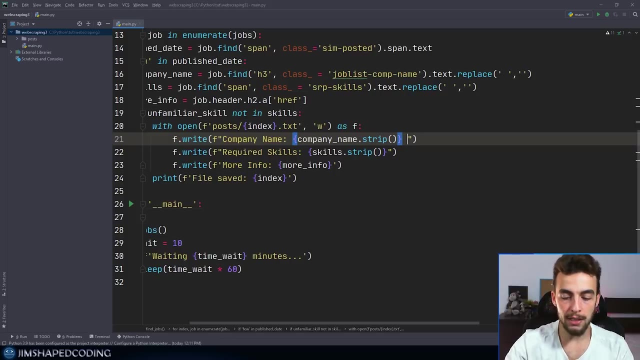 want to divide those information in separated lines, But that is not going to be complex. So we just have to go inside our Python again And then whenever we write to the file, we have to use that convention where you can just jump a line And that will be backslash n. So when you 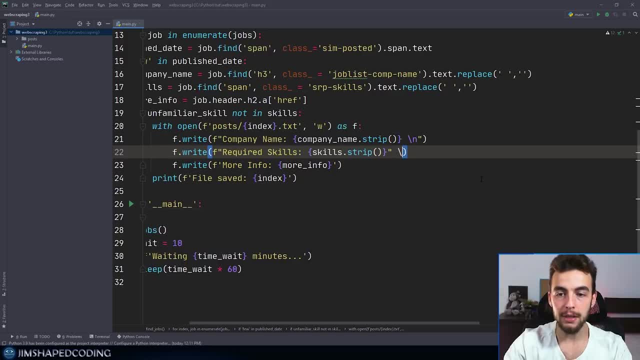 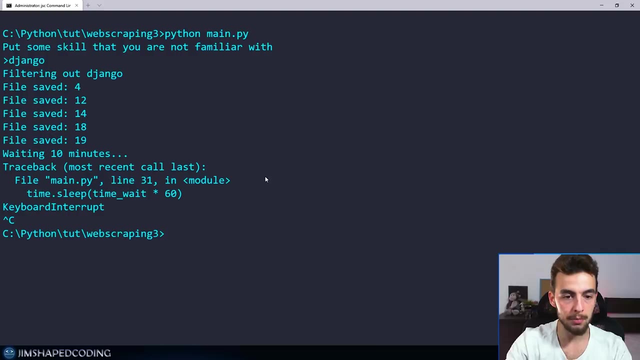 provide backslash n inside a string. it is just a convention that is going to jump to the next line right after it. So it will be backslash n for the first line and then also here, And let's run this program one more time. So I'm just going to break the program and re execute it, So that time I 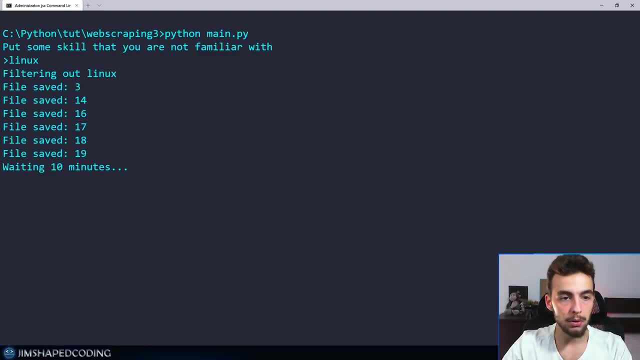 will write Linux, And then let's test our results one more time. So let's go inside our 19 dot txt And then let's test our results one more time. So let's go inside our 19 dot txt And then let's go. 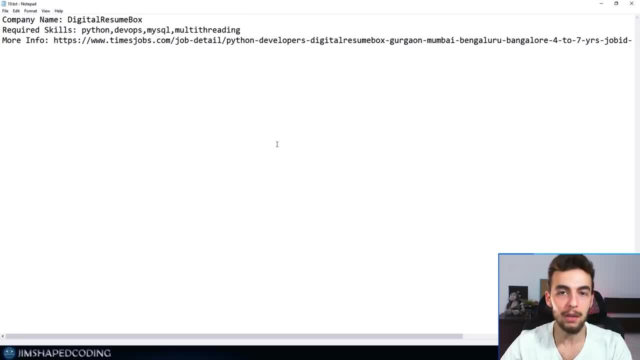 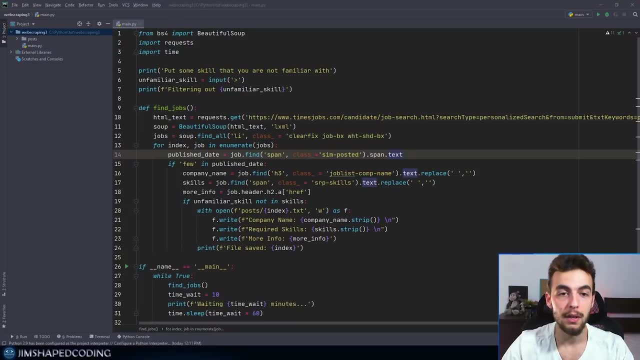 inside our 19 dot txt And then you can see that the information is right there, just like we expected. Okay, so this is quite great. Alright, guys. so I hope you enjoyed this entire series, And you can find everything that we have done here by the links in the description, Of course. 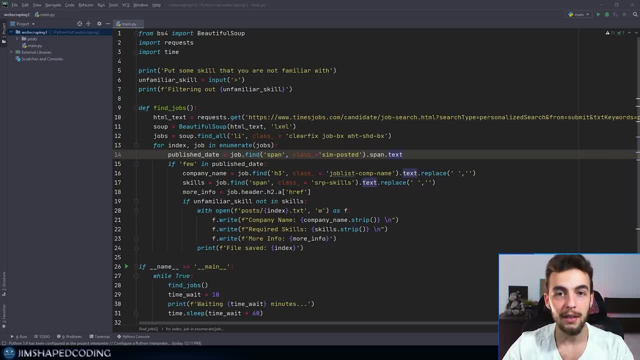 I will provide extra information in my website about this series. So if you like this video, consider subscribing and also hit the like button. I will see you in my future uploads.